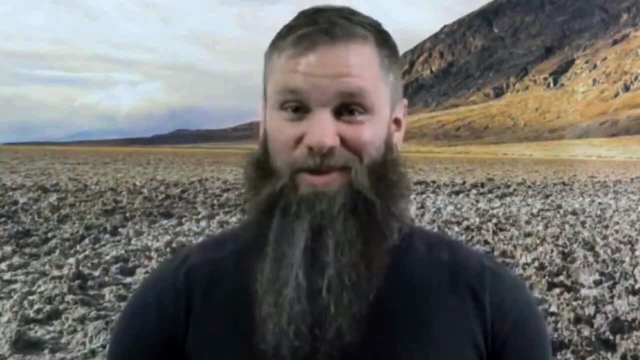 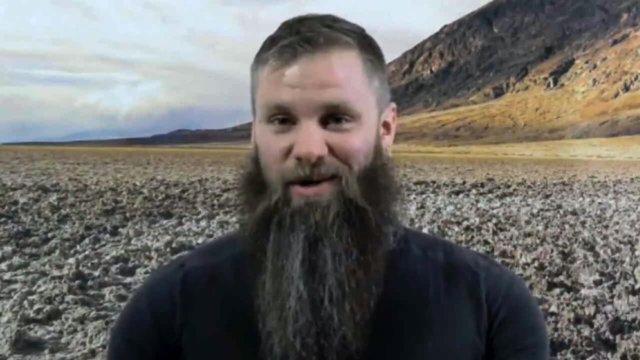 I have an awesome guest for the show today, so I'm kind of giddy, super excited. But before we get to our guest, we have to do our background quiz. As those of you who are consistent audience members know, every month we have a photo behind our back. 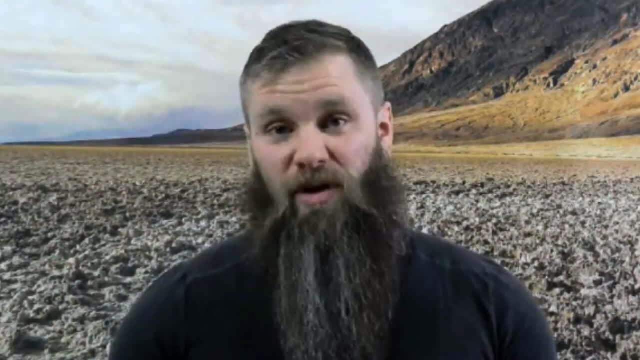 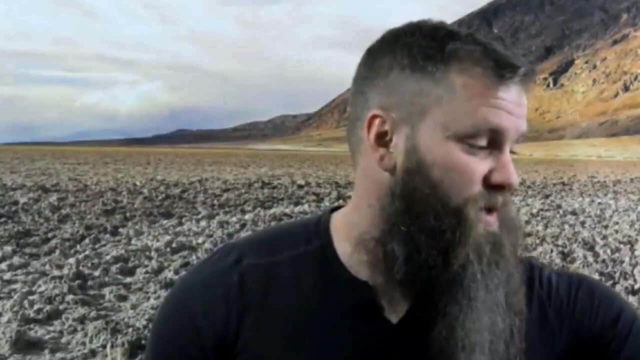 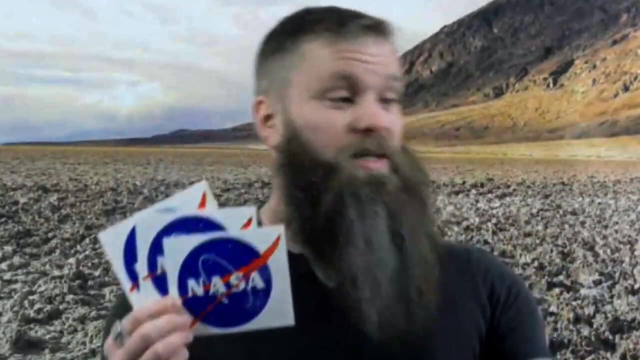 Our host And we give you a chance then on Twitter before the next episode, to give us a guess at what that is and maybe win some prizes. So, for instance, our third place winners: they win some of these really cool NASA stickers, And our second place winners win NASA stickers plus the Astrobiology Graphic Histories. 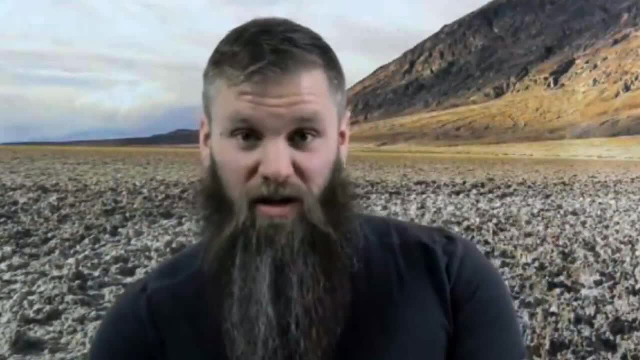 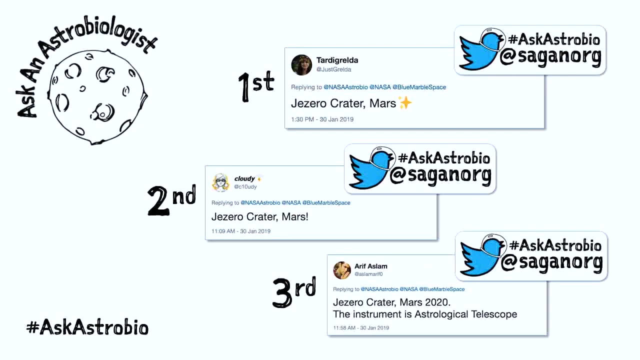 And then our first place winners. they win both of those, as well as a glass, a drinking glass from Saganet. This month's winners from all the right responses We had on Twitter yesterday are: in third place Arif Aslam, in second place Cloudy and in first place Tardy Grotto, which is an incredible name. 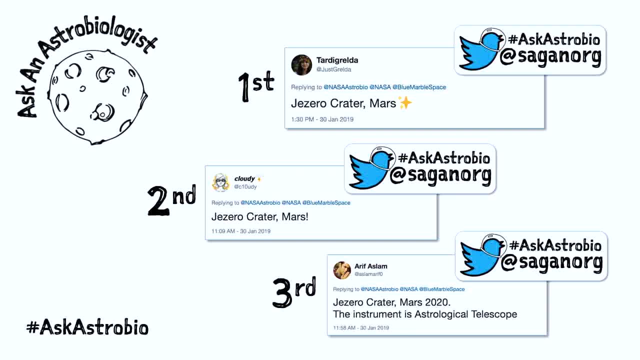 I do have to say, Arif, our third place winner, you got the right location. It is Jezero Crater on Mars, the next landing site for Mars 2020, for our next big rover. However, there is no instrument called the Astrological Telescope. 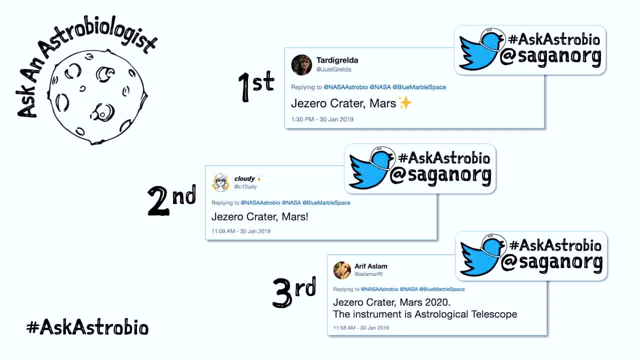 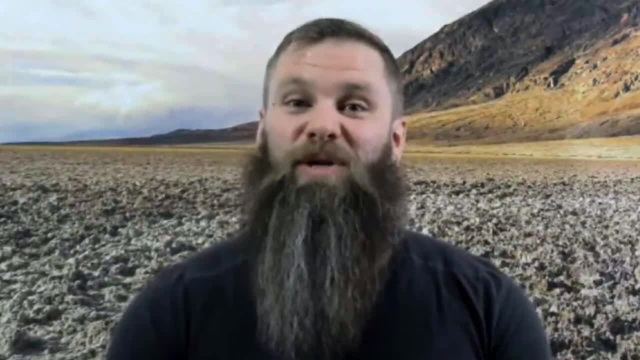 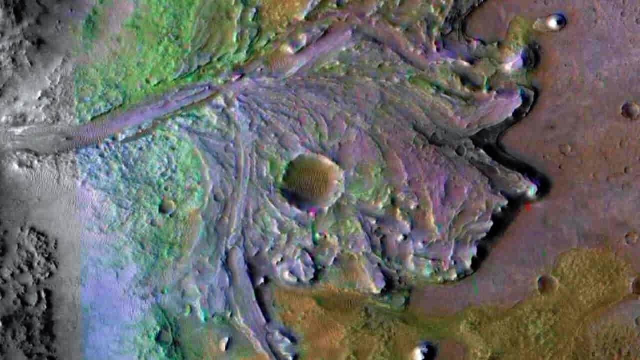 We do astronomy and the instrument was CRISM and the context camera On board of the Mars Reconnaissance Orbiter showing that beautiful area around the next place. we're landing a really big rover on Mars. So thank you very much for that- for competing in our background quiz for this month. 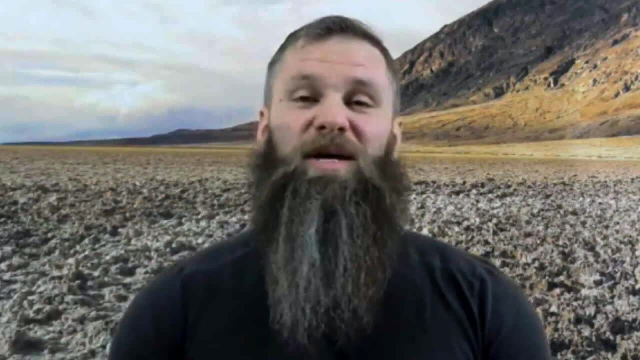 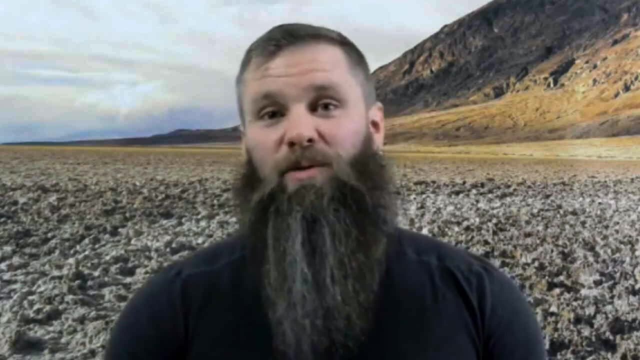 The picture behind me will be the background quiz for next month, So if you have an idea of what it is now, that's great, But just wait until we announce the day before our next episode, when we have the background quiz, And you can then answer and try to win some of these awesome prizes from NASA Astrobiology. 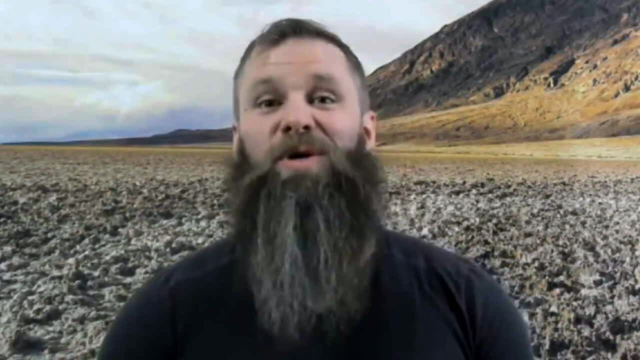 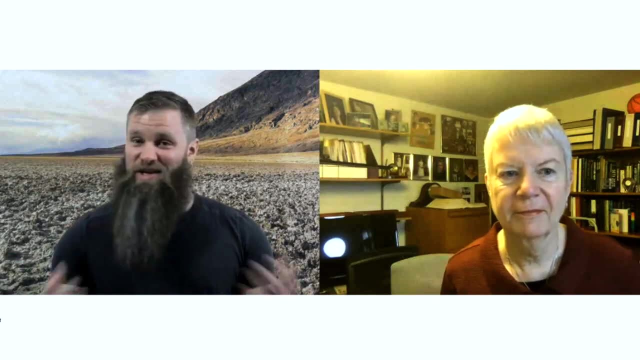 And from Sagan. So, without too much further ado, I'd love to get into today's conversation with our guest. Today we're speaking with Dr Jill Tarter. Many of you know her for all of her years in doing research with the SETI Institute- the Search for Extraterrestrial Intelligence. 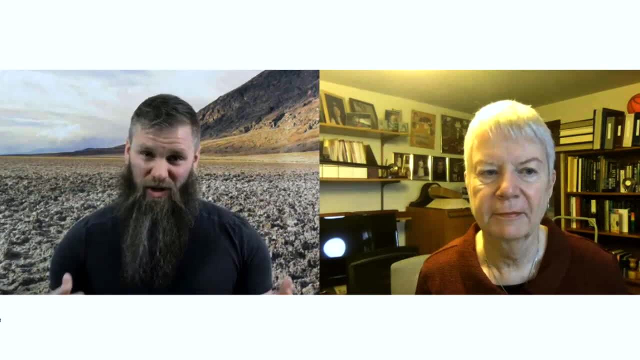 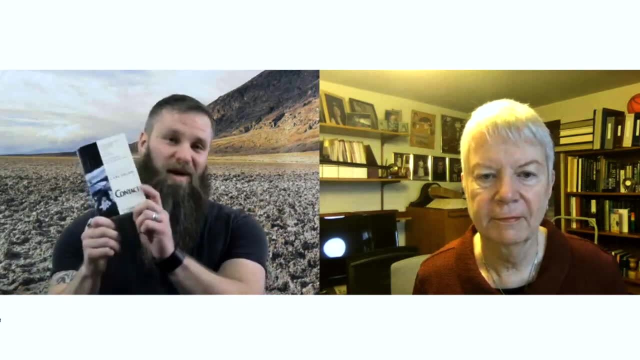 She's been a huge proponent of speaking about the importance of asking that big question of are we alone? And many of you also know that she was the basis for the character of Ellie Arroway in Carl Sagan's novel Contact, Which was made into a film back in the 90s starring Jodie Foster. 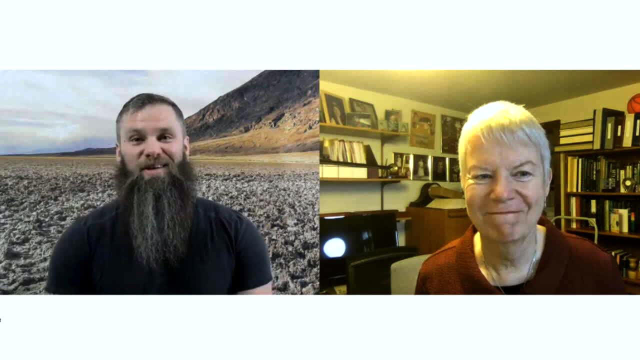 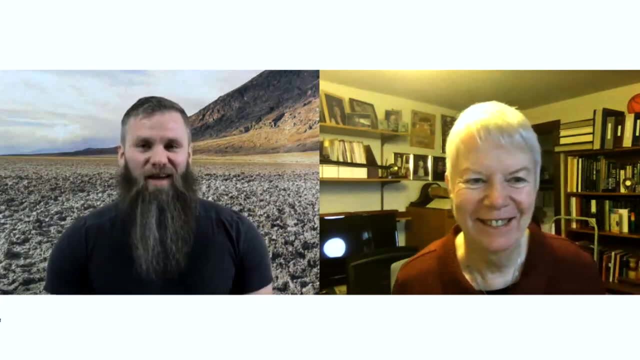 So, Jill Tarter, thank you so much for being an Ask, an Astrobiologist, Thanks for having me. Hopefully we won't have any technical difficulties. Yeah, I know, Sometimes the connections can be a little weird when we're doing a show like this where we're connecting in from different places in the country and sometimes across the planet. 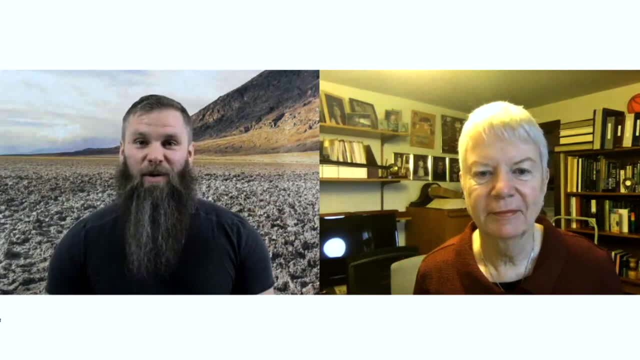 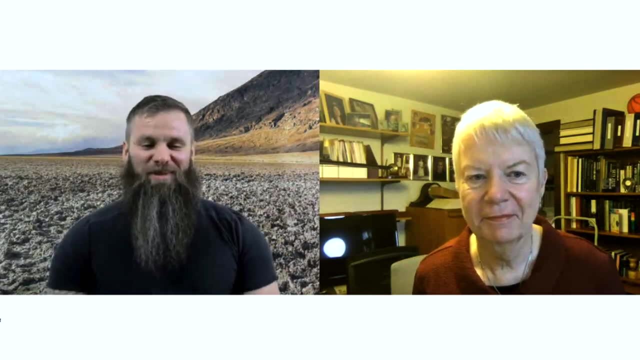 As much as we love technology, it's done great things for us, allowing us to put our ear to the heavens and see if there's neighbors out there. Sometimes we still have some issues, But that's okay, Let's just start chatting. It'd be kind of cool. 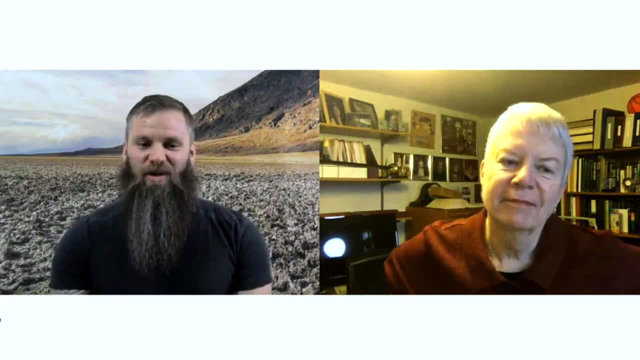 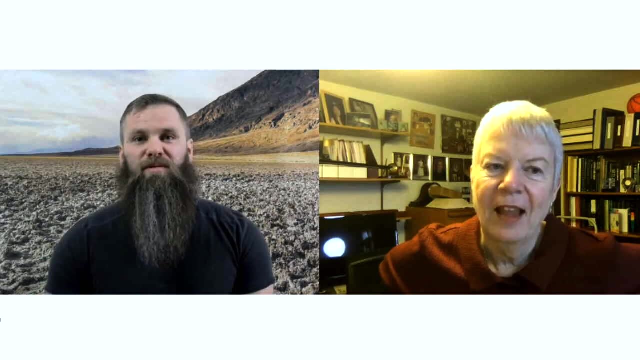 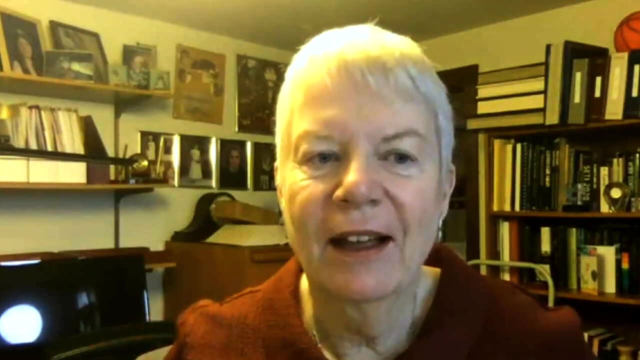 The first big question I'd love to start off with is: what got you interested in science and that big question of are we alone? Well, it was a really very fortunate accident for me When I was a graduate student. my first year I was supported to learn how to program the first desktop computer we ever had. 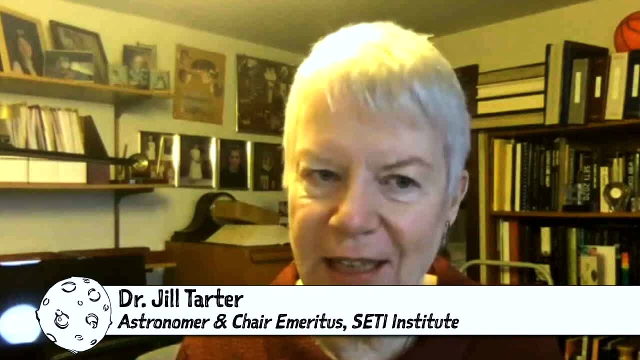 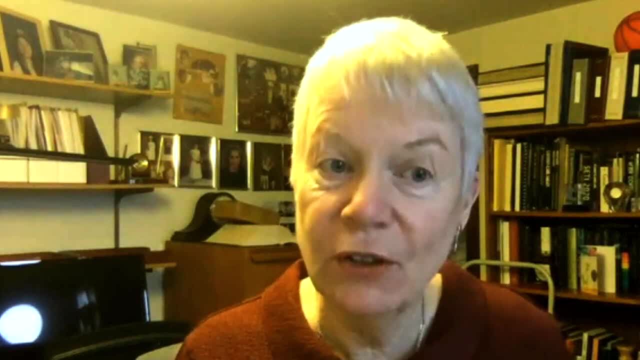 Now this was the PDP-8. Slash S. I always thought the S was for stupid And it took two of us to put it up on the desk Right. But you could use it And there was no language, So you had to program in an octal. 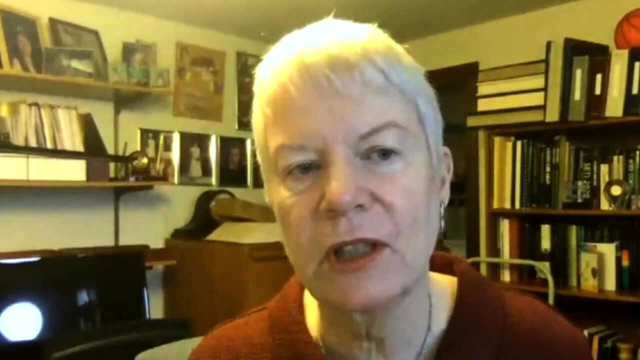 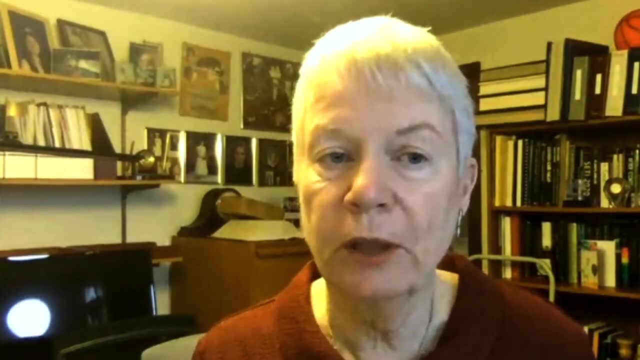 You had to set all the ones and zeros for the 11 instructions that this machine could do. And years later I was still a graduate student and this piece of equipment was surplus And it was given to Stu Boyer, an X-ray astronomer who had a brilliant idea. 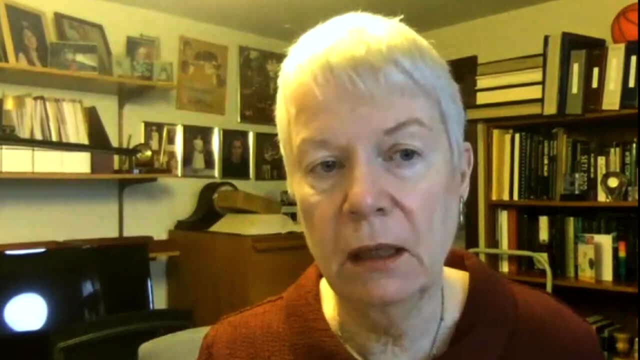 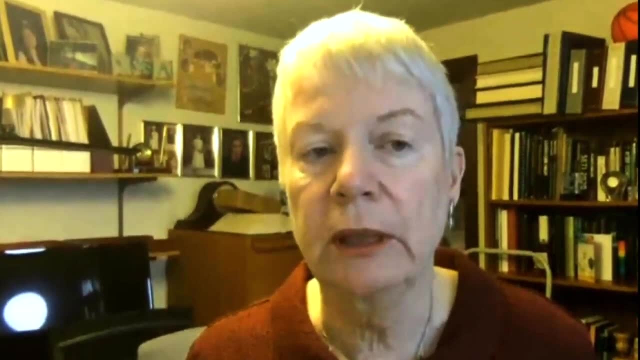 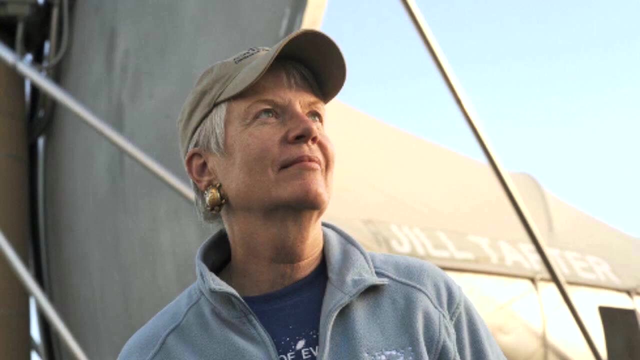 about how we could do SETI. while the radio astronomers were using the Hat Creek telescope that was run by UC Berkeley to do their studies, We could just make a copy of the signals being collected by the telescope and analyze them for engineered signals. He hadn't any money. 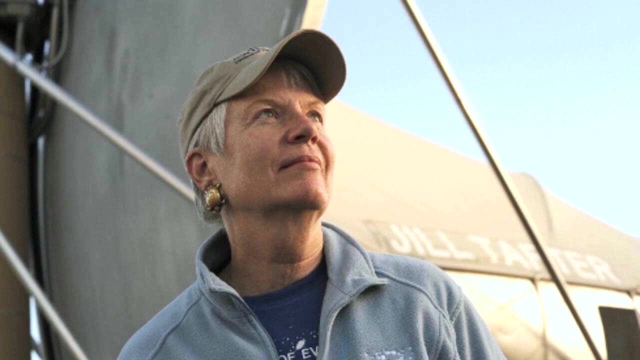 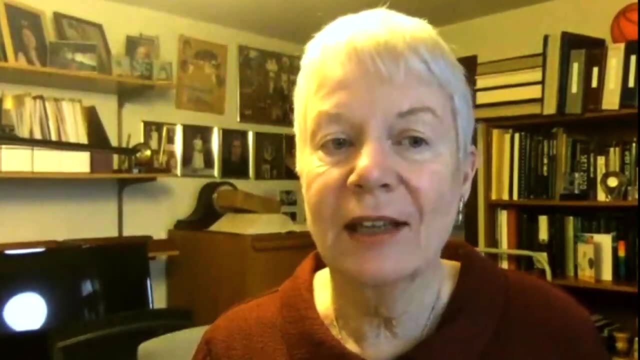 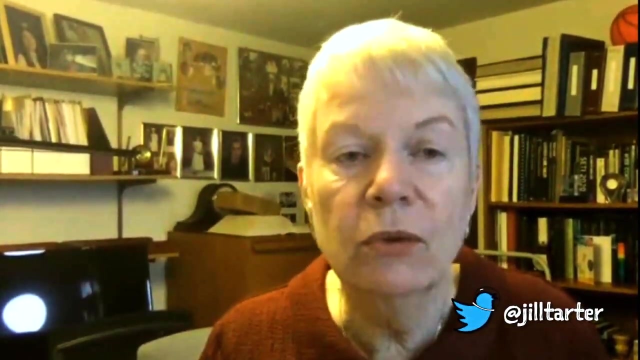 He was looking for ways to do it. Somebody gave him this old computer. He came to me And I thought: Oh my gosh. After millennia of asking priests and philosophers what we should believe about the question, are we alone, Suddenly they're tools. 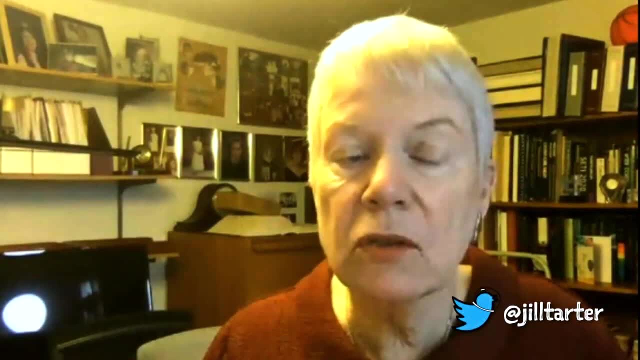 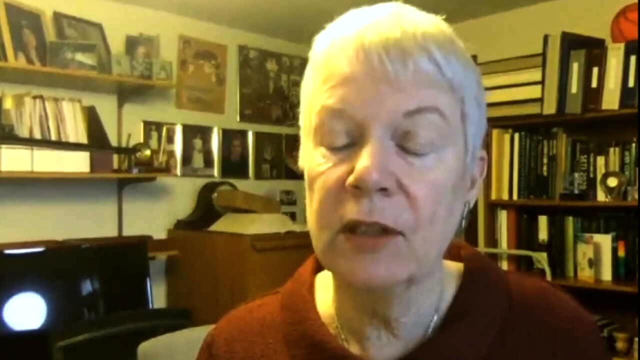 There's radio telescopes, There's computers, And so scientists and astronomers can get involved to try and find out what's out there, rather than accept somebody's beliefs. And so I said I'm in, And that's how it started, And I got hooked. 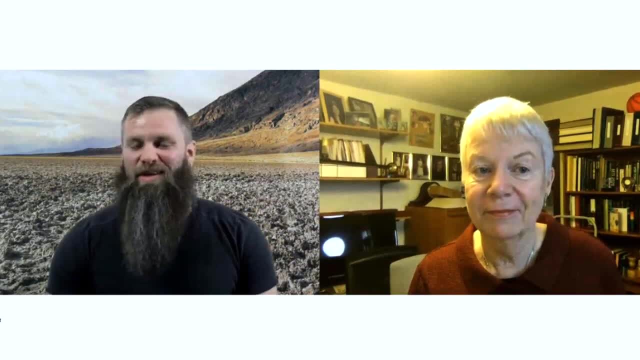 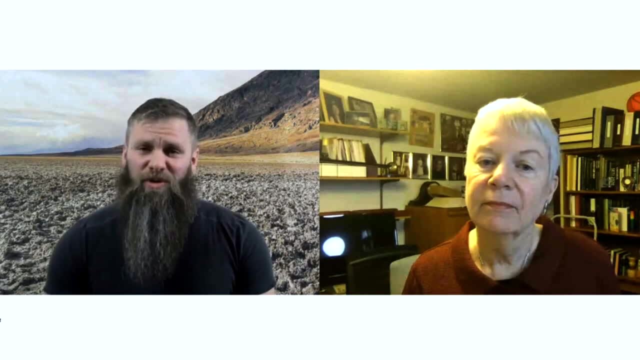 And I've never gotten unhooked. That's awesome. Yeah, I think a lot of us. we have those ideas when we're young. We look at the stars at night in the heavens and we wonder if we're alone, And it is really cool that we have these tools now. 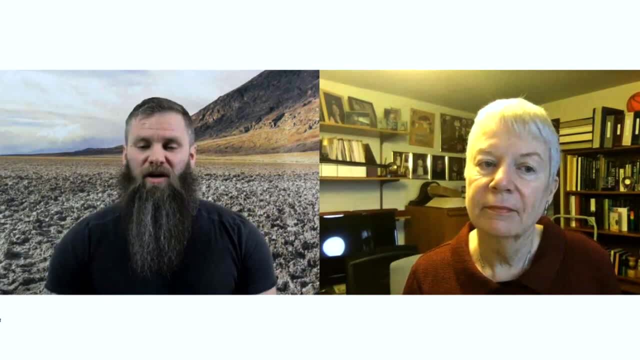 I think a big question a lot of people have is how SETI itself has changed over these last several decades. How much better have those tools gotten And what big things have happened in SETI during your career. Well, in terms of ideas, 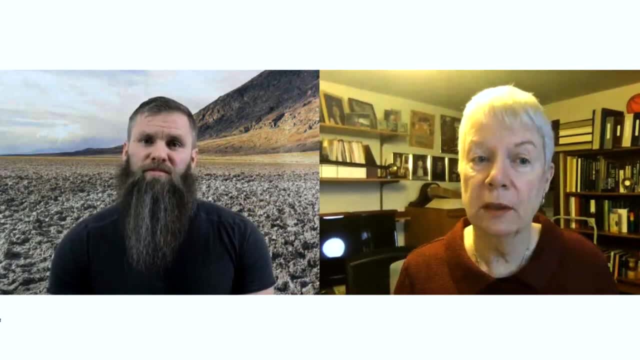 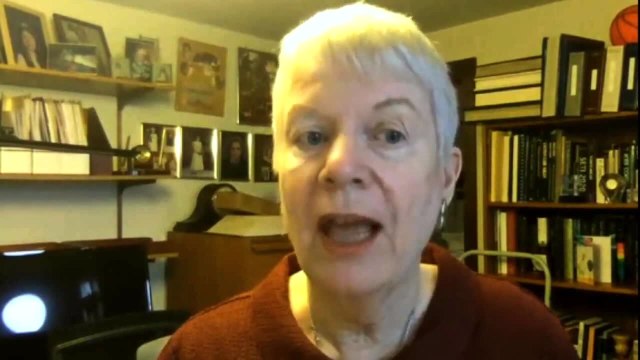 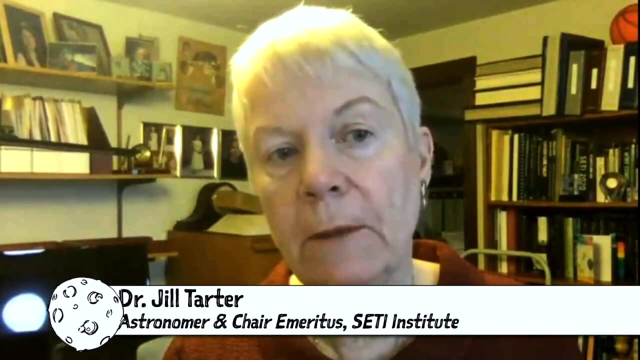 two enormous game changers over my career: One exoplanets, Two extremophiles, And then, in terms of instrumentation, we started out purely as a radio source, a search. We've added more computing. that's gotten better. We've built our own telescope so we can look all the time. 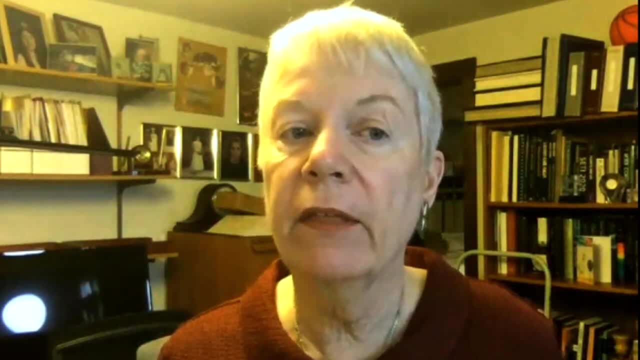 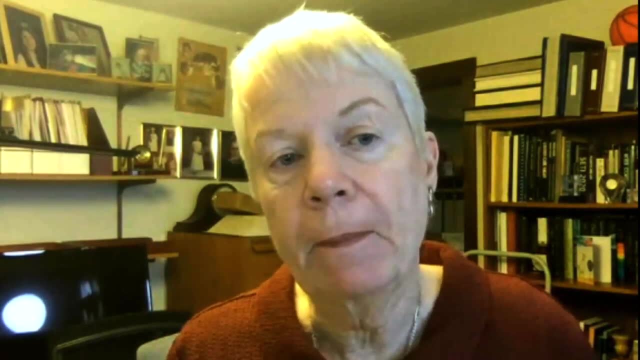 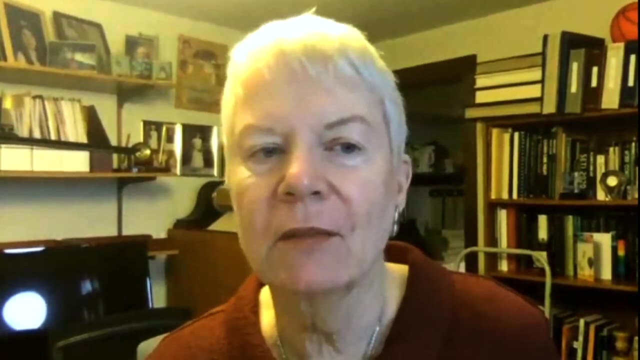 And then, when the technologies became available, we started to look at other things. We started to look at other things, We started doing an optical search, And so our current instrumentation threshold, I would say now, is to be able to get some sensitivity to transient signals. 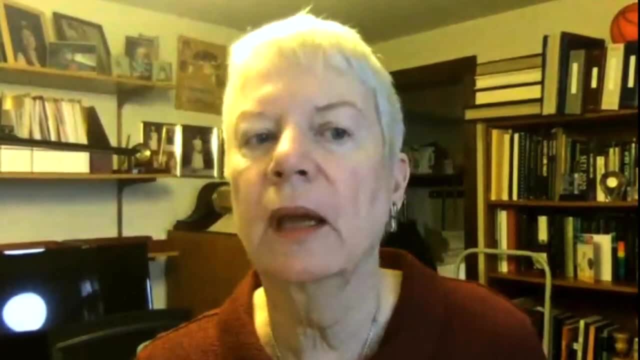 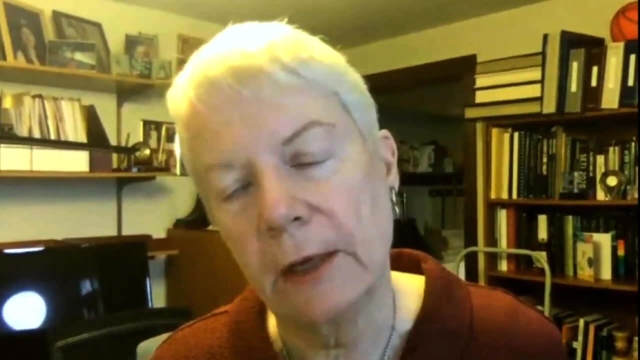 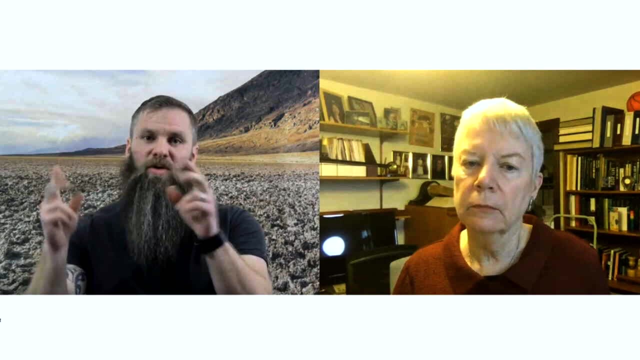 So we'd love to look at all the sky all the time, at all wavelengths. That's the next instrumental challenge whose door we're trying to beat down. Okay, that's interesting. So right now we're kind of limited to some window of radio. 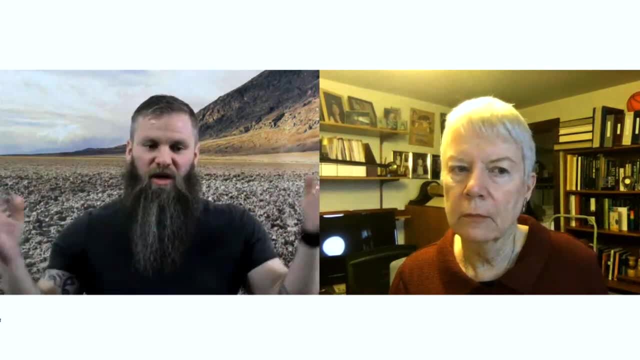 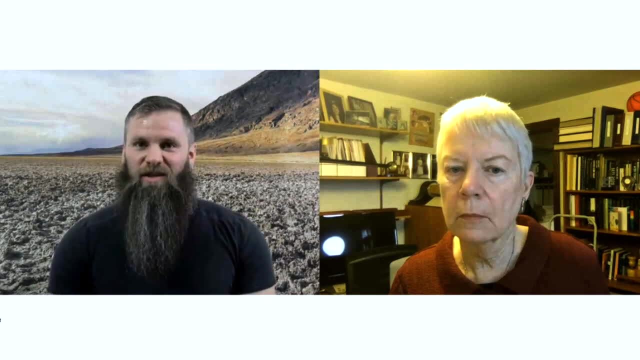 a window in optical but not really looking through the entire EM spectrum yet. But you did mention that we now have this telescope that allows us to be looking all the time. I imagine you mean the Allen Telescope Array for our audience members to know. 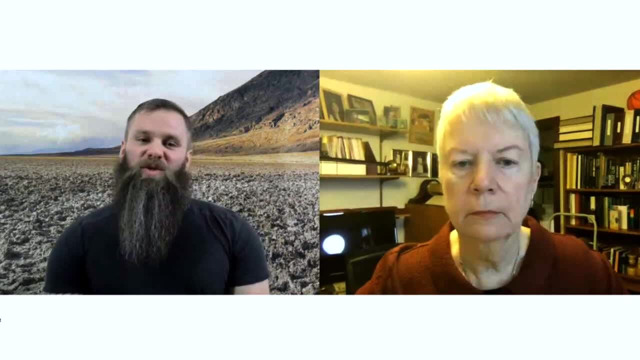 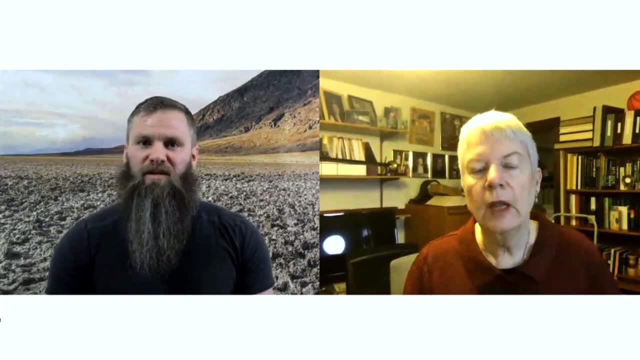 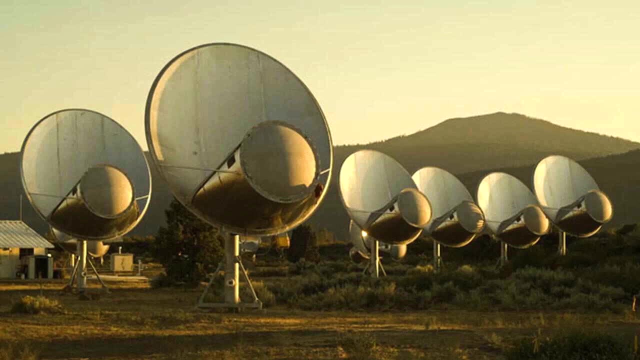 I do What we're speaking of there. Yeah, so now the Allen Telescope Array is, to my knowledge, the very first SETI-dedicated telescope array. Is that correct? That's right. It's the first time that we've built a telescope on purpose. 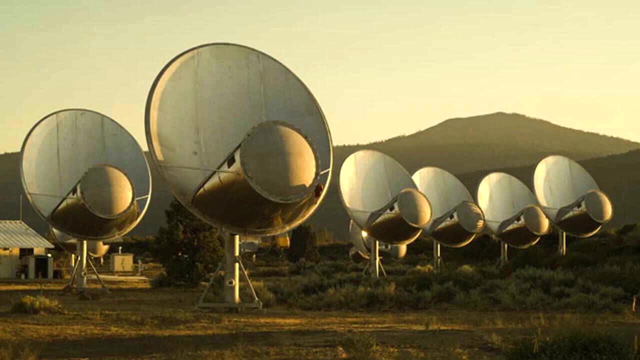 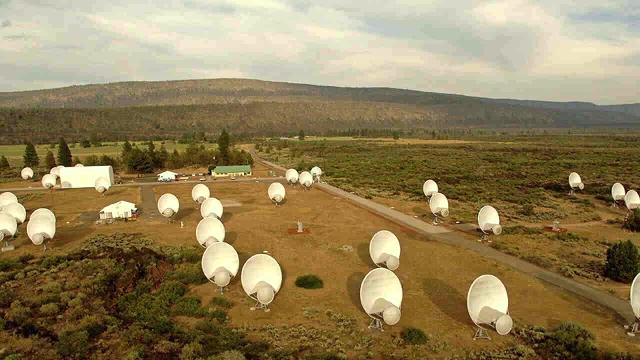 as well as doing radio astronomy, And it's the first time we've built a radio telescope as a large number of small dishes all hooked together with an enormous amount of computing, And that looks like the way in the future to continue to build ever-bigger radio telescopes. The Square Kilometer Array in South Africa and Western Australia will be built that way. The next generation, a very large array will be built with smaller dishes and more of them. So this is a good idea and we've proven that it can be done. 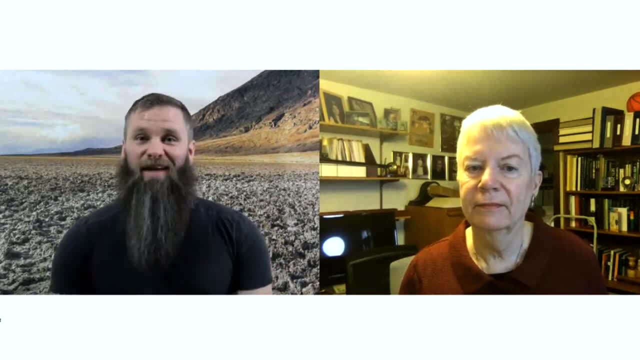 That's incredible. That's awesome. I'm so glad we finally have some dedicated instruments just for SETI, even though we have had other SETI searches on things like the Arecibo radio telescope And also the FAST telescope now being developed in China. 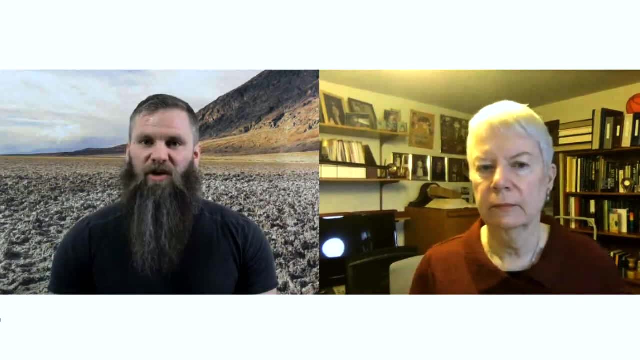 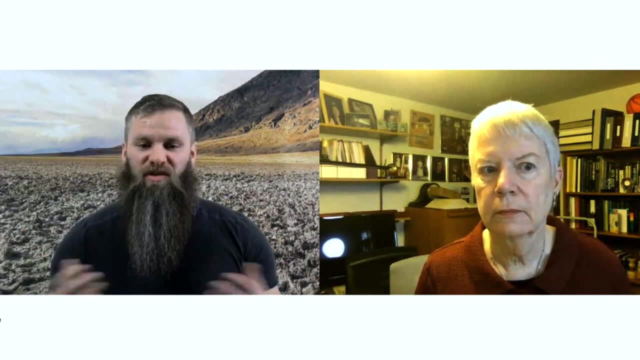 to my knowledge, has a mission objective of the search for extraterrestrial intelligence. If I can, how do you feel about now other nations also getting interested in SETI and kind of forming their own SETI searches? Okay, Bring it on. 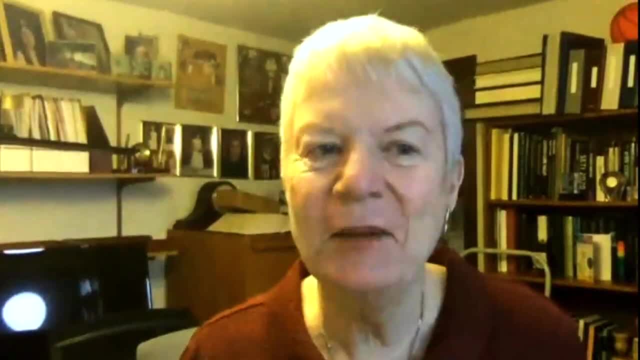 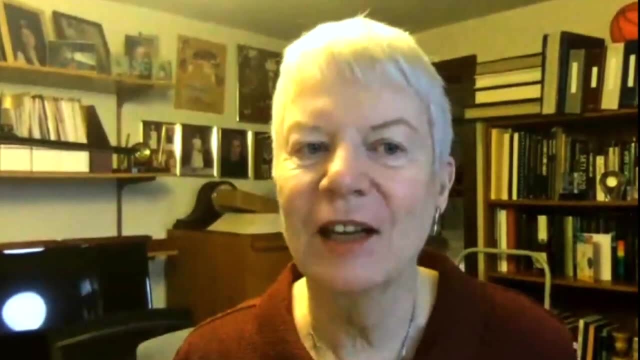 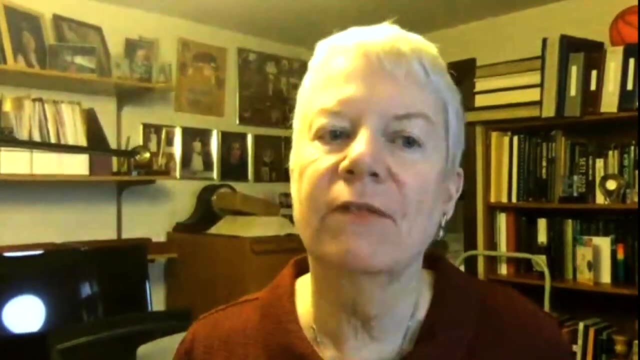 Absolutely. There's a message out there. It's coming to the planet, right, It's not coming to California or to China or to South Africa, It's coming to the planet, and that information is the property of all humankind. I think that's actually one of the very best things about SETI. 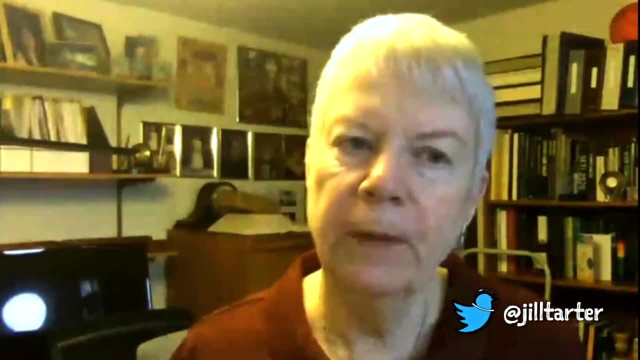 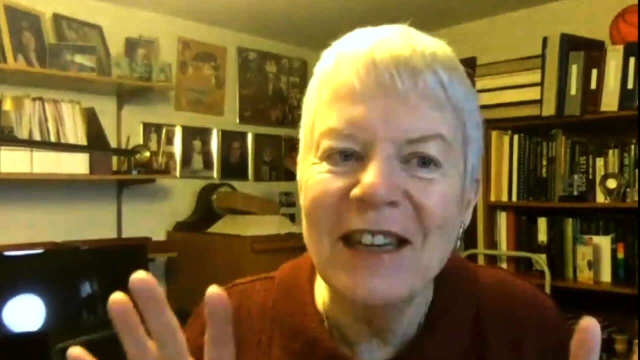 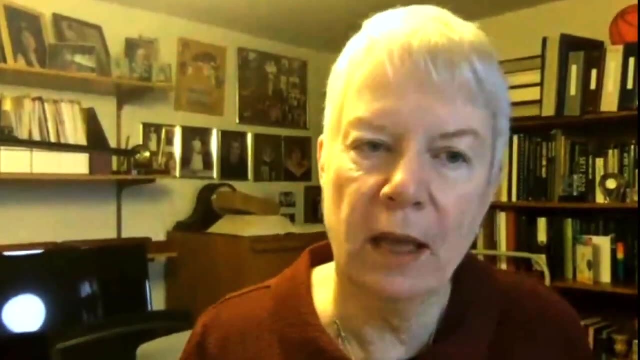 As we talk to people about what we're doing and try and get them interested in participating and supporting the work, we're actually expanding their perspective. We're making them, we're giving them the opportunity to see themselves in a different way to see themselves. 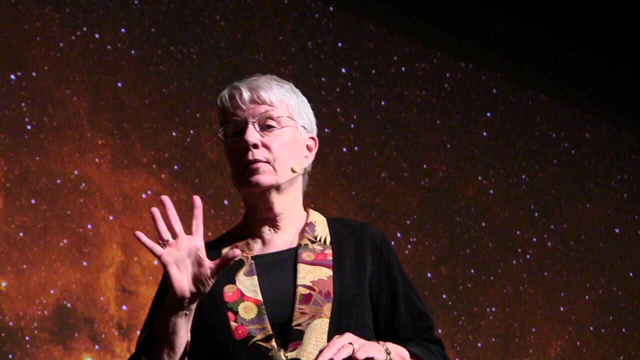 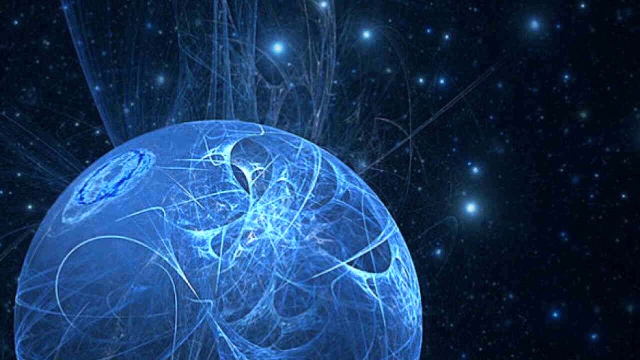 as one species- humans on one planet- And SETI kind of holds up a mirror to all of us on this planet and says: See, See, All you guys, You're all the same when compared to something else out there, And so it naturally reinforces. 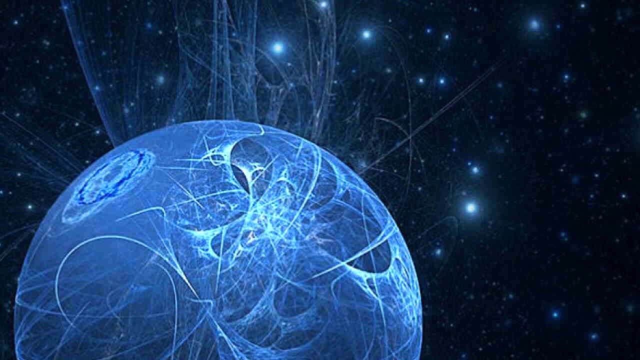 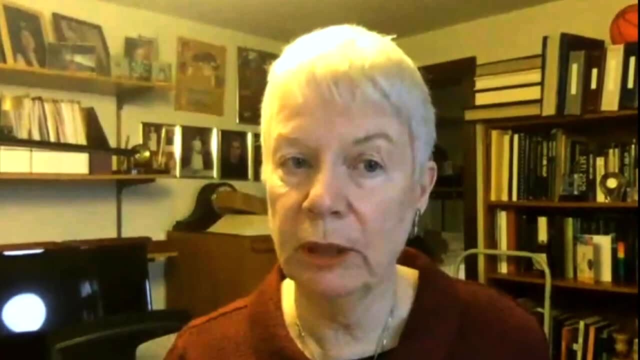 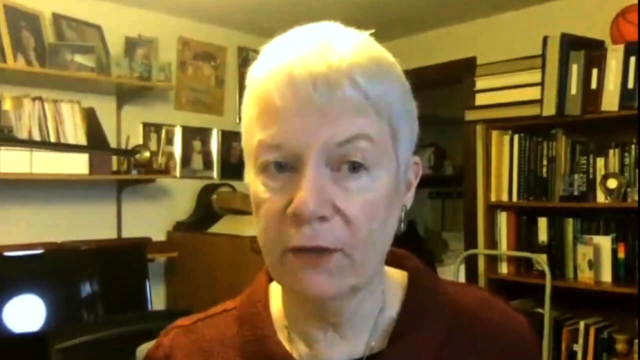 this cosmic perspective And I think that's such a very important thing for our long-term survival. We've got lots of challenges on this planet and those challenges are going to respect national boundaries. We are going to have to solve them globally, systemically. 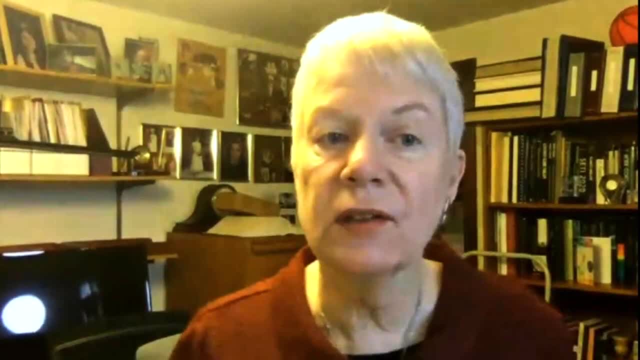 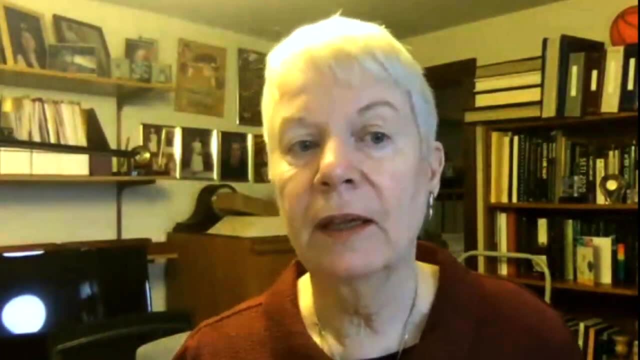 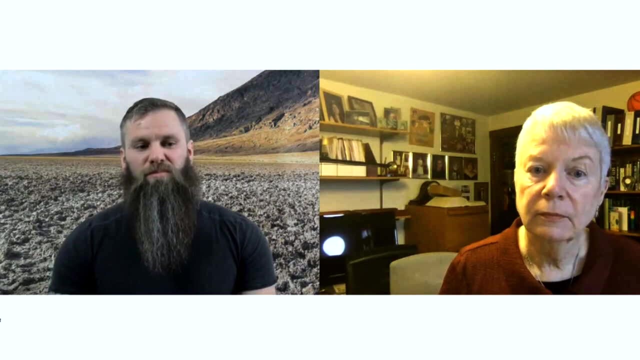 And if we get into the mindset of seeing ourselves as earthlings because of working with SETI, then maybe that's the first step in getting together to work effectively to overcome these challenges. That's interesting, yeah, having more of a global view through our cosmic perspective. 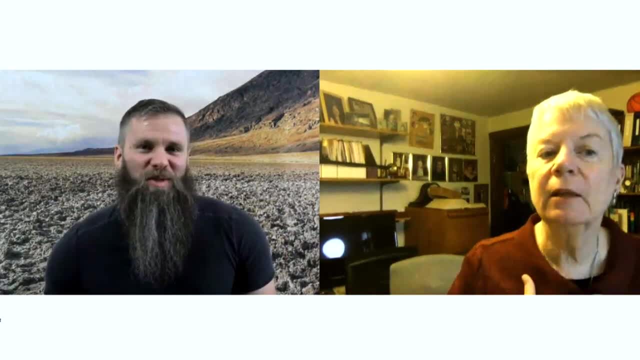 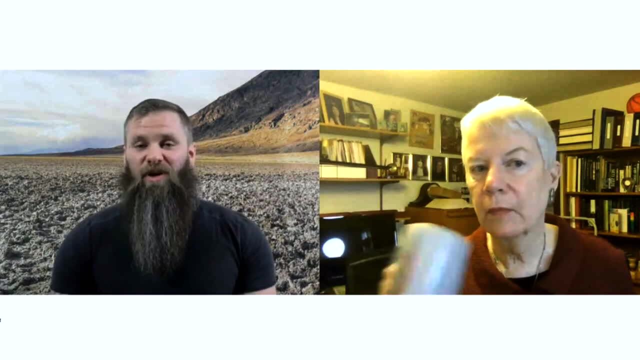 I love that I do have to ask so, since you brought up extremophiles and exoplanets earlier, you know this is Ask an Astrobiologist and most of our guests on the show previously have done more work in the realm of geochemistry. 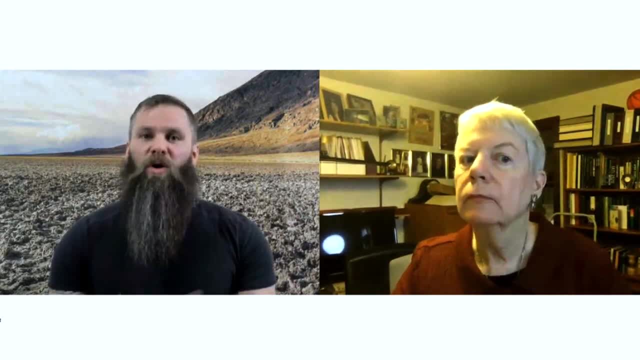 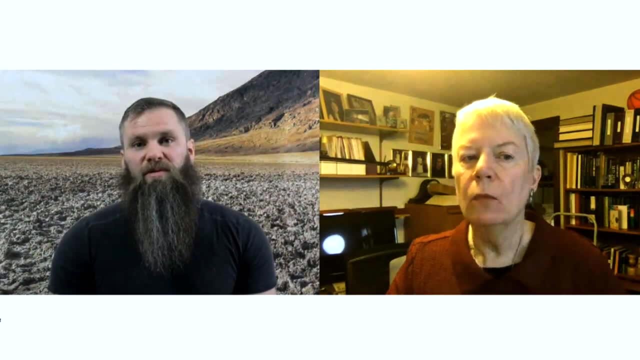 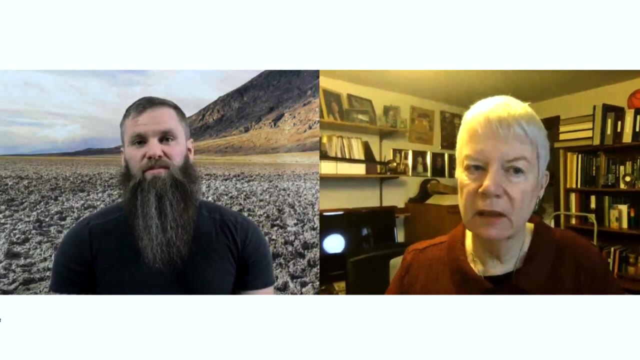 and planetary science. I'm wondering if you can speak for our audience, maybe about how SETI itself really fits inside of astrobiology. Well, most people think about astrobiology as looking for in situ biomarkers or remotely for biosignatures. 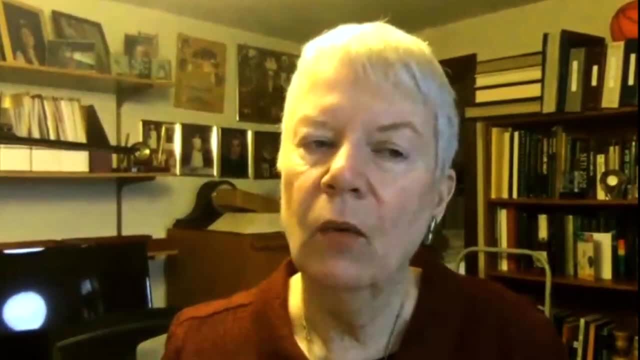 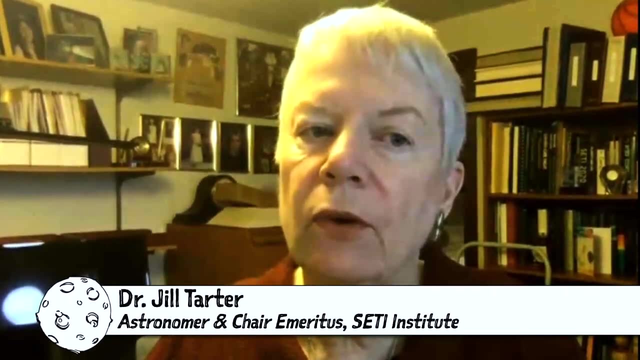 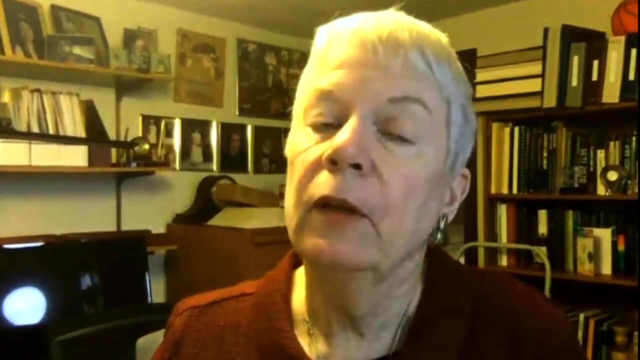 Well, think about it in a parallel way, that what we're trying to do is look remotely for technosignatures, looking for evidence of civilizations that modify their environments appropriately In ways that we might sense over the vast distances to the stars. Sure, we started out. 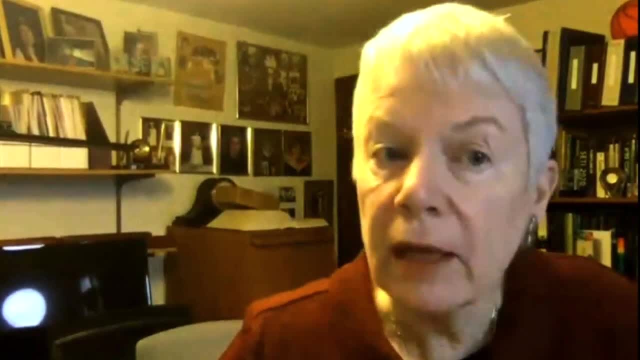 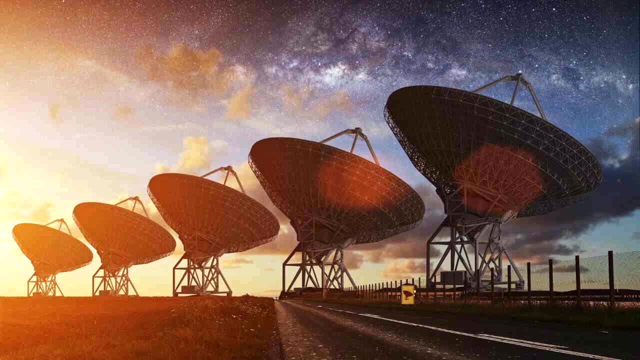 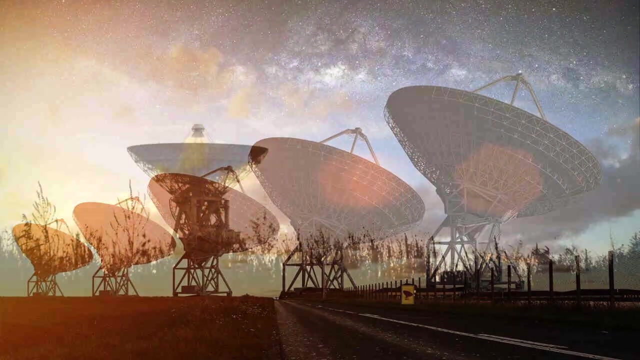 with electromagnetic radiation. That's what we knew how to do. We had radio telescopes, we had optical telescopes. Now, think about it, We are building, or talking about building or wishing to build, lots more large glass facilities on the ground and telescopes. 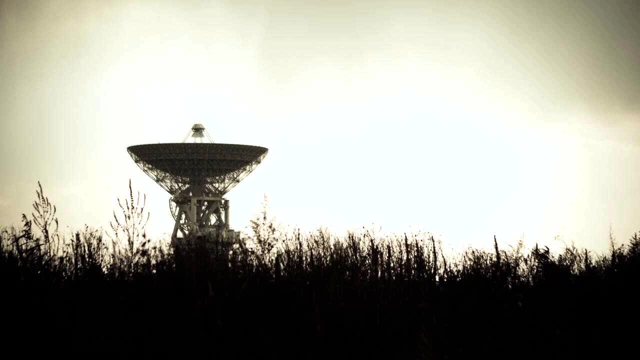 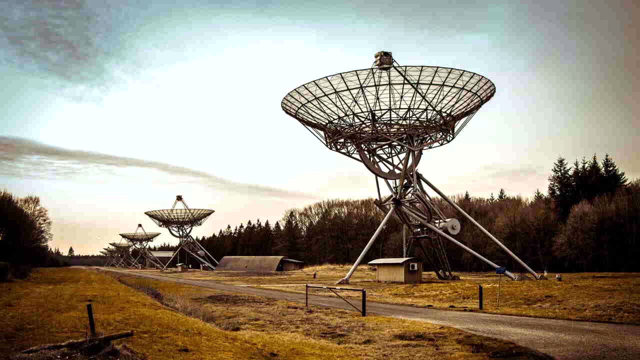 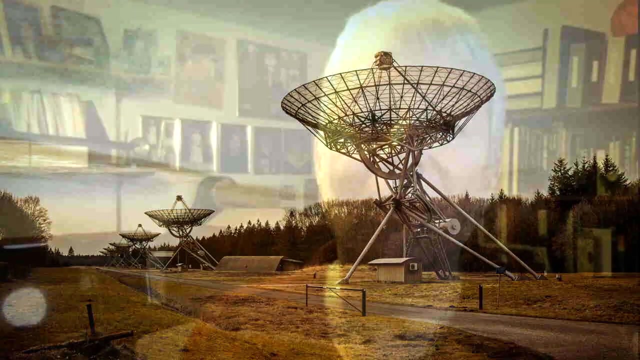 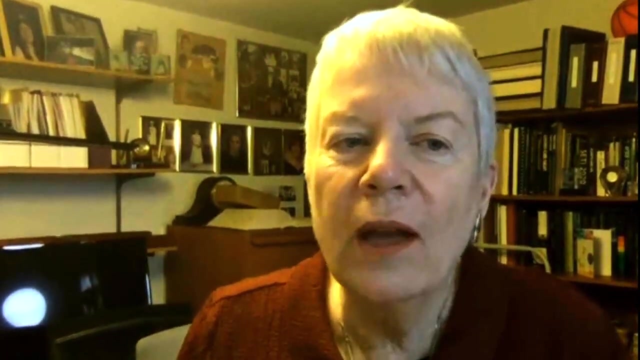 with lots of different capabilities in orbit, And these are being built in part to look for biosignatures. What else might they see that would indicate astroengineering, not just astrobiology, And so we've been trying to talk to the community about what might an engineered planet look like? 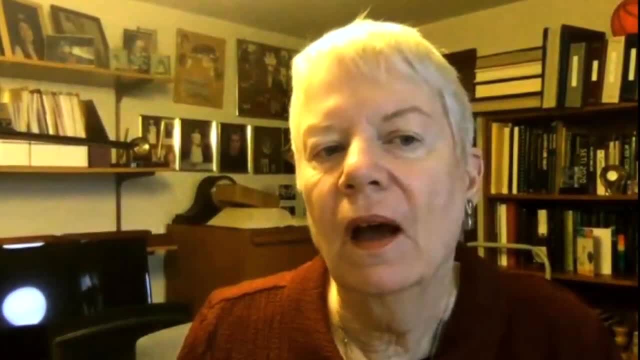 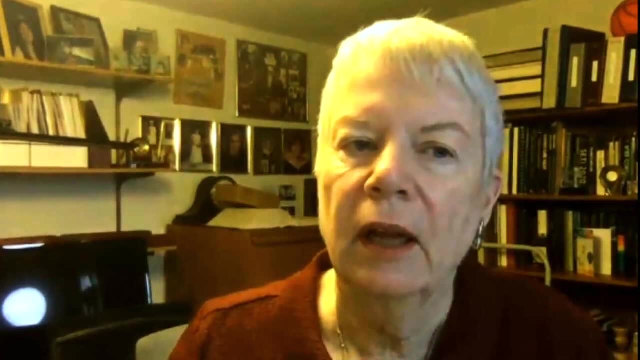 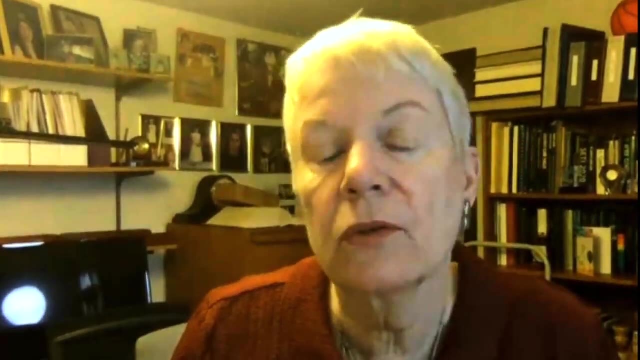 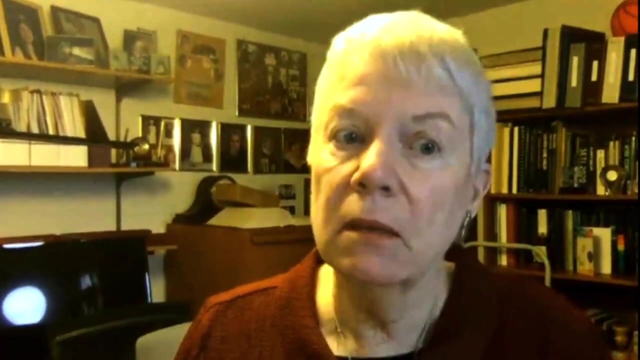 How might we tell something that is modified as opposed to natural out there? Big, large astroengineering project to capture energy might be one thing- Mirrors or Dyson spheres- But we also, when and if we get the capability to image these distant exoplanets. 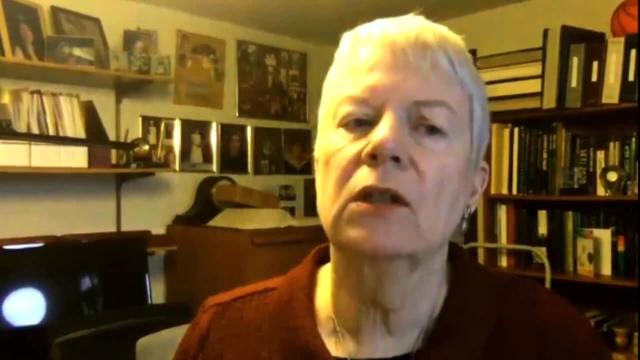 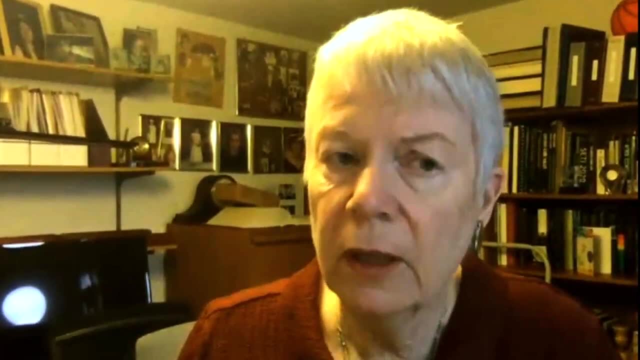 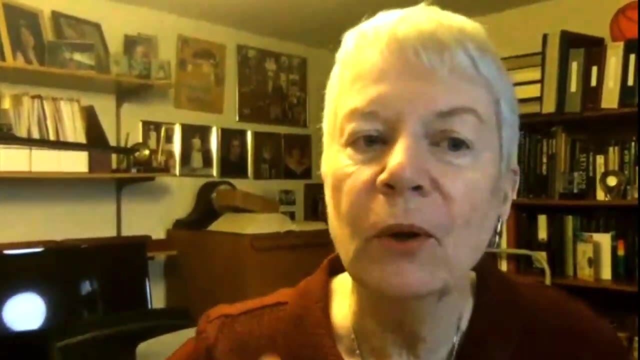 we might find that their albedo is strange, Their temperatures are strange, both of which could happen because of life. But if we find that their temperatures, for example, are uniform from pole to equator, maybe that's an indication that somebody is looking. to make more habitable real estate, to manage weather, do something that we can't do, that's for sure. but maybe another technology could Suppose. you look at the TRAPPIST-1 systems, right, Those seven planets all closely orbiting a red dwarf star. 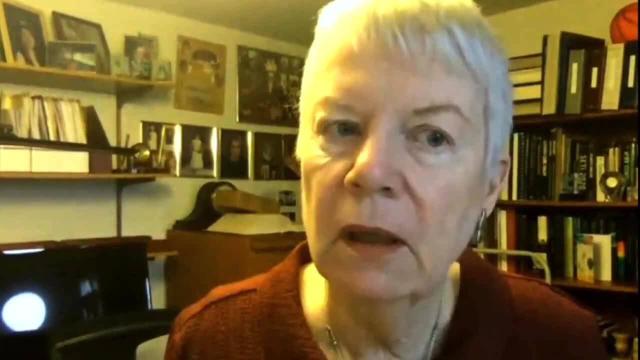 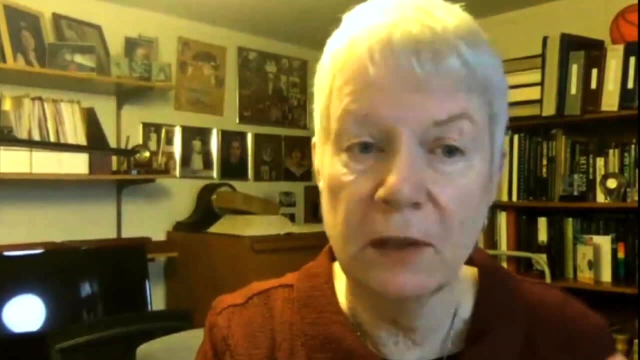 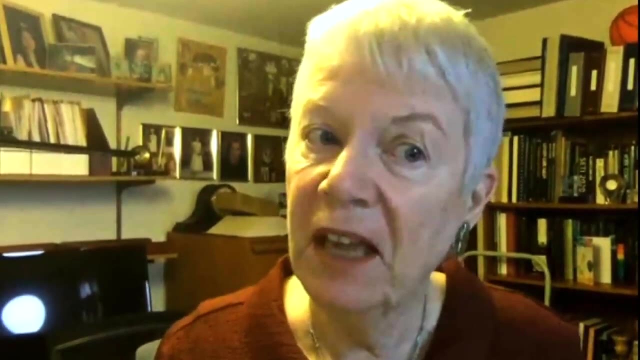 And when we get the ability to image them, we find out that they're all the same. right, They should be different temperatures because of their different distances from their host. But what if we find that they're all the same Again? maybe somebody needed. 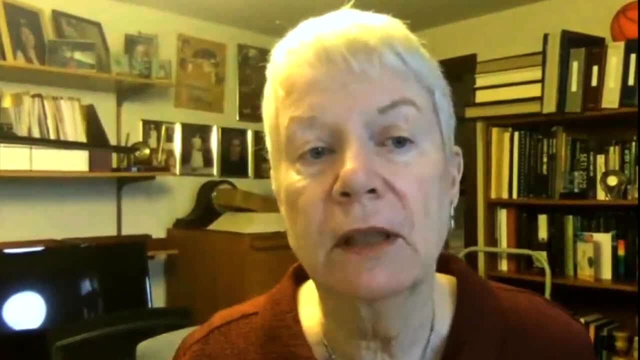 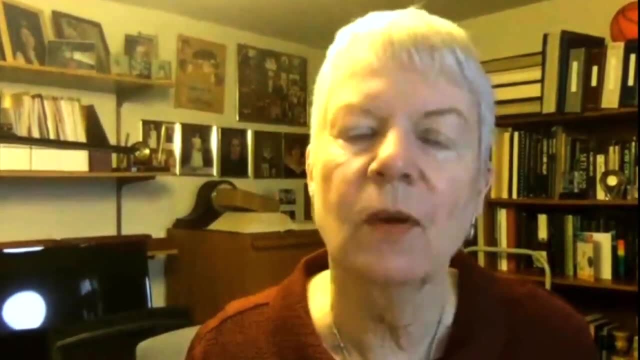 some more habitable real estate and decided to engineer some of those planets. It's this kind of thing, thinking broadly, technosignatures as well as biosignatures- Interesting. That makes me think a lot about David Grinspoon's recent book. 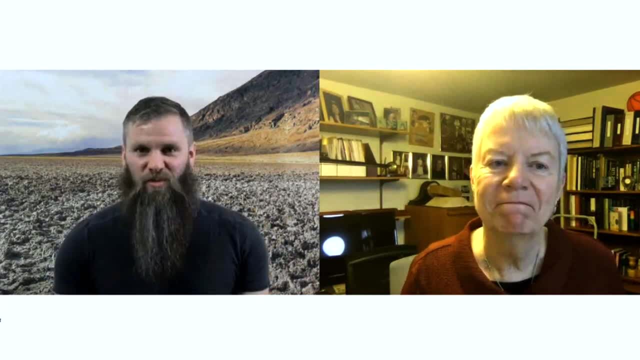 Earth in Human Hands and how he discussed that the future of humanity might be coming to the point of actually geoengineering our planet to, for instance, control our own climate, our own temperature. So I find it very interesting that we might look for 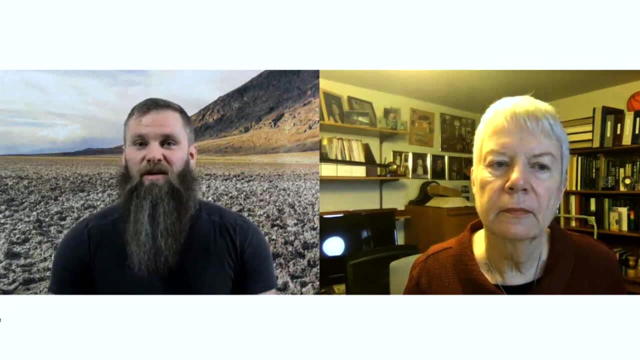 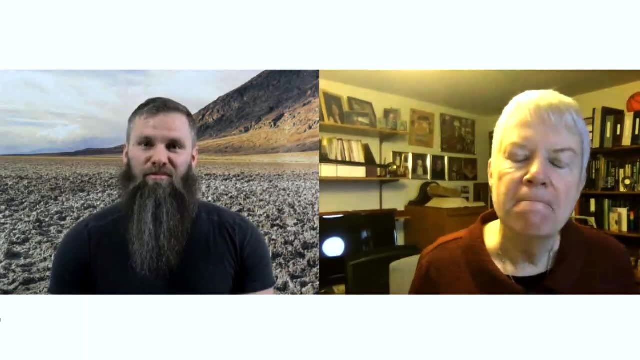 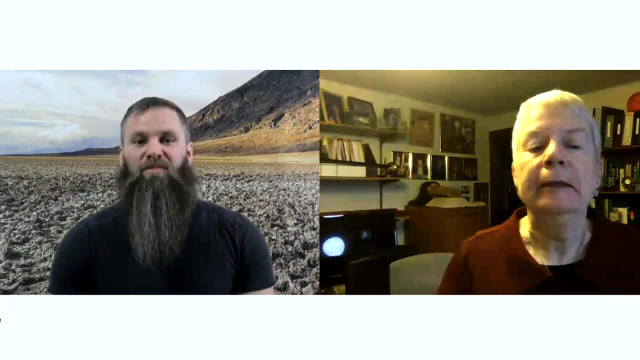 other civilizations who've gotten to that point already in controlling their own worlds. Well, you know, Arthur Clarke gave us three laws right, The third of which was: any sufficiently advanced technology would be distinguishable from magic, right, And we've sort of been using that. 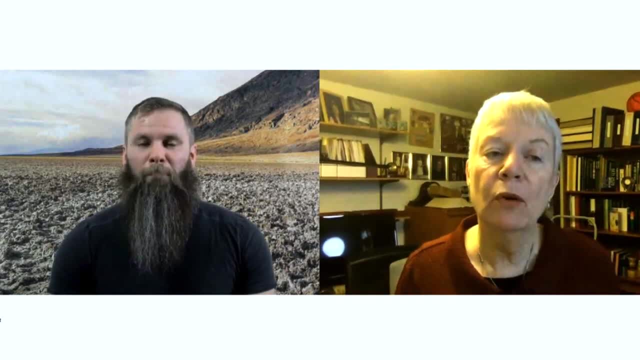 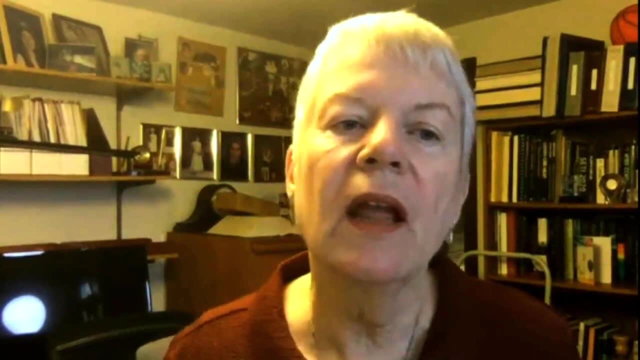 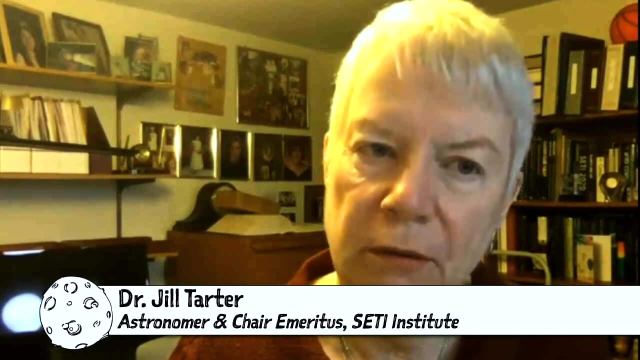 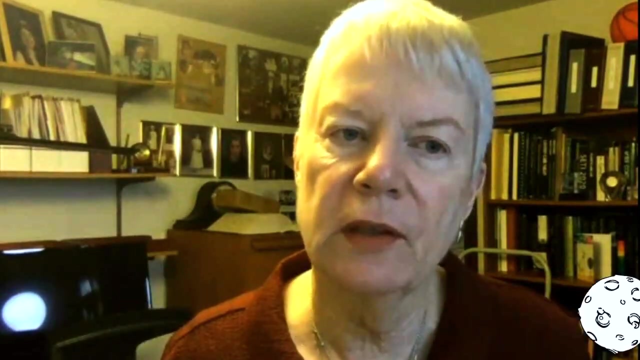 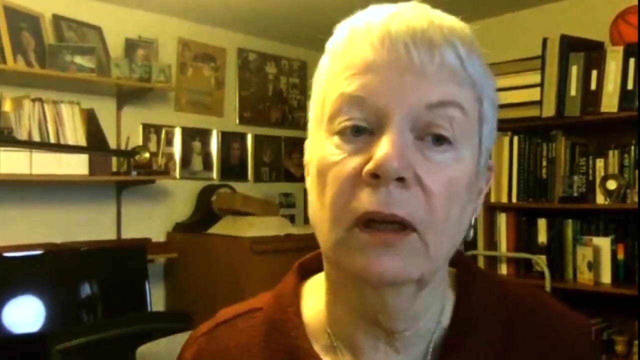 as a backdrop of our thinking. But more recently, a philosopher by the name of Carl Schroeder has suggested that any sufficiently advanced technology would be indistinguishable from nature. That is, that sustainability would require a technological civilization to become extraordinarily efficient and not put their planet out of kilter. 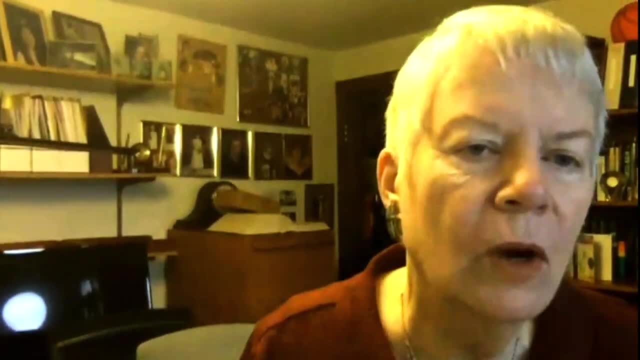 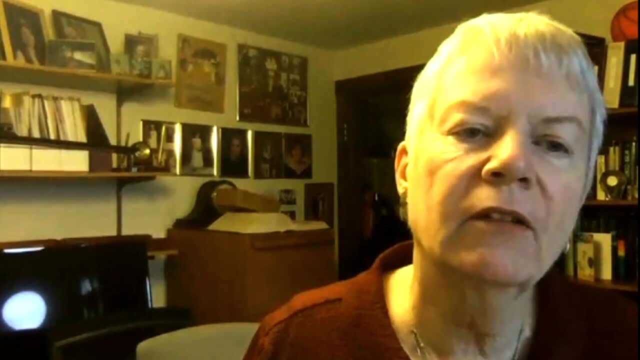 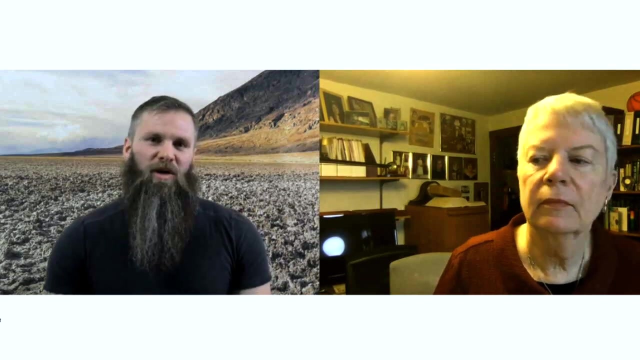 So scratching our heads about that one and thinking what would that imply in terms of interpreting the data that we're going to get back from these future missions? Hmm, interesting, Yeah. so kind of in that vein, I have a question I want to ask. 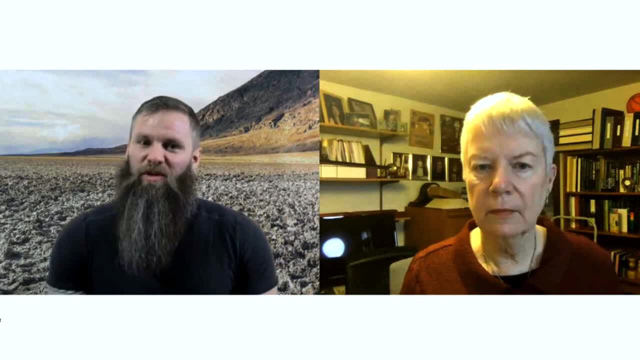 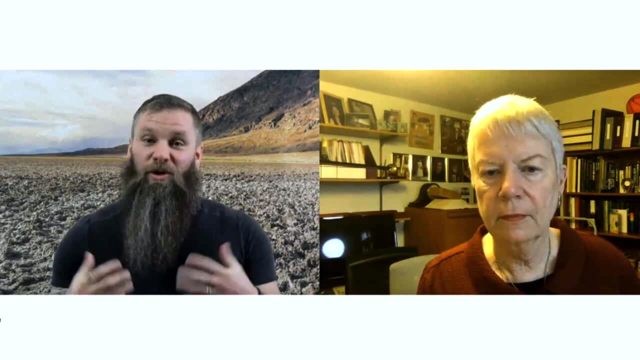 You were on an interview with Science Friday a couple of years ago and I heard a statement that you said that the 21st century will be the century of life on Earth and beyond. I wonder if you could speak more to what that really means. 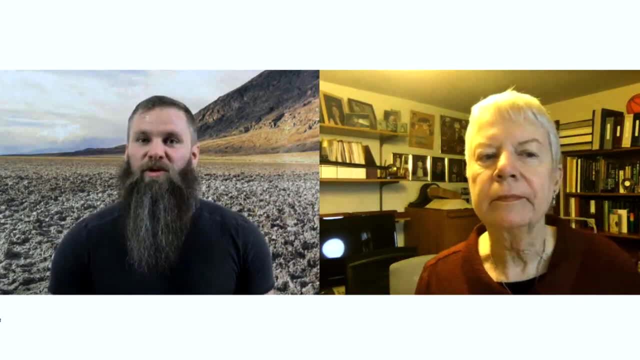 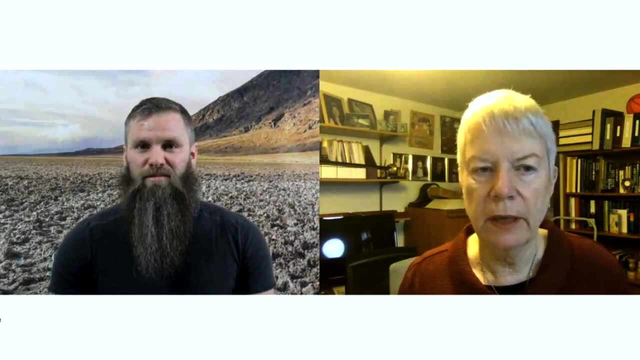 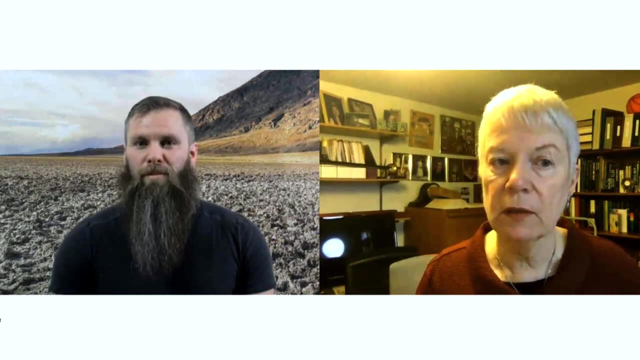 for our audience that this century might be the century for life. Well, this is taking off from a quote by Carl Venter and Daniel Cohen in 2004.. They wrote a paper that said: whereas the 20th century had been the century of physics, 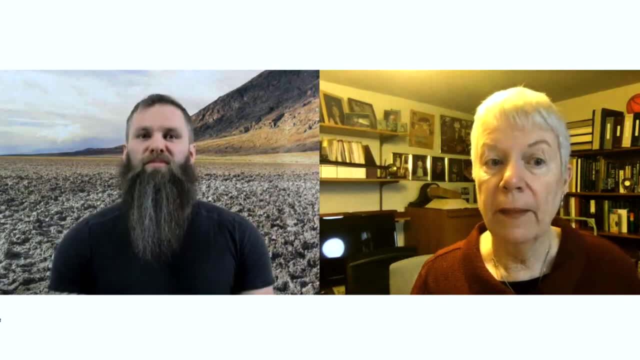 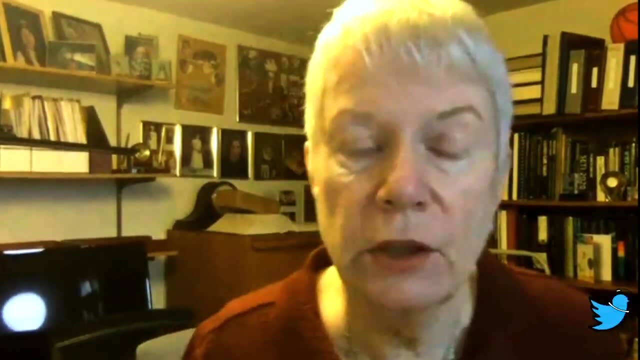 21st century was going to be the century of biology, And that was a real bold prediction. And they were talking about genomics and proteomics and bioengineering and all of this wonderful stuff Which is in fact paying off much quicker. 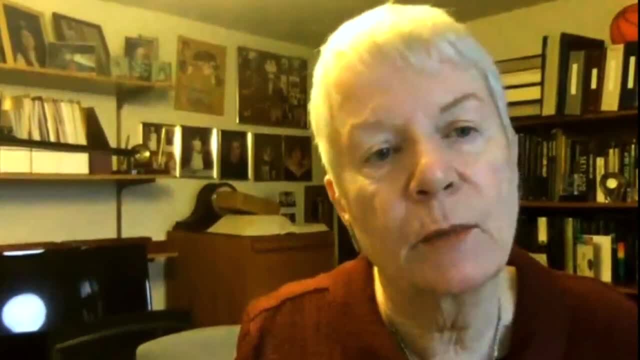 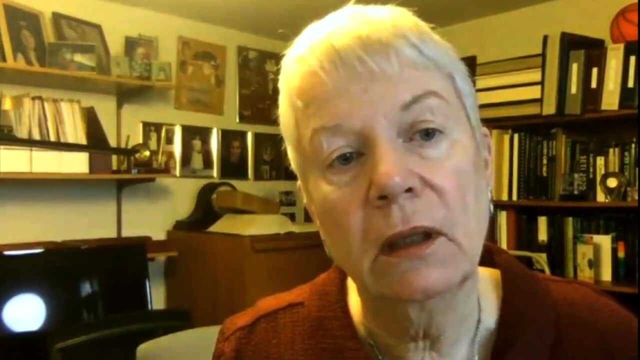 than they might have anticipated, But I think, as bold as that was not really bold enough, I think that this is going to be the century of biology, not just on Earth but beyond, Because I think there are a number of ways. 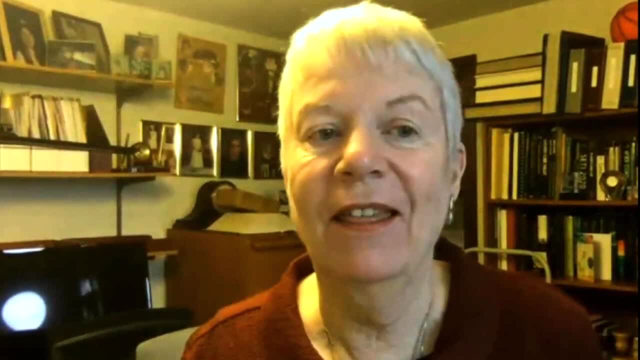 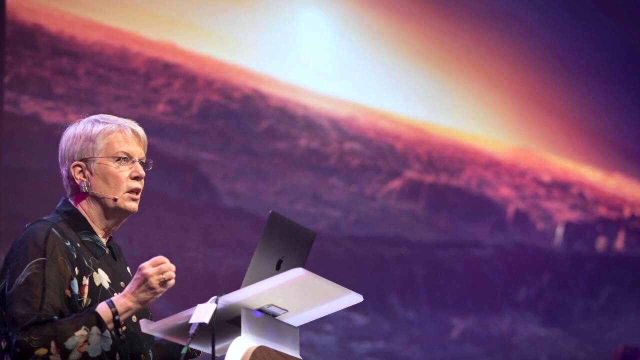 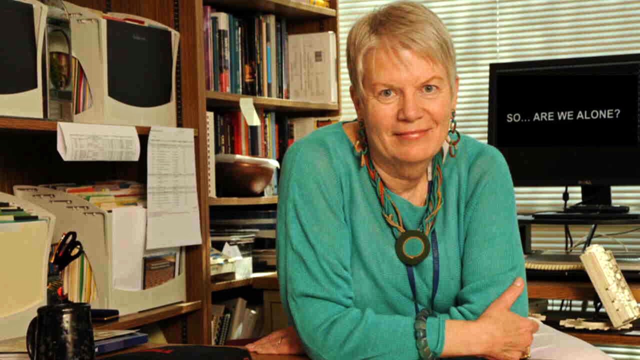 that we can detect biology this coming century. We can find it with the missions that are being proposed to look for microbial life, to look for the chemical signatures of life in the atmospheres of exoplanets. We might find evidence for extinct or even extant life. 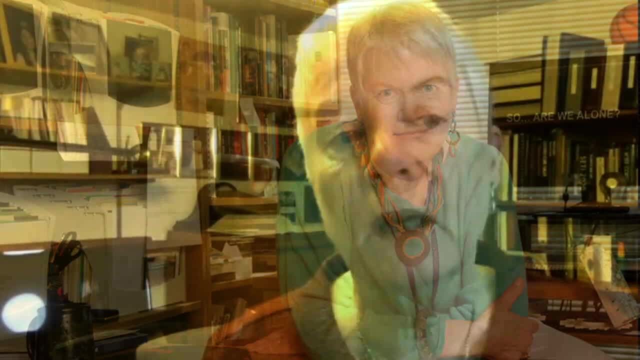 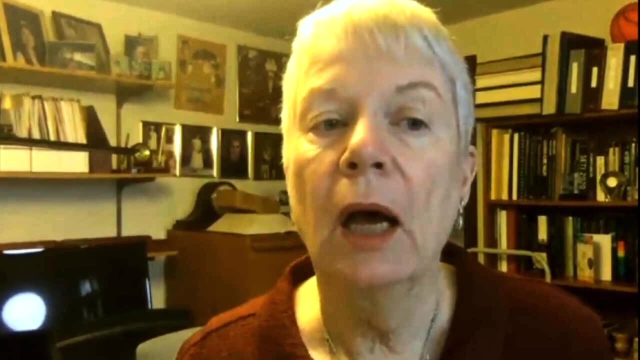 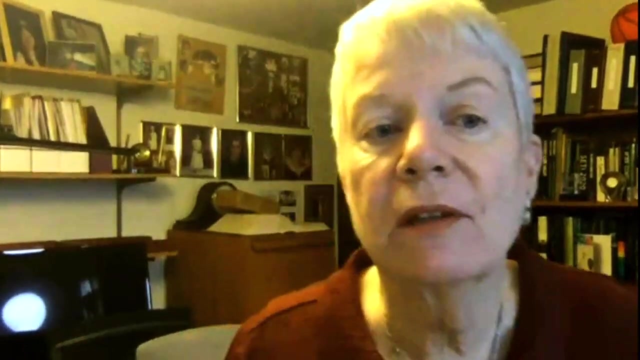 on some of the bodies within our own solar system as we get the opportunity to explore those robotically or in partnership with humans, And we might in fact, as we're looking for something else, stumble across evidence of huge astroengineering projects. And lastly, 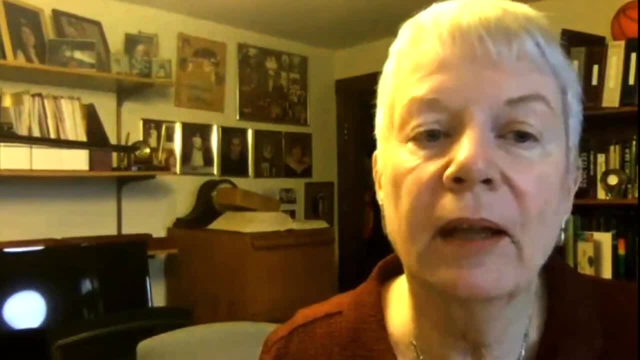 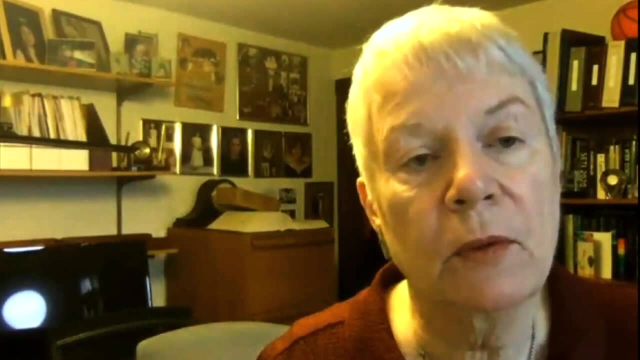 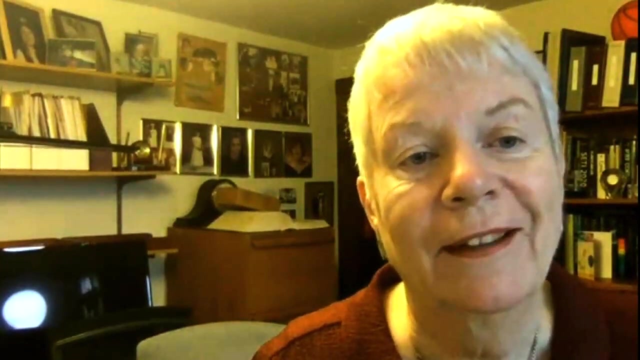 we might take it there Right. We might, by going to the Moon and to asteroids and to Mars. we, in fact, might be responsible off this planet. So I think this next century is going to be incredibly exciting, right, And I wish I could plan. 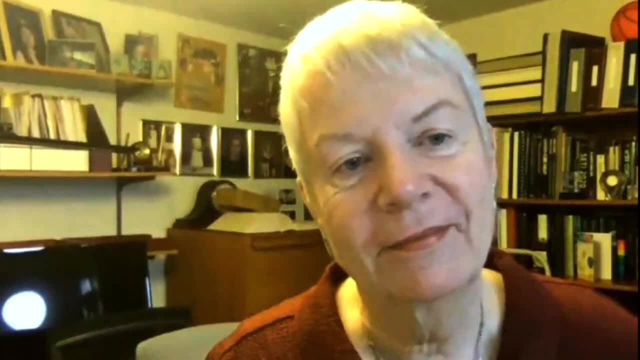 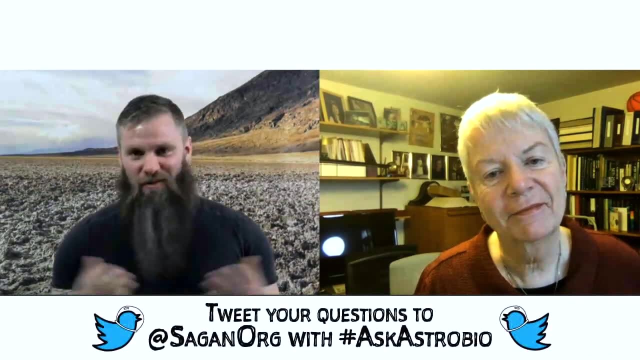 to stick around to the end of it to see how it all works out. Yeah, no, kidding, That's wonderful. Yeah, it's kind of interesting just to think about what's coming right now For all of us in astrobiology. there's so many things. 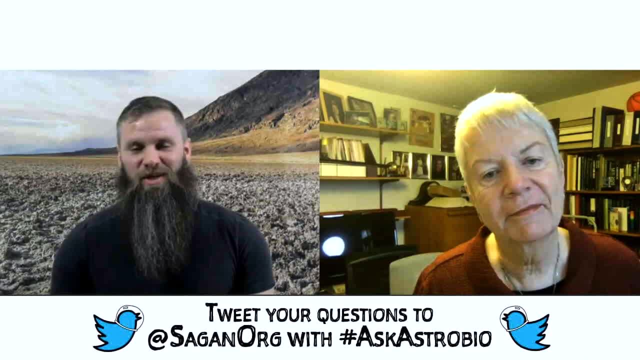 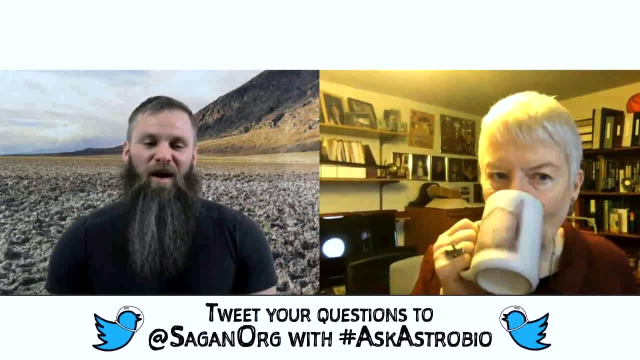 Like you mentioned, we have spacecrafts studying our solar system, We have telescopes on Earth and in orbit studying exoplanets, And we also have SETI. I wonder if you could, for our audience, tell us what you think right now is the most important thing. 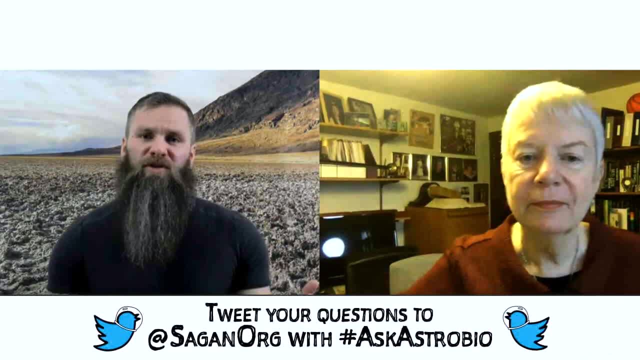 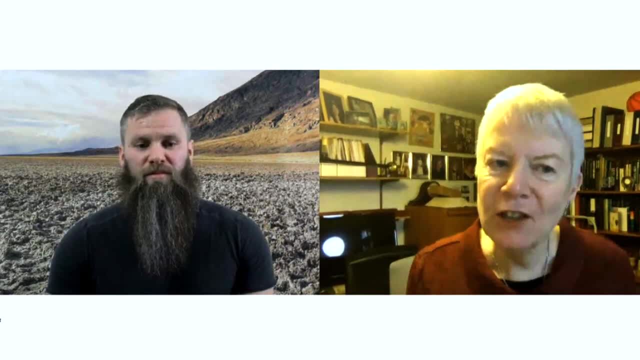 not just for SETI right now, but for the future of SETI as well. You know I missed the end of your question. You said not just for SETI right now, but But for the future of SETI as well. 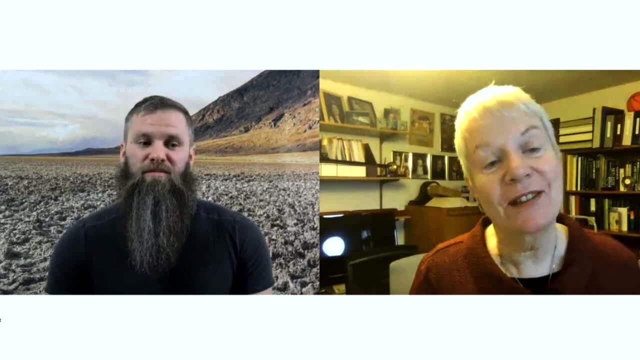 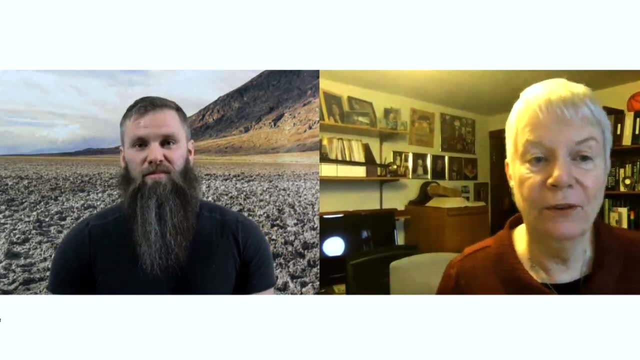 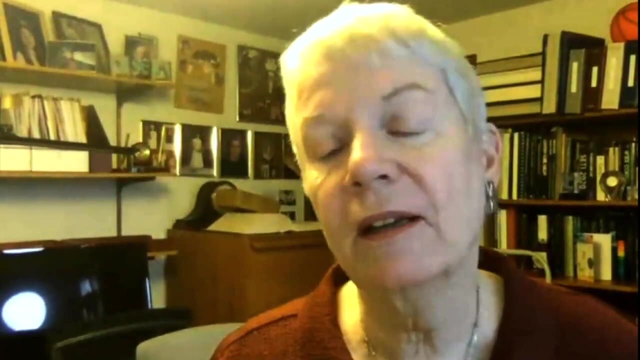 Okay. Well, the answer to that question is pretty simple. It's a sustainable funding profile, right? SETI's funding has been a roller coaster historically And we need to put it on a stable platform. We need to find a way to fund projects. 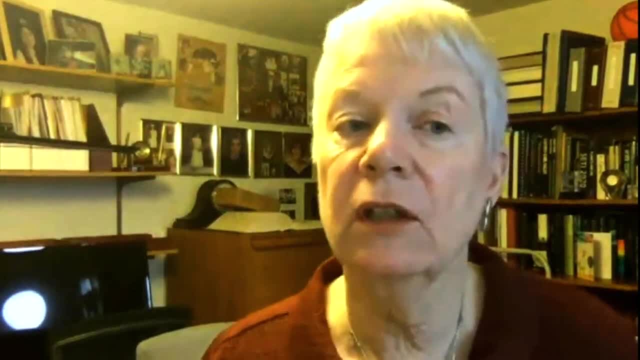 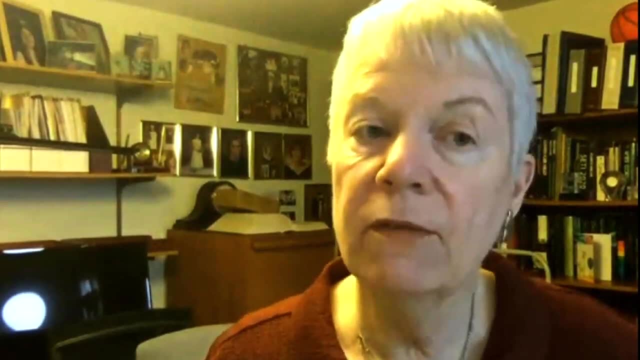 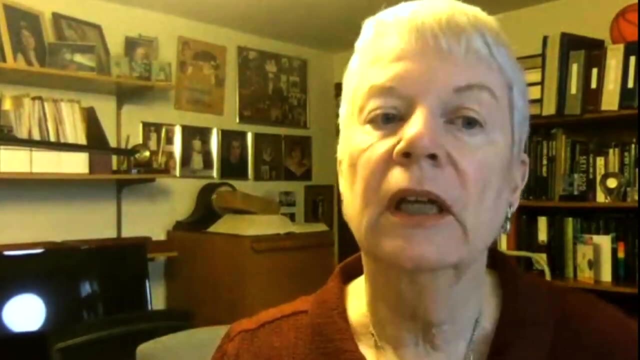 that have a very long horizon, potentially before they pay off. The high energy physics community and the gravitational wave community have been able to do that when putting funding, year after year after year after year, into building instruments that weren't good enough when they were turned on. 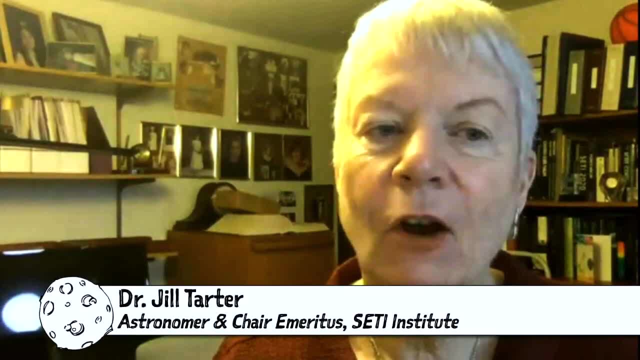 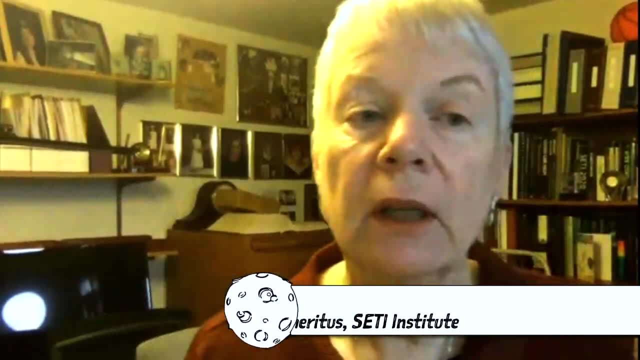 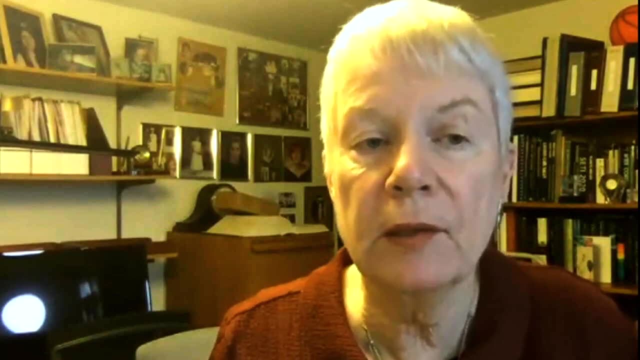 and got made better. We need to find a model for that, Hopefully at a lower price tag than building LIGO or the Large Hadron Collider, But a model where, because we have some sort of dependable funding base, we can in fact attract the best and the brightest. 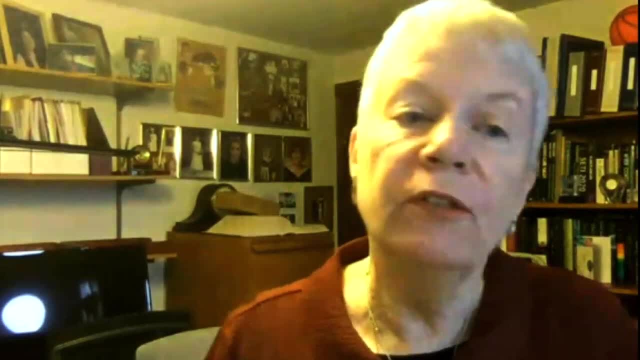 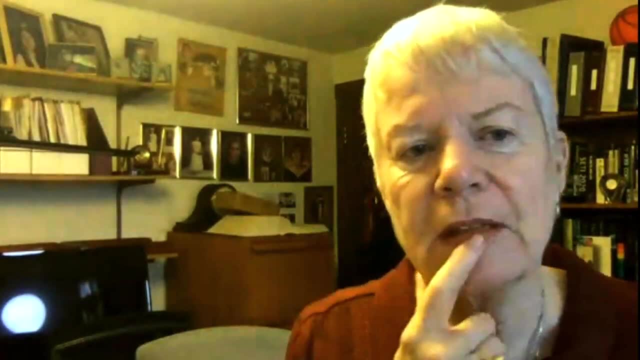 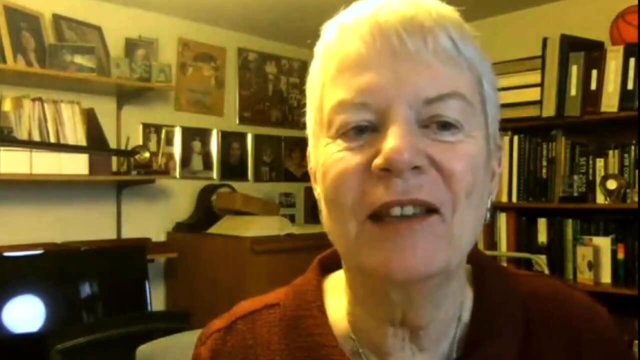 You know people are excited about this field. But if you tell them, oh, this and the other thing, but maybe I can't pay you next month, That's a little bit close to home right now, But seriously having a funding base. 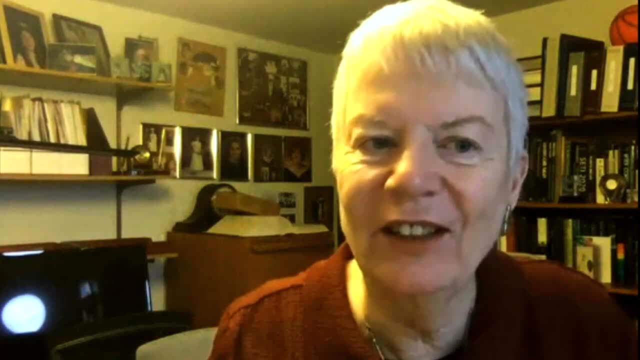 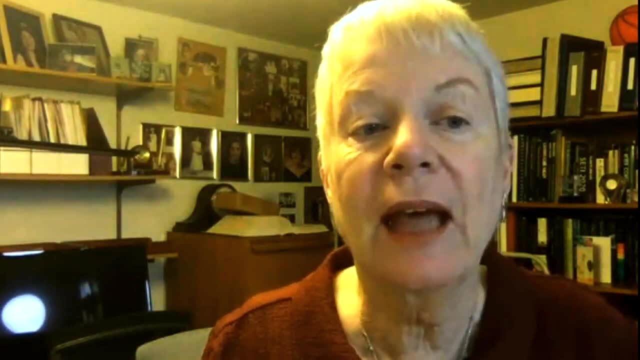 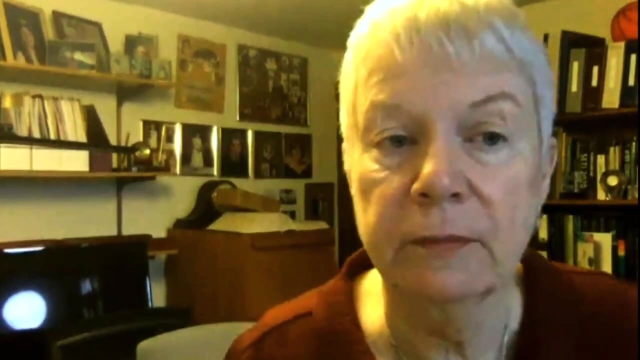 will allow us to take on very large projects that provide us with huge improvements in our capabilities and will allow young people with great ideas to become part of this exploration. Awesome, yeah, I think we have some of those best and brightest watching our show right now. 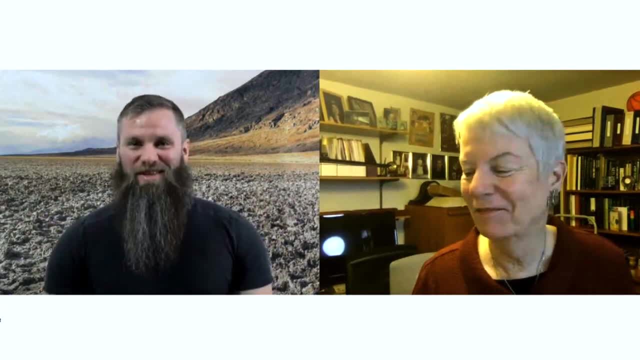 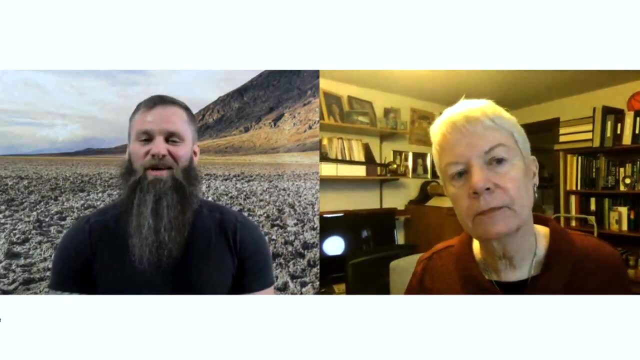 So you know if you're out there, you know these are things you can do now. So before we do open it up to questions from the audience, I do have a couple of fun things I want to bring up For one, 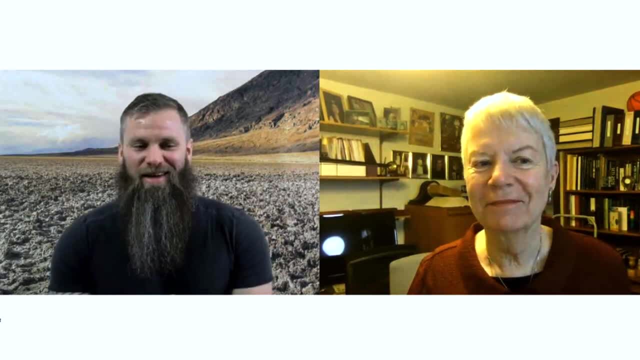 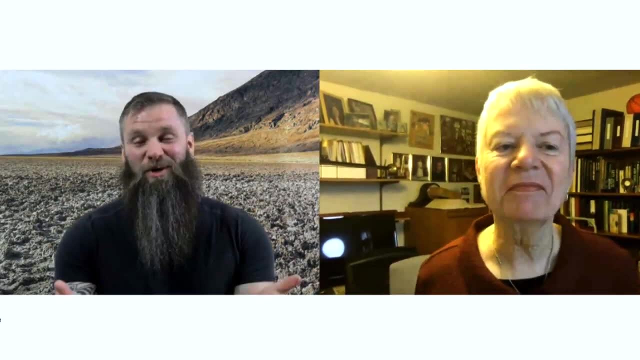 David Grinspoon, had posted on Twitter last year some pictures of you fixing a model of the Green Bank Telescope At the SETI Institute. I wonder if you could explain, since we're going to show the picture right now for our audience. if you could explain. 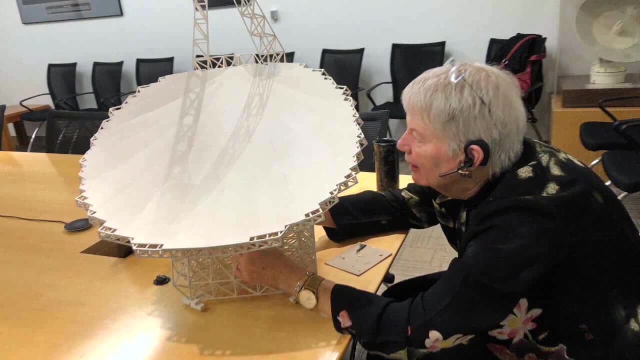 what's happening in that picture? Well, the Green Bank Telescope is a wonderful example of an offset Gregorian design, which means the telescope feed doesn't come up from the middle of the telescope, It actually hangs off from one side. And now 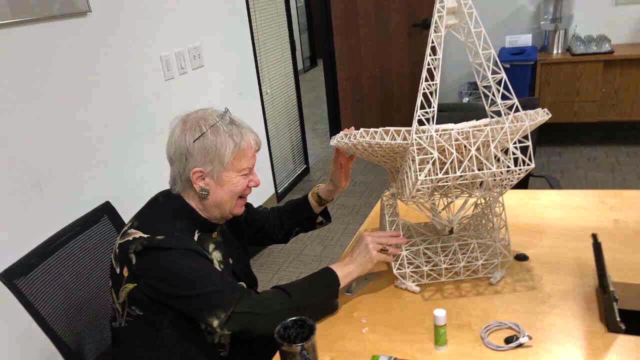 you can decide if you want to do it from one side or from the other side of the telescope. You can decide if you want to do it from one side or from the other side of the telescope. You can decide if you want to do it. 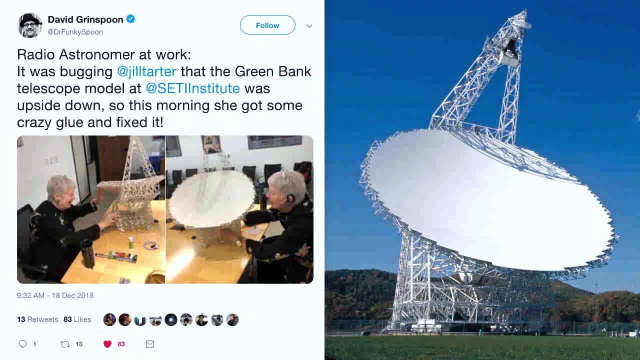 from one side or from the other side of the telescope. And now you've got a telescope to hang your feed up high or hanging off the bottom down low. And the Allen Telescope array has a feed low configuration but the GBT has a feed. 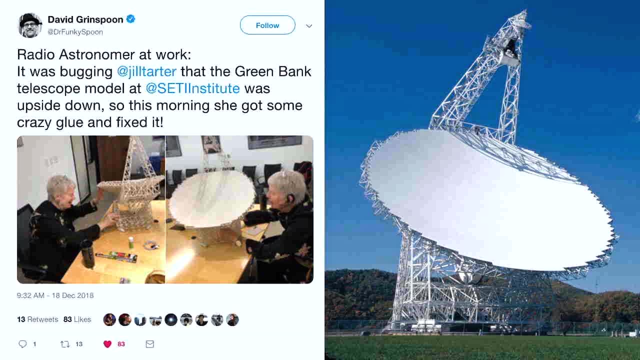 high configuration And we have this beautiful model at the SETI Institute that, with moving around and changing offices, et cetera, had gotten broken And its its broken position had it lying down with its feed on the ground, And now 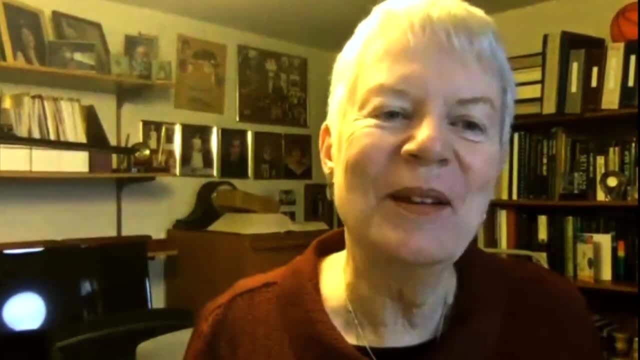 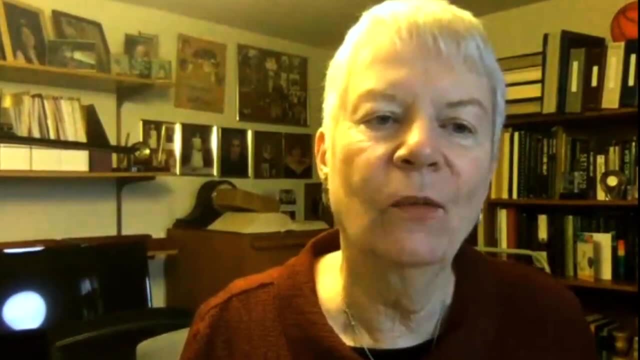 you can see that the feed is now up where it should be, And so, now that it has become a viable SETI instrument being used by the Breakthrough Listen project, I really felt that we needed to have it presented correctly, So I was early. 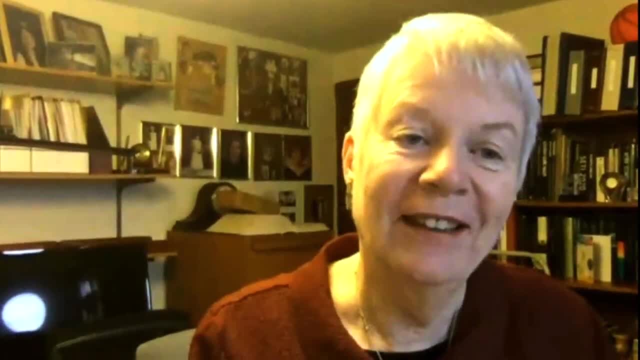 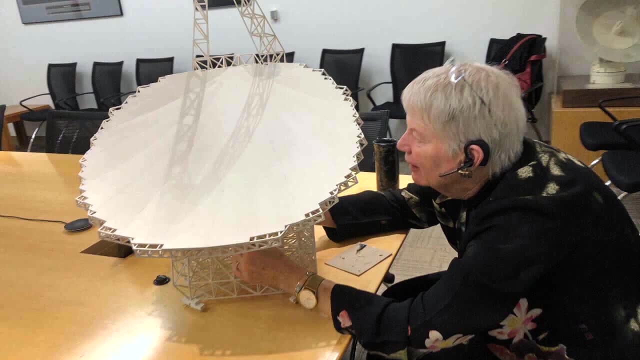 for a science advisory board meeting one morning and I got out the super glue and the scissors and the tools and I fixed it so that the feed is now up where it should be. I felt very good about that. Yeah, it's perfect. I mean. 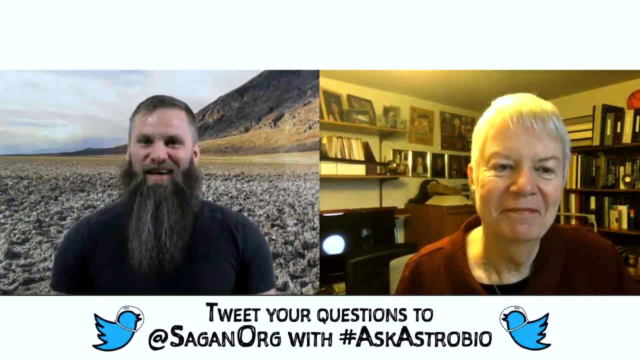 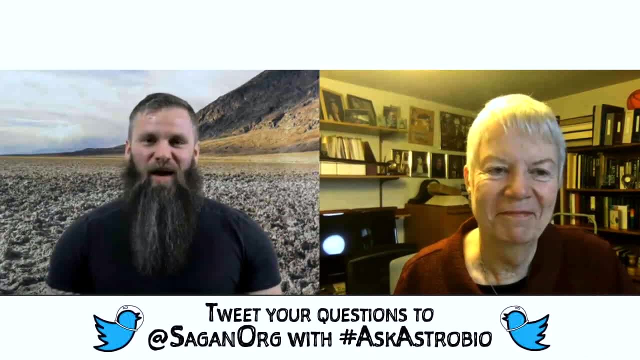 there are things you know that need to be fixed. I mean they're kind of messed up like that. Engineers do that You know they see things that aren't exactly the way that they are in nature. We question why. 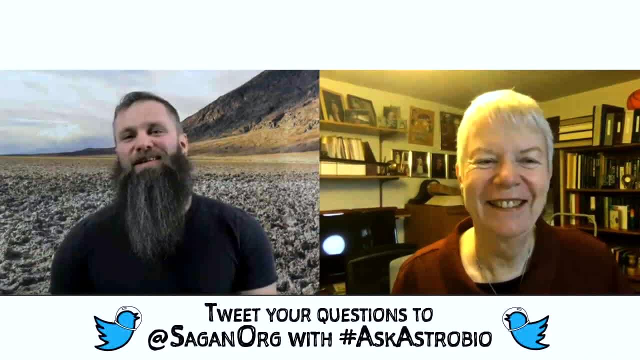 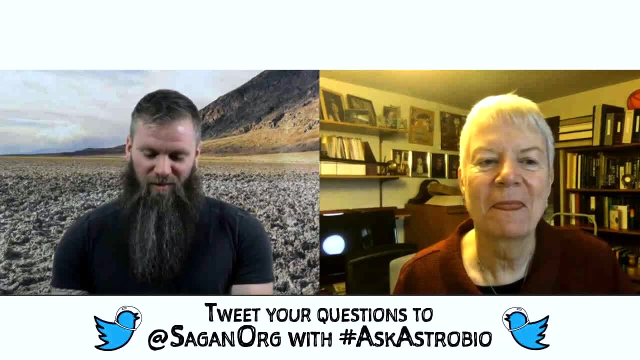 And I love that. I would be remiss if I didn't bring up contact and what it was like having Carl Sagan and Andrew tell you that you were the basis, in some ways, for this character of Ellie Arroway. Can you tell us what that was like? 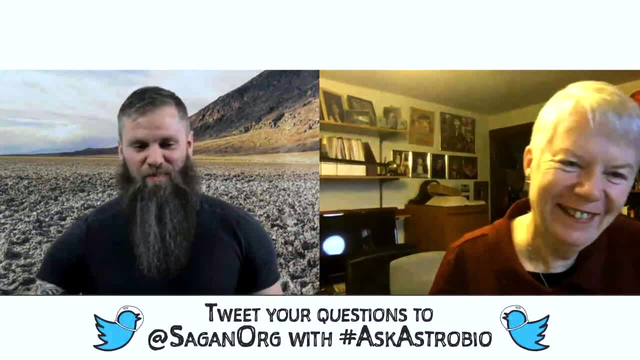 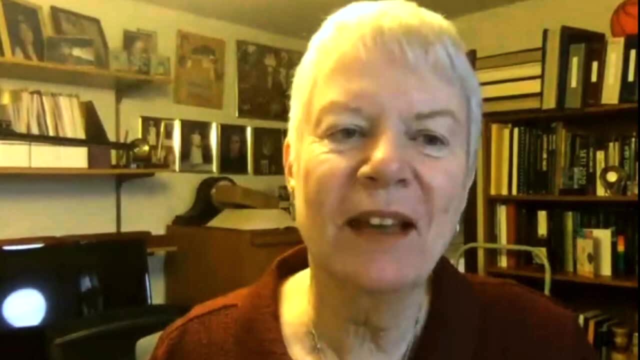 when you found out that you were in a relationship with Carl Sagan. Well, it was a long time ago, It was in the mid-80s. Carl was a colleague and I actually happened to be back at Cornell for a meeting and Carl said: 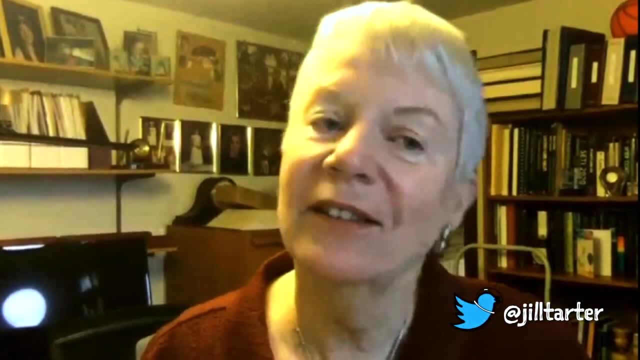 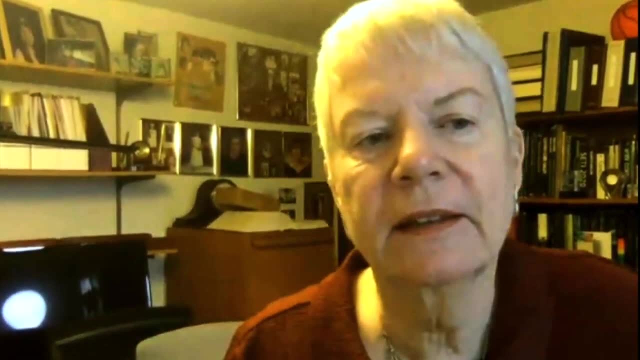 come on up to the house. We're having a cocktail party. So I dutifully went up to their beautiful house in the hills and they took me aside, Anne and Carl, and they said Carl's writing a science fiction book. And I said: 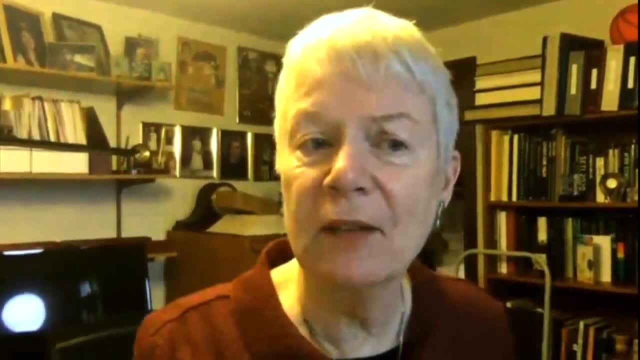 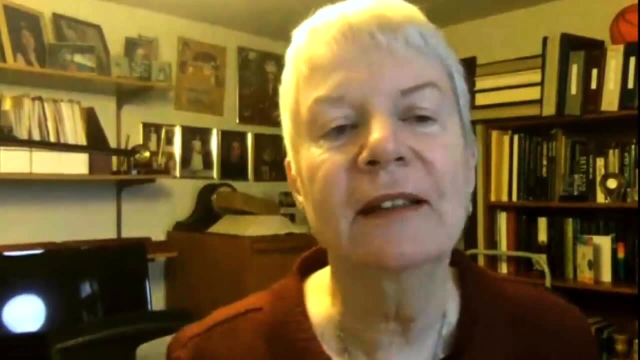 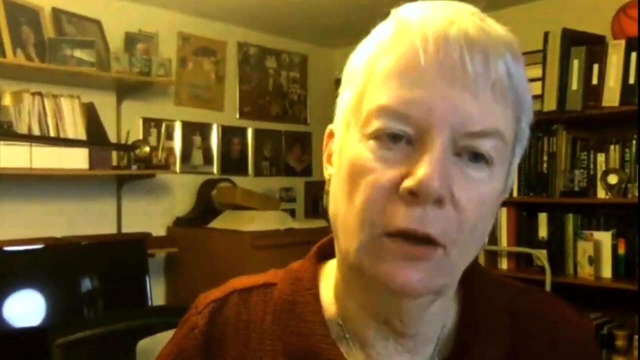 oh, come on. The New York Times last weekend told us what kind of an advance he got and we're so bloody jealous, right? And they said: well, you may think you recognize someone in the book, but I think you're going. 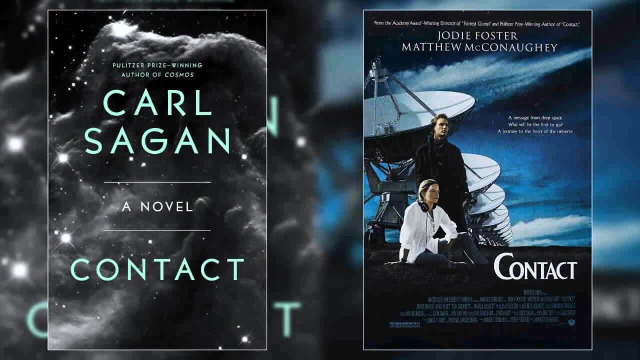 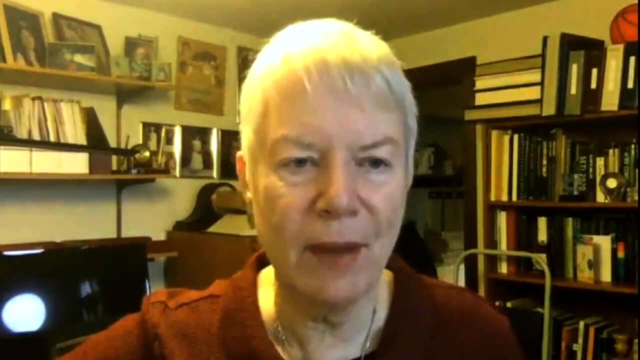 to like her, And so I said: oh my goodness, Look, just make sure that she doesn't eat ice cream cones for lunch, because that was something that I got teased about at lunch to walk from our laboratories over to the Baskins. 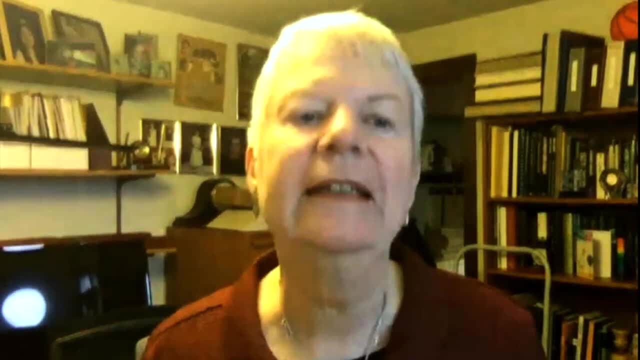 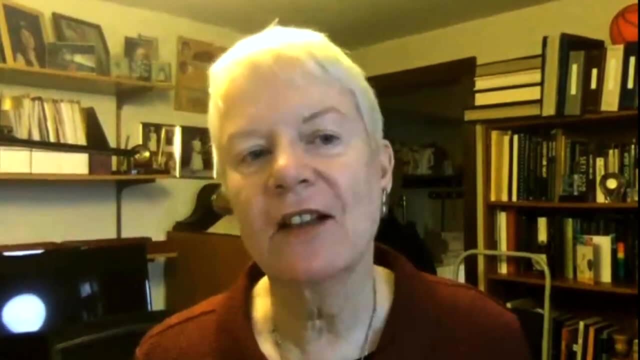 and Robbins on the base and get ice cream cones and walk back right, So I could have my pleasure and get my steps simultaneously. And I thought, well, as long as that characteristic isn't there, nobody's going to think it's me. 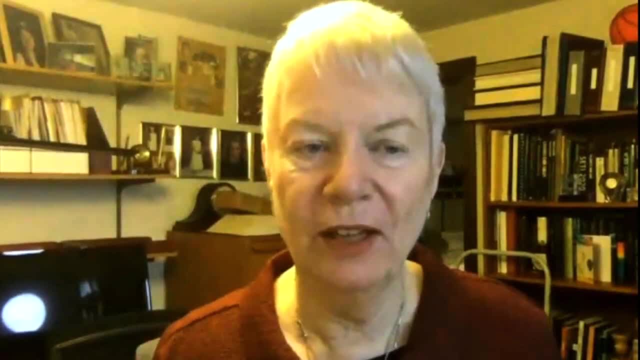 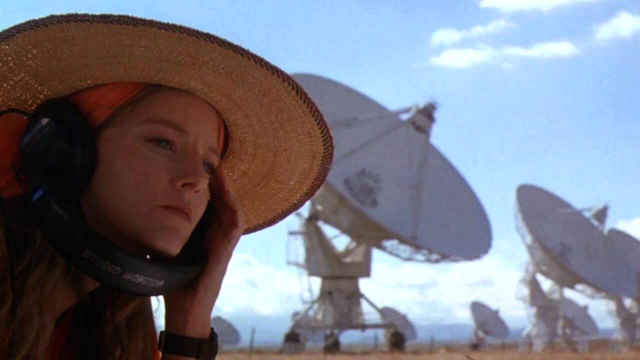 Well, it didn't exactly work out that way And I had a great time when this book turned into a movie. It was a real privilege to be a brilliant, wonderfully good actor, very kind person, And we had a lot of fun. 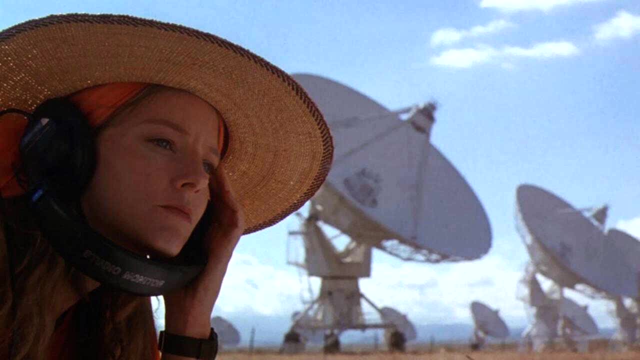 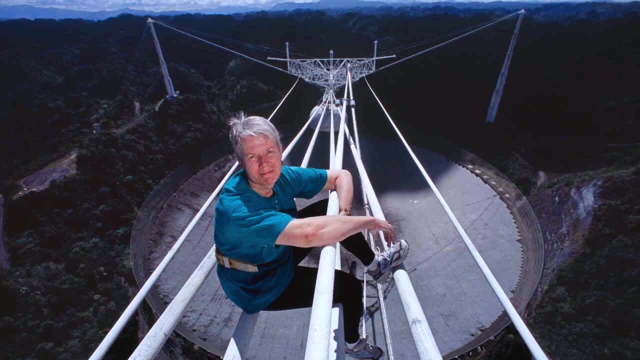 And actually I was down at Arecibo when they were filming there. Sadly I left too early to prevent the huge innumeracy that's there. But while I was there I just was fascinated by all their gear They've got. 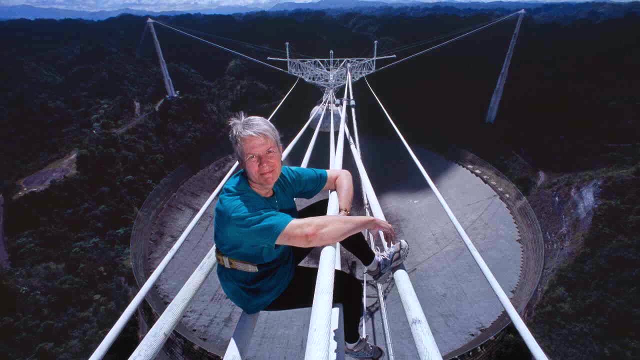 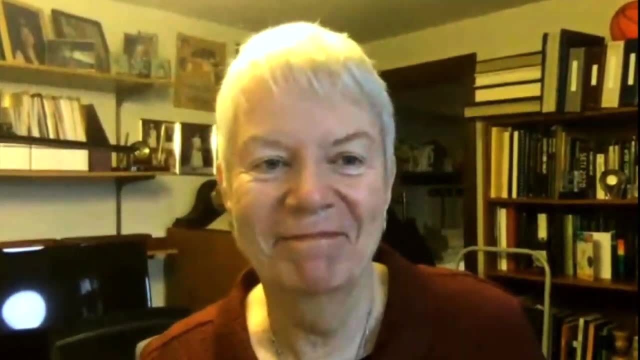 really good technologies And I was thinking, hmm, I can make movies if I can't make it in SETI, right Yeah, absolutely. I think a lot of people who are interested in astrobiology interested in this idea of are we alone? 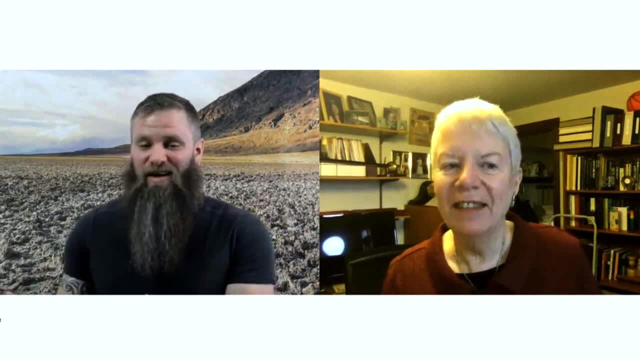 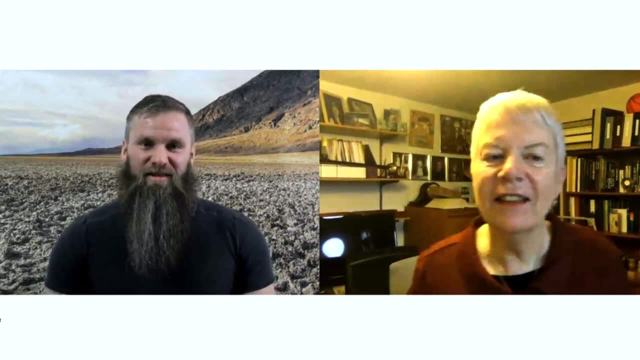 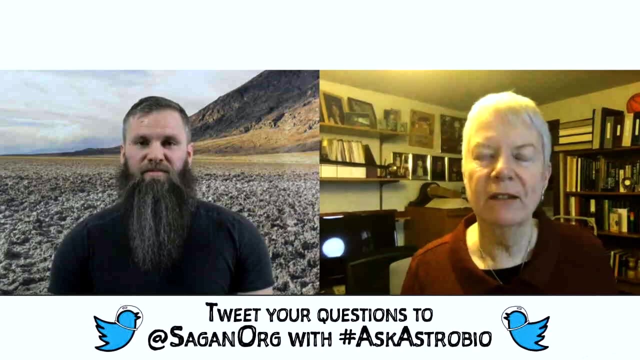 are also huge fans of science fiction, And so things like contact inspired so many of us, And it'd be kind of cool to have that chance to see. I think science fiction is great because it gives us an opportunity to think about things that we can't conceive. 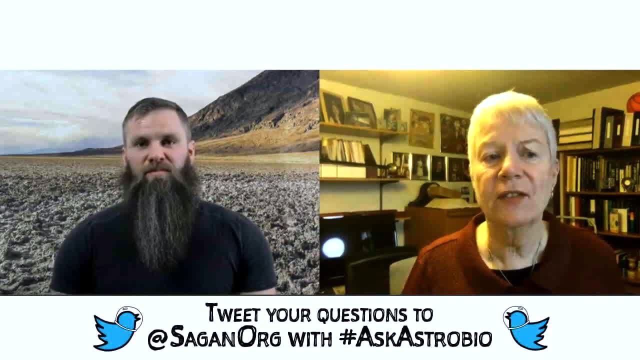 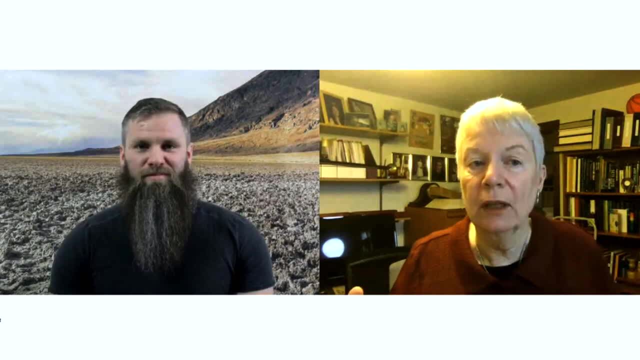 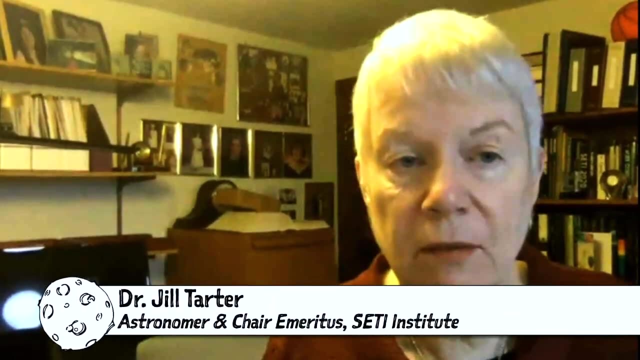 of. I mean, one of my favorite science fiction stories is Fred Hoyle, cosmologist wrote a story about a plasma cloud that was intelligent and causing us unintentionally blocking the sun as it came to visit us. That's a type of intelligence. 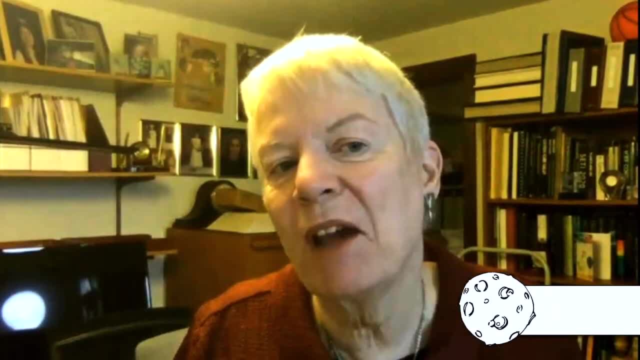 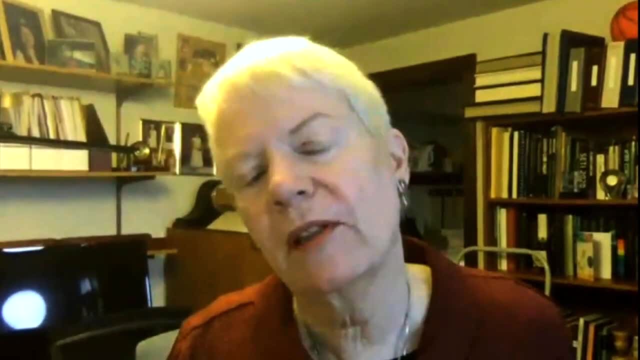 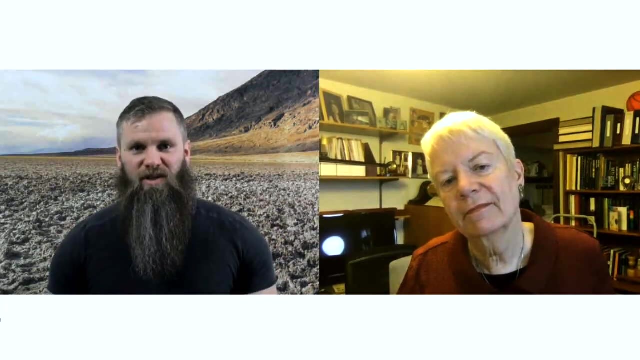 I might not have thought of, But now that I've read that book there's some little piece of my mind that's open to that idea Interesting. yeah, It's interesting how science fiction kind of gives us a way of seeing ourselves in settings. 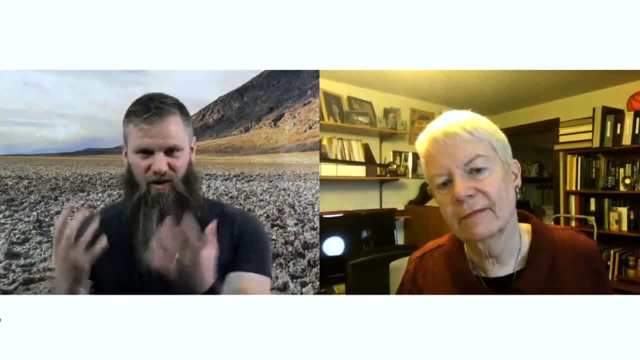 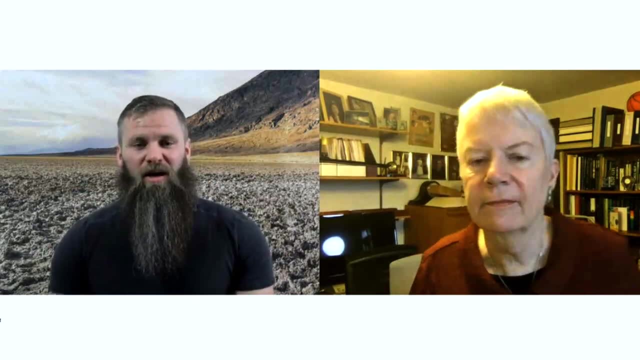 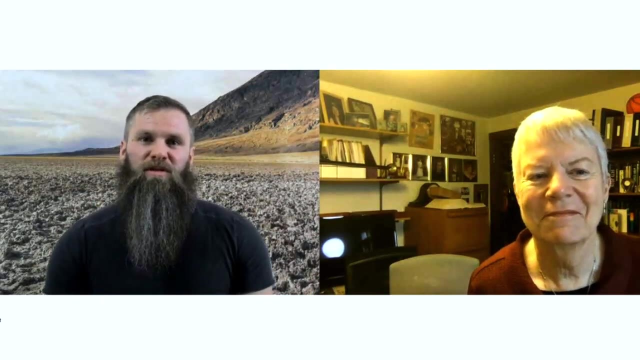 in different time periods. I do have to ask: if Carl Sagan was here right now and was writing the novel Contact right now, or if the film Contact were being made right now, what would Carl do in 1985 when the novel was? 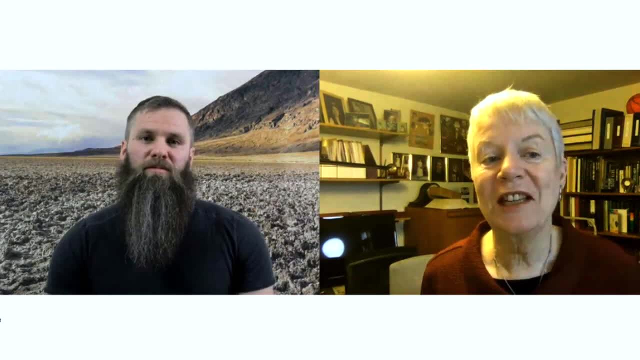 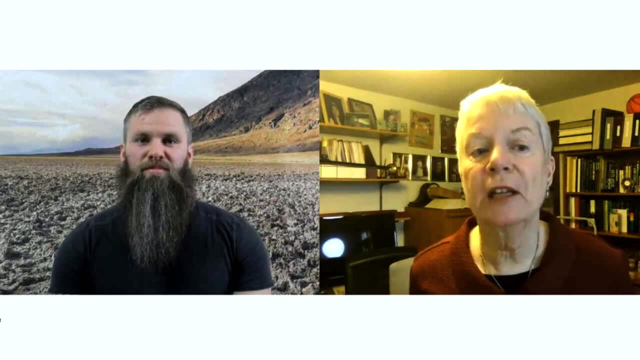 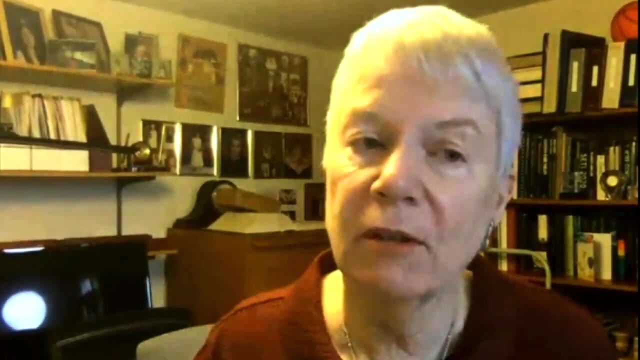 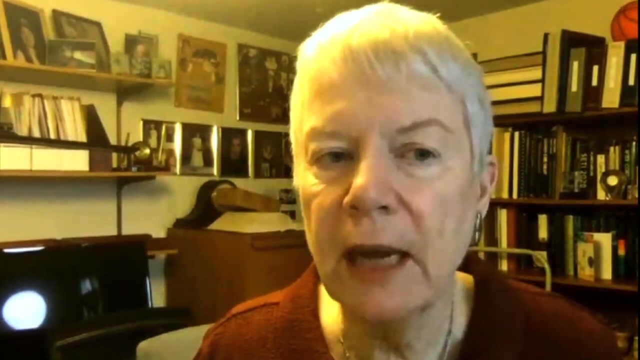 first published. Well, Carl was prophetic, unfortunately, in terms of understanding that, whereas we were a government program and fat, dumb and happy in some sense, we would face termination of the funds and then be struck with the difficulty of going back to. 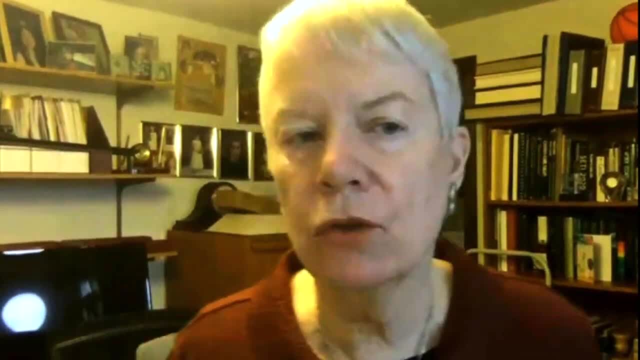 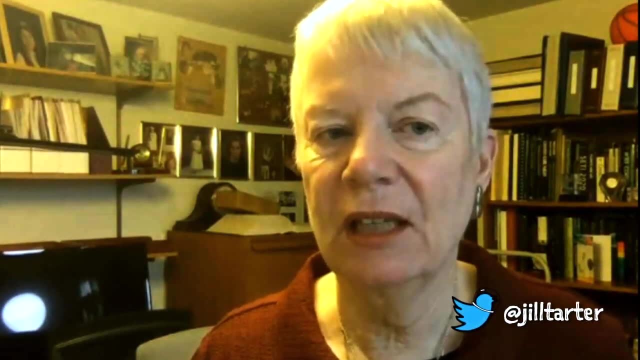 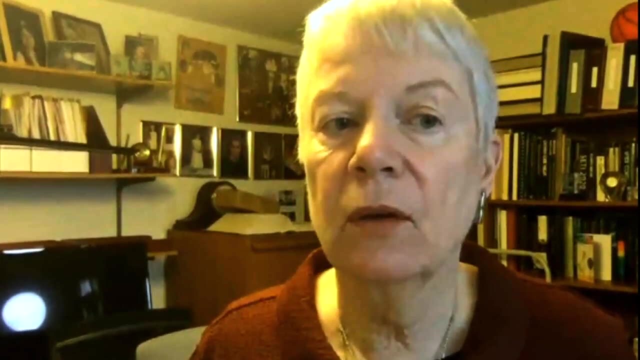 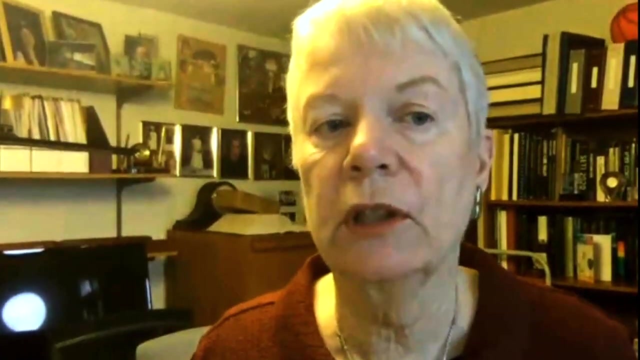 where we were, And I think what would be different now would be a larger concentration on private funding being sufficient, or at least maybe just adequate, to take on the challenges of space flight. So I think he would be having a lot to say about SpaceX and Blue. 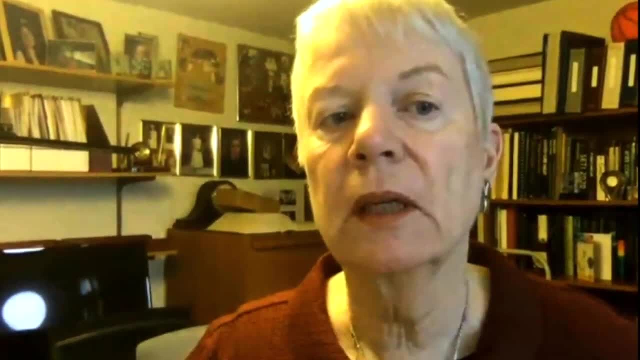 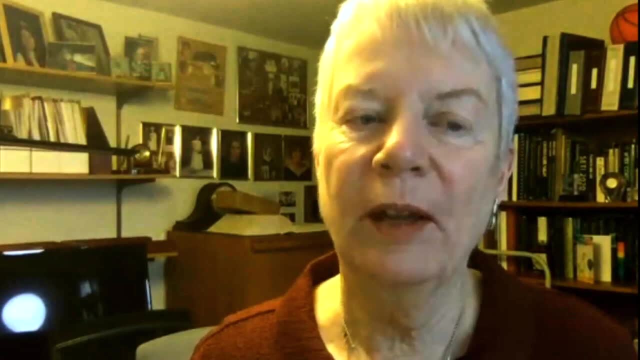 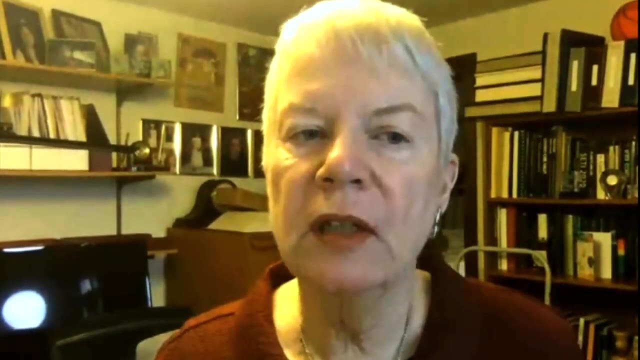 Sky And I think Carl would be fascinated to see where that was going. You know things have changed a lot. I mean for the generation coming up right now. you know, for them it's a different way of doing it. 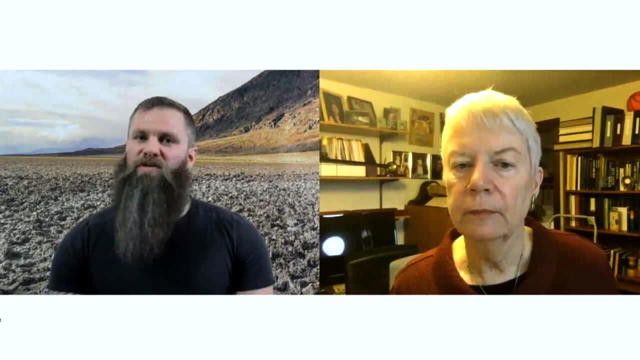 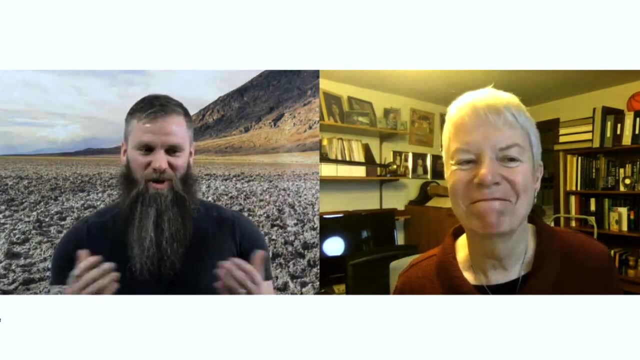 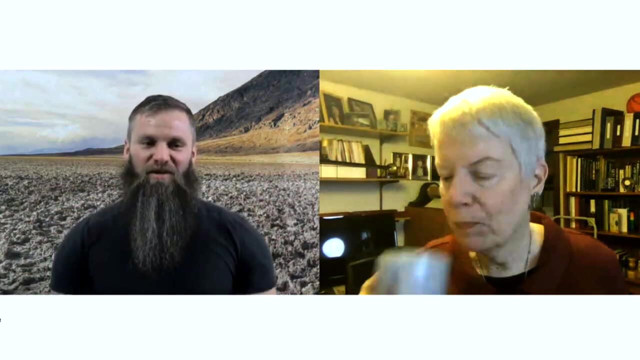 And I think Carl would be fascinated to see where that was going. You know, for them, we've always had people in space, in orbit, And we live in a time where we have private companies developing rockets and we have, you know, Breakthrough. 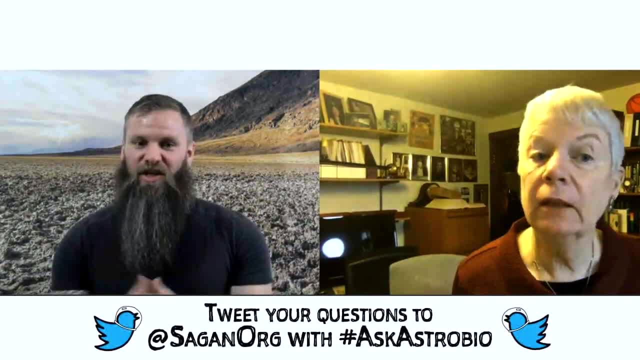 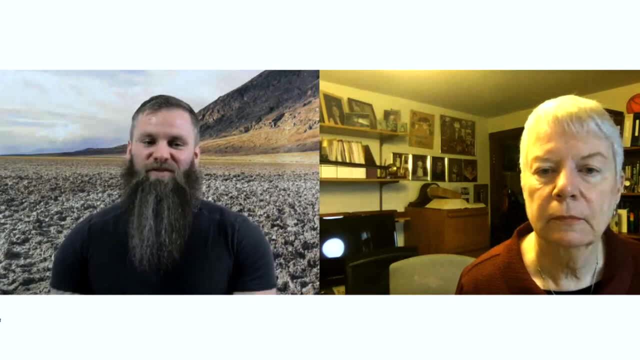 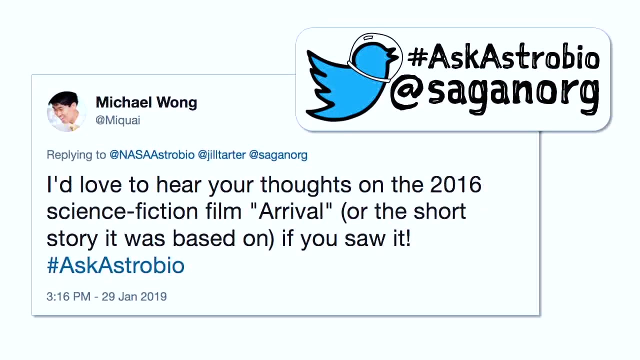 and SETI and these different companies, these organizations kind of you know, taking on some of these tasks themselves. But I think it is a good time now to hear your thoughts on the 2016 science fiction film Arrival. if you saw, 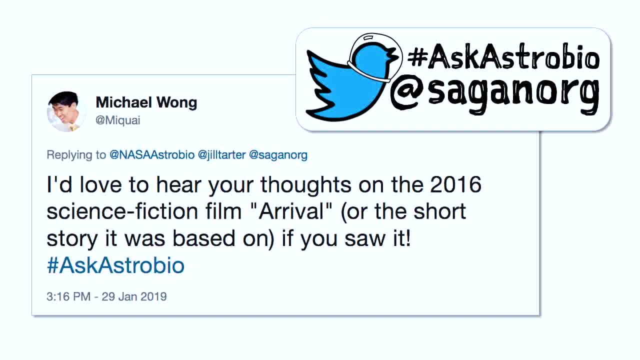 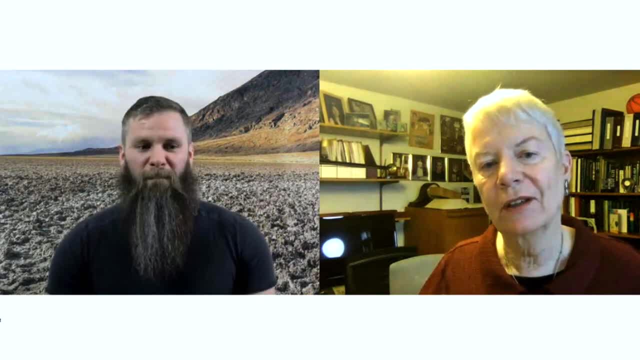 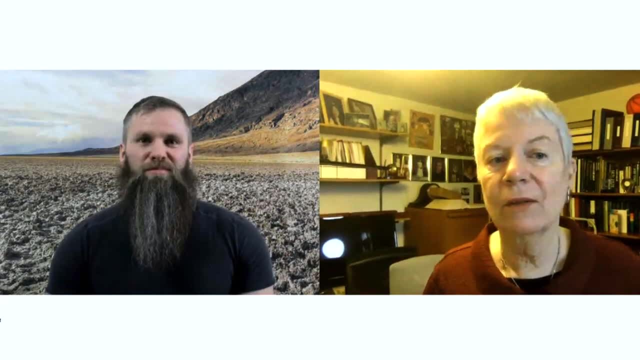 that I saw it and I loved it. I just I keep trying to wrap my head around the fact that if you're going to write in circles, you have to know the future, And I think that's such a mind exploding concept. 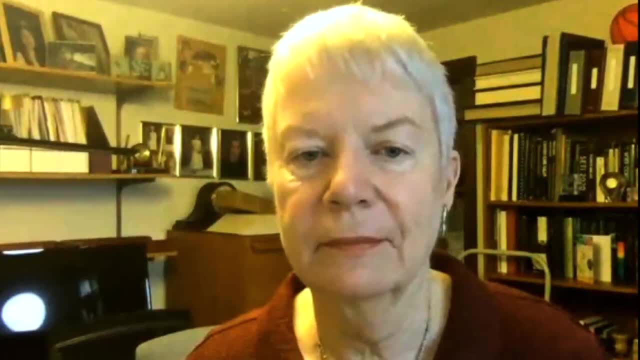 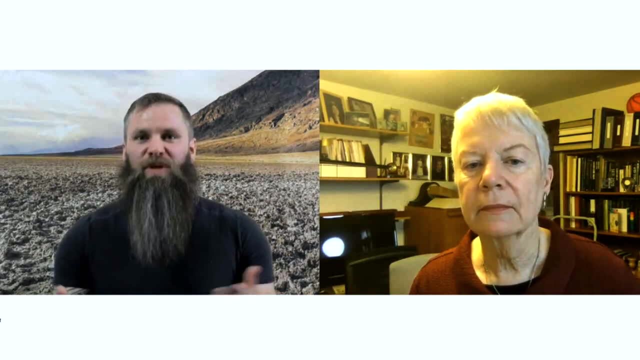 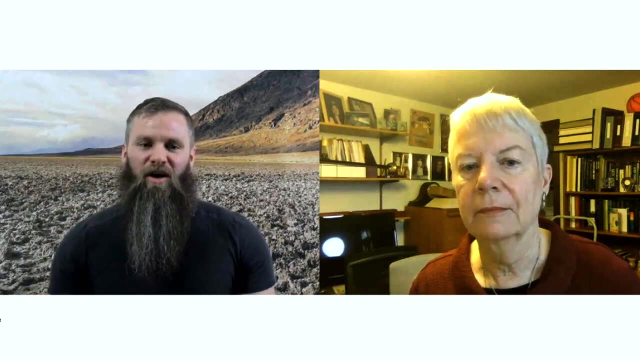 Great, I really liked it. Yeah, me too. It seems like SETI and people you know who are really thinking about SETI deeply are also people who are considering what language would be like if it were different from the way that we use. 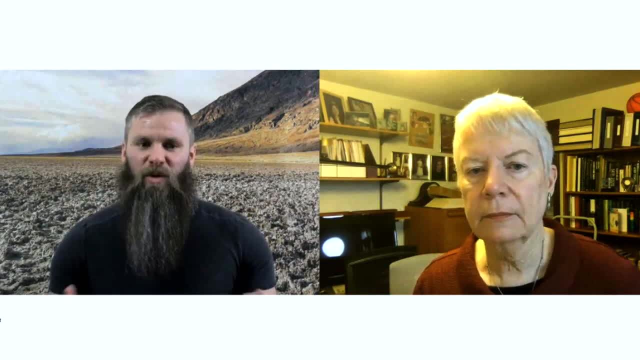 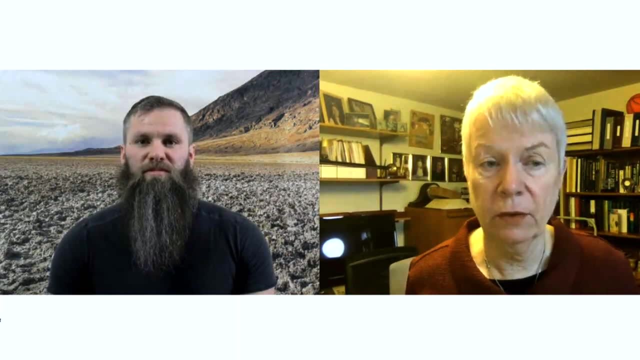 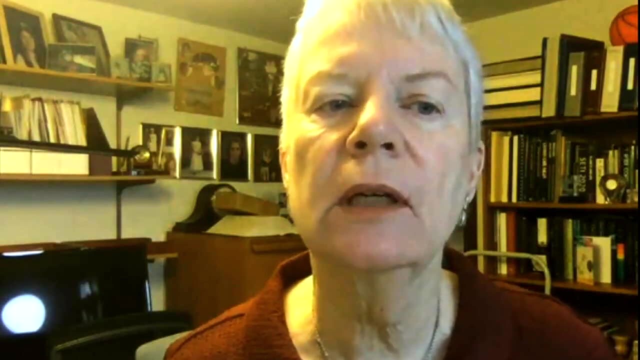 language, And so it kind of makes sense. you know the question: what happens if we write circularly? Are there people actively thinking about what language we're going to use? Yeah, that's a really interesting topic of interest for quite a while. 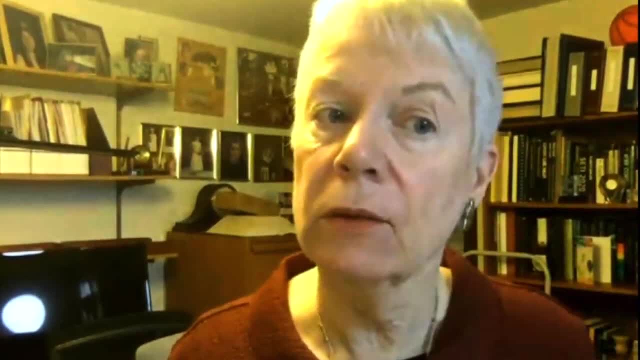 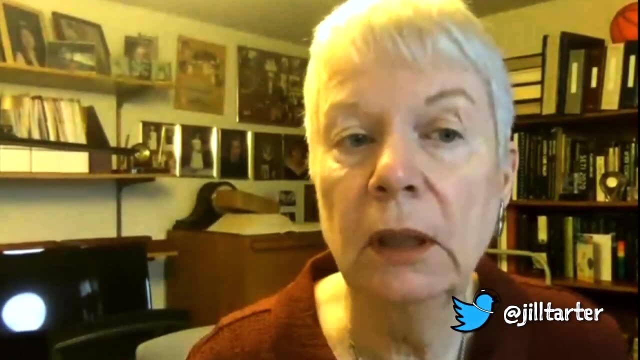 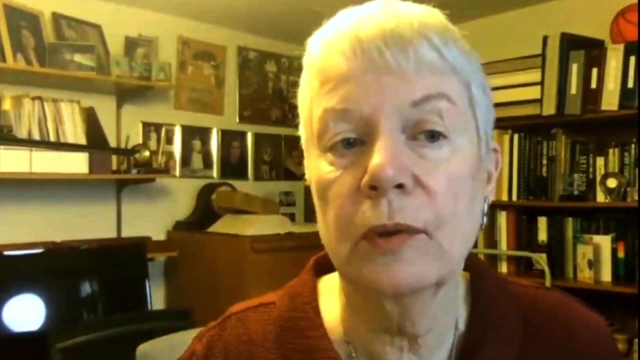 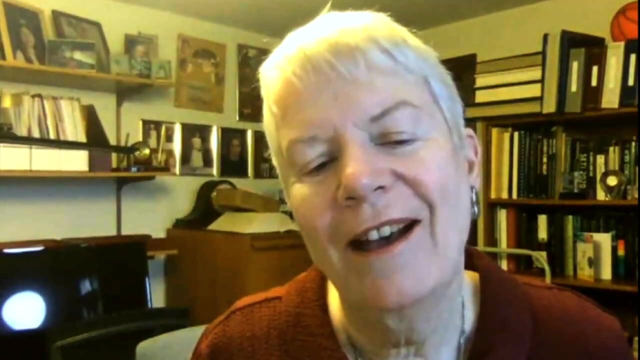 And at first I think the easy solution to that was: well, it will be based on mathematics, right, And certainly developed this whole language rules, sort of mathematical rules. But then I learned more about the brain, it seems to us now. 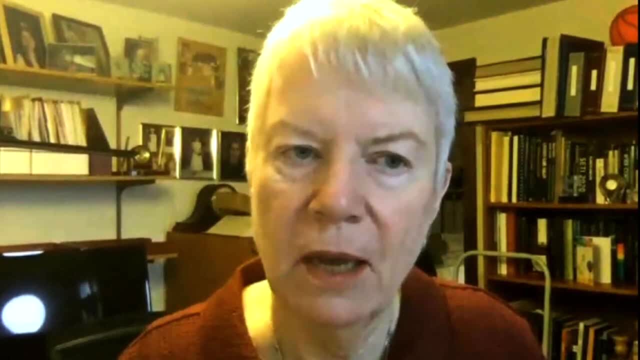 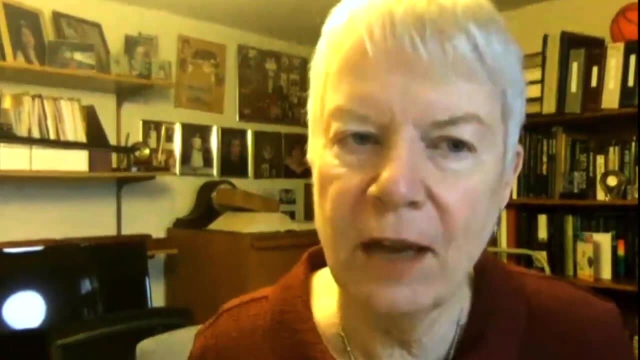 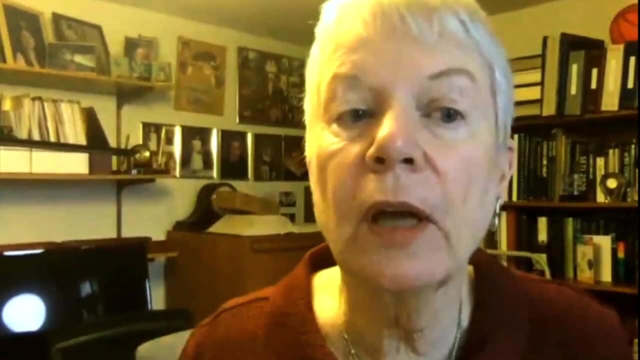 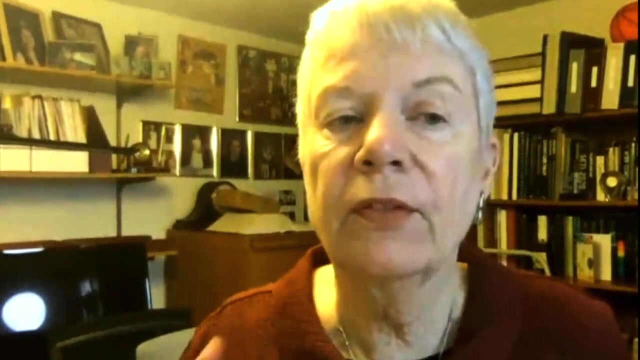 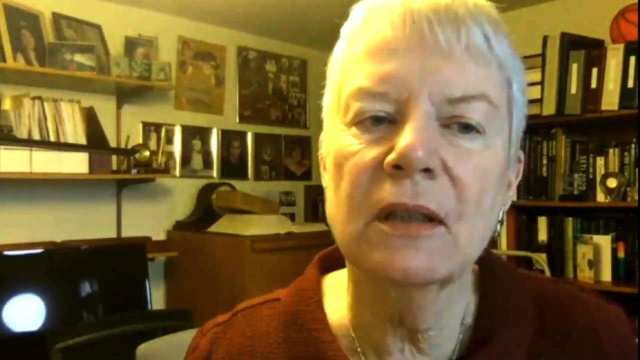 that the actual structure of our brain dictates how we think about mathematics. perhaps So we might be correct that something like the periodic or simple rules of addition, subtraction and that sort of thing, that they're all correct, But even to technological civilizations trying to 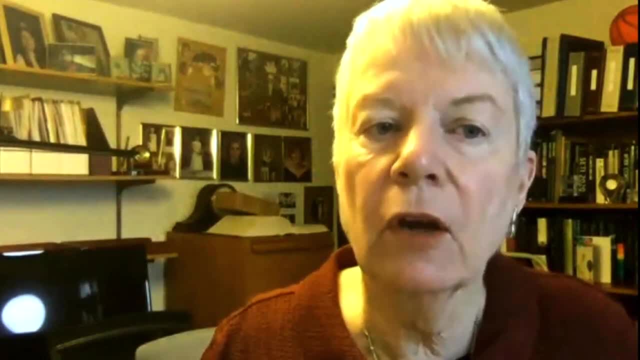 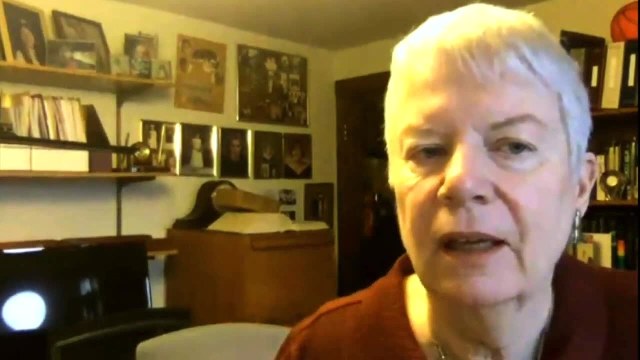 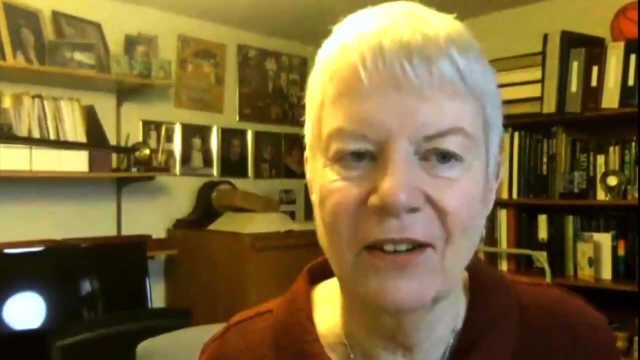 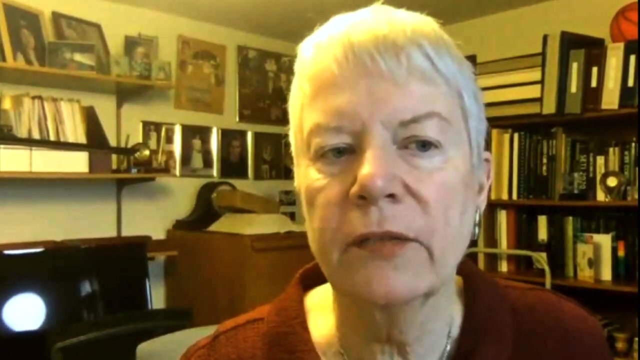 describe the same phenomenon using their intrinsic math. it might not look anything like the same thing. We're getting a bit. we're going beyond the back of the envelope in our thinking here, trying to understand what, if anything, is universal, what is? 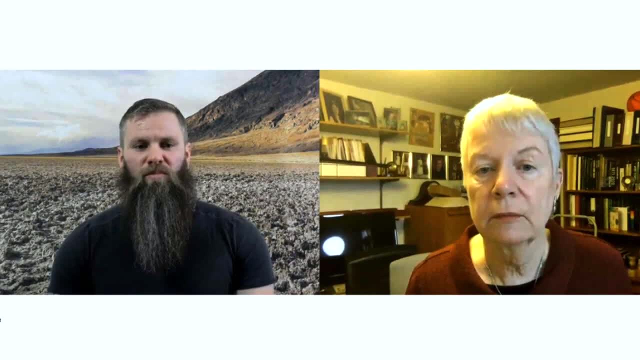 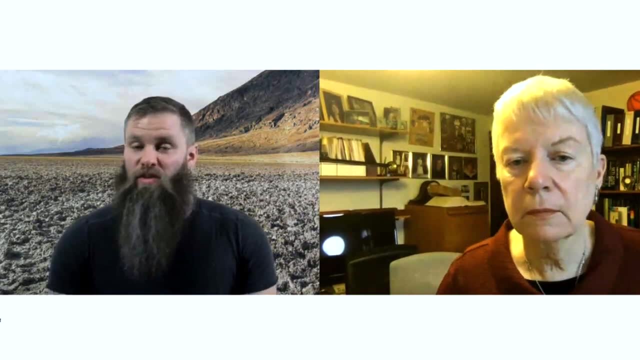 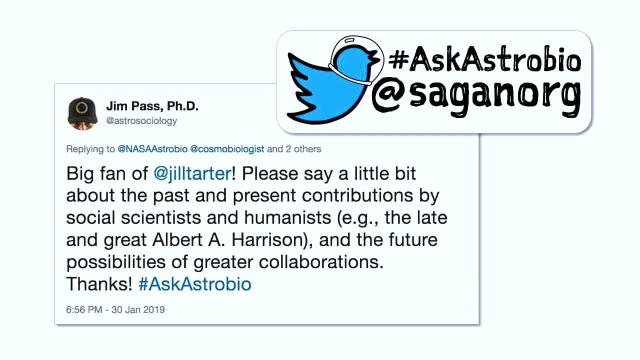 fundamental and what is contingent upon the fact that we have a three pound brain that is structured by the universe and the universe, and the universe and the universe. So we're going to have to think about the universe and the universe and the universe, and 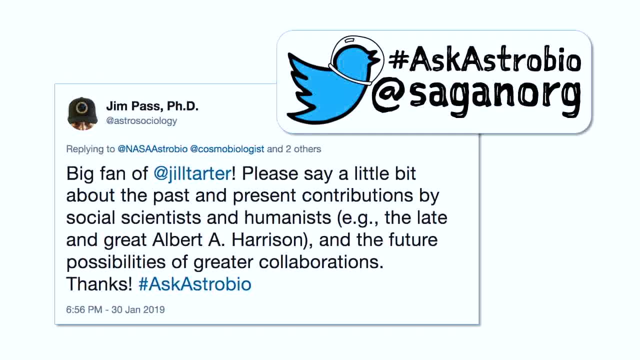 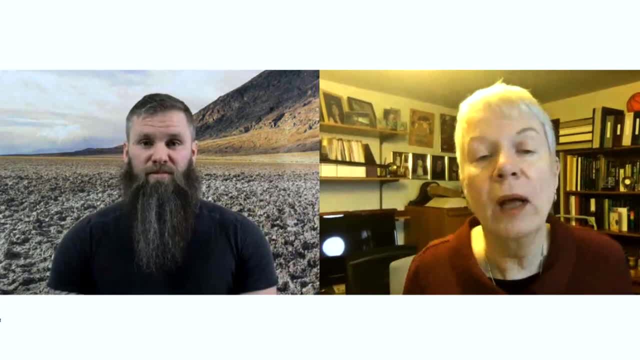 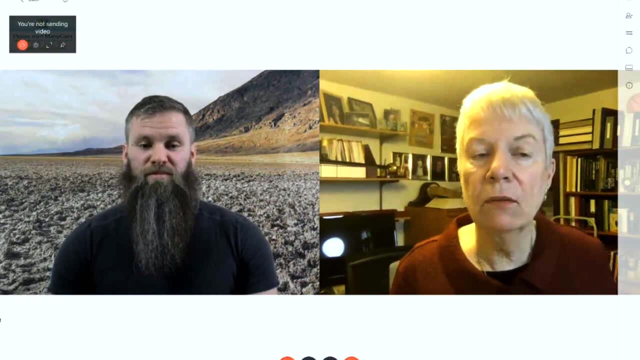 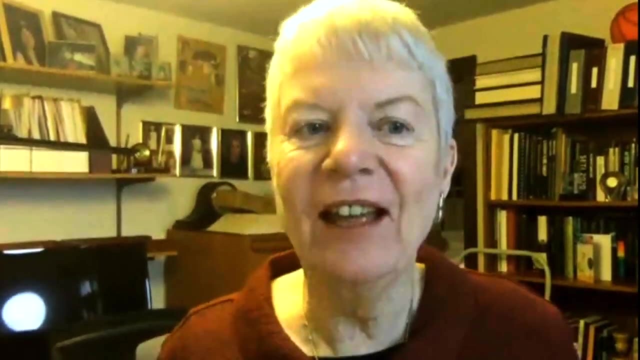 the sciences and things like astrobiology and SETI. He's right in the fact that in the past they haven't been included or not well included- Right to get smarter, and so now we are looking for opportunities to work with these other disciplines. It's 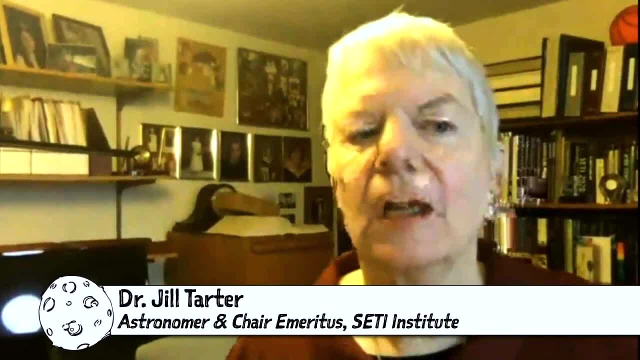 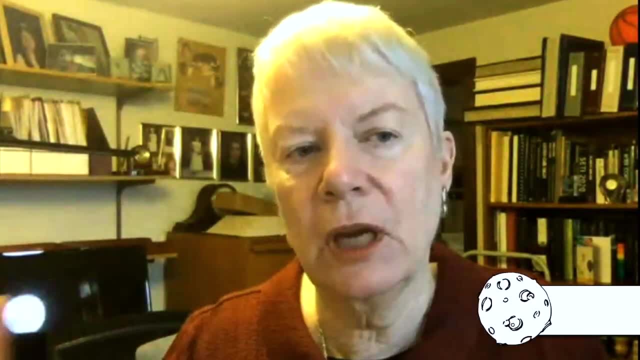 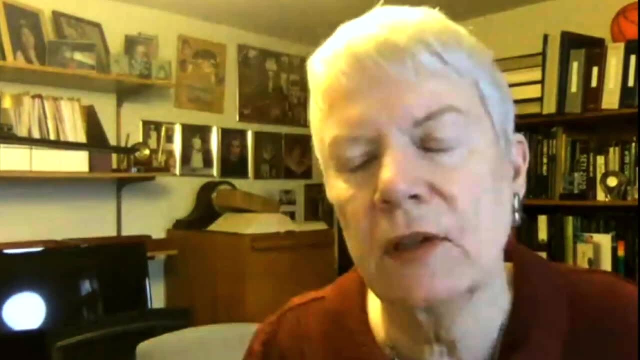 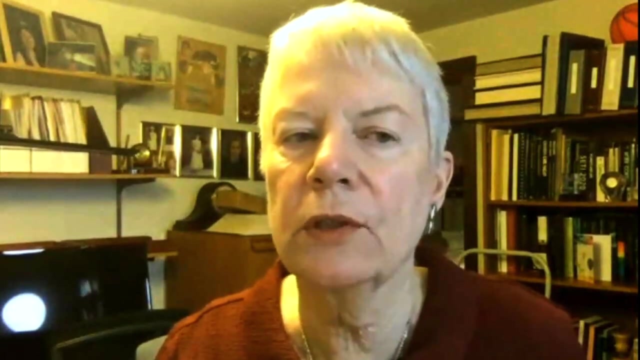 difficult. We all have our own, and it's more than just writing an astrobiology primer with a glossary to explain to a geologist what a chemist means. There's some more difference in the way that some of the social scientists and some of the 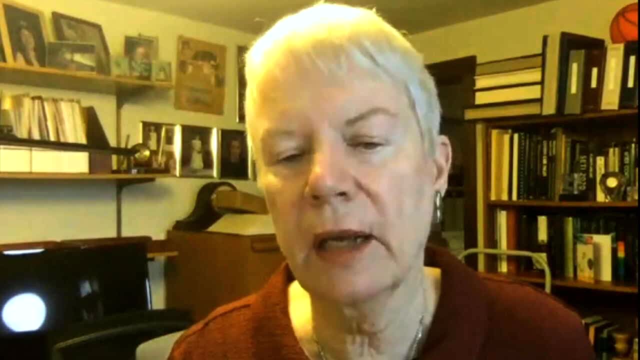 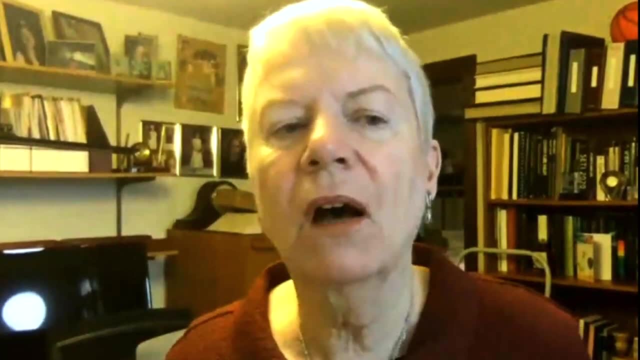 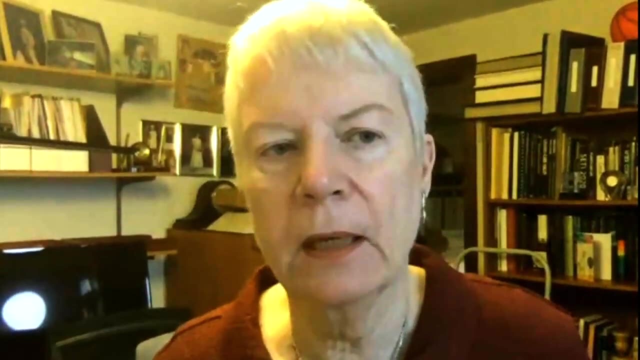 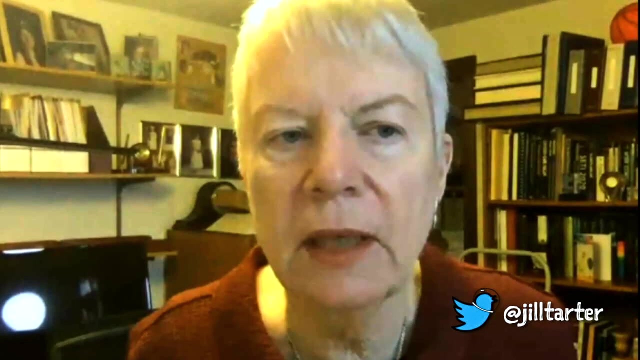 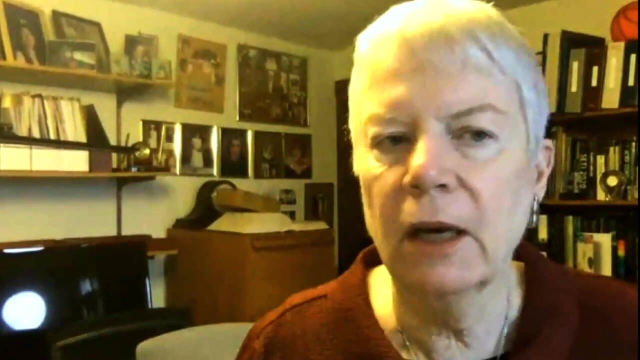 SETI scientists approach the world. For example, there's a terrible book decades ago called Chariots of the Gods, which was totally disrespectful to civilizations from millennia ago, because he said: oh, you couldn't have done this or built this or created this unless there was. 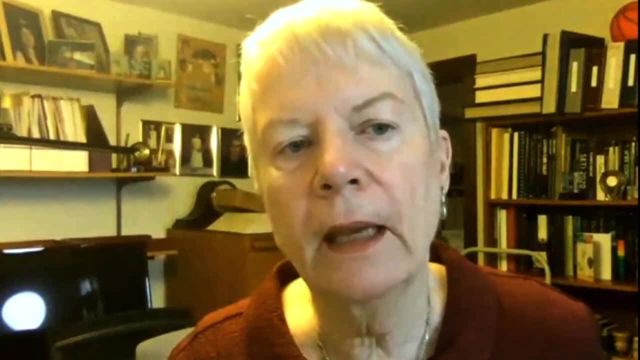 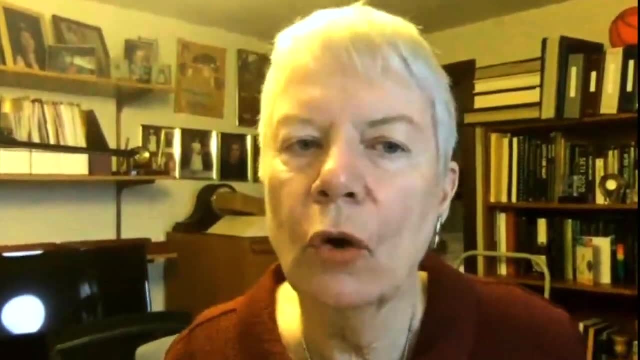 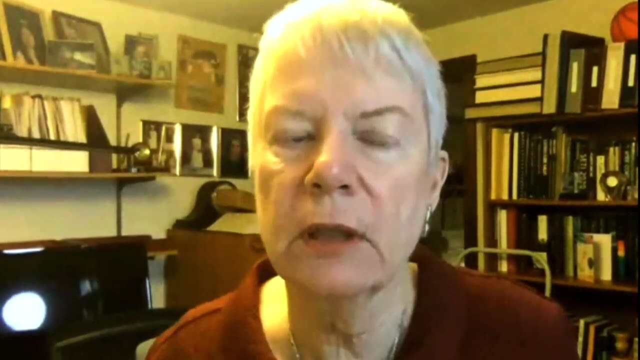 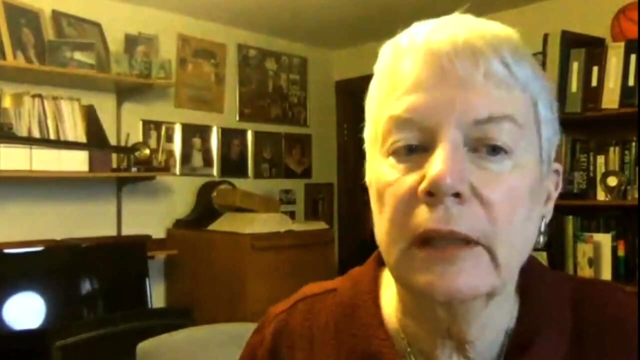 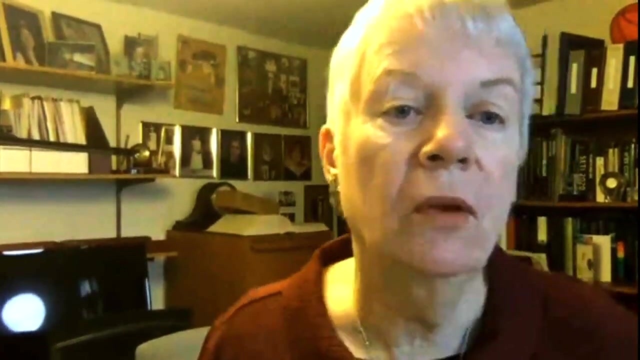 some other way to do it. So I think it's really powerful to those civilizations and as a very, very first step, it really makes sense to go back with folks that are trained in techno signatures, Who knows I mean. unfortunately, the whole thing has a bad 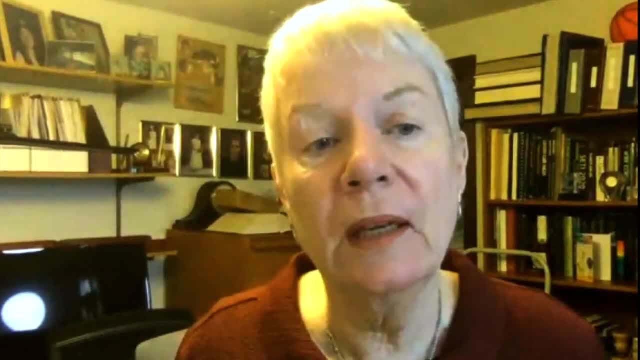 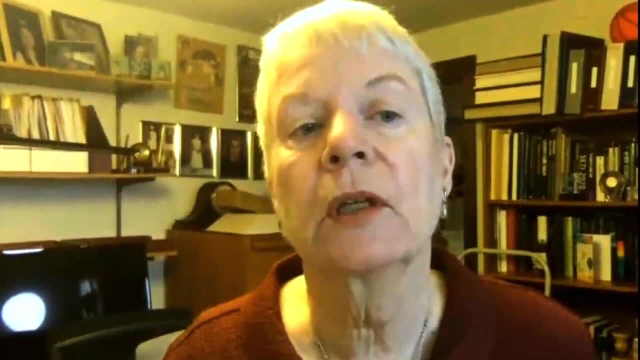 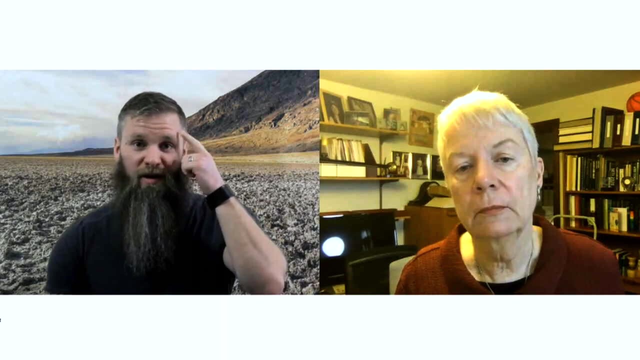 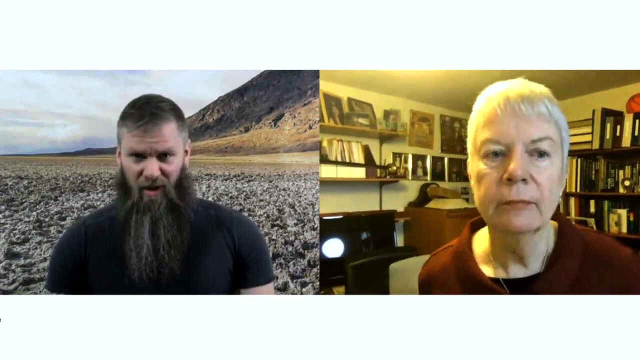 taste because of how poorly it was done with Chariots of the Gods, but it is a project that could be well done by cooperating with experts in those fields. Absolutely The inherent racism and culturalism involved in that. so I'm glad you brought that up. 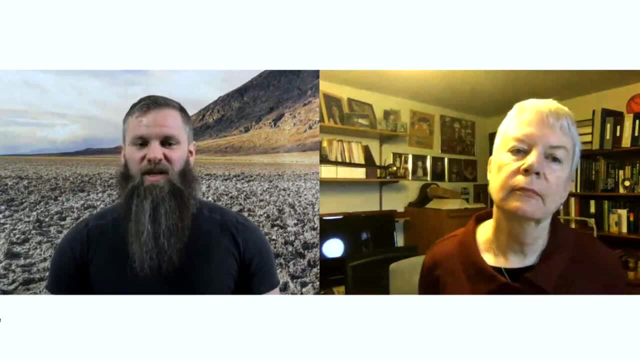 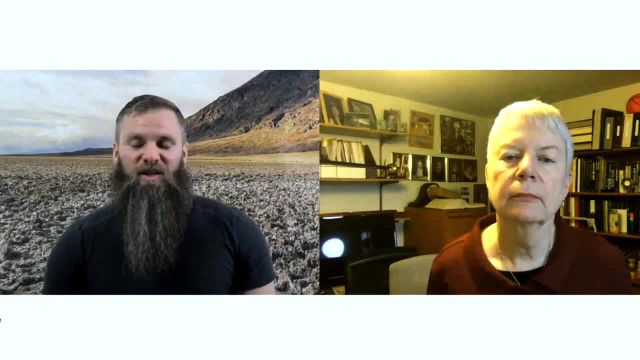 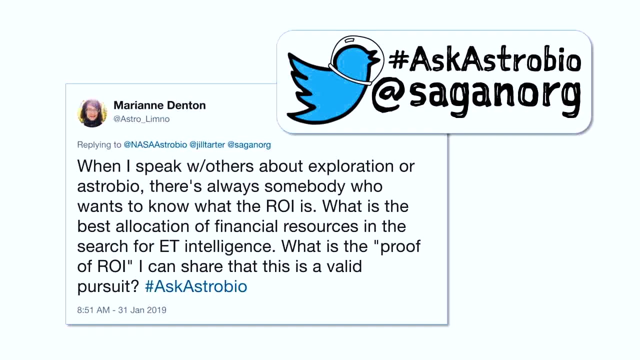 We have another question, and this one kind of often comes to lots of us in the realm of astrobiology and even space science in general, when people say: you know why go spend money on going to space and what the investment is. So her question is: 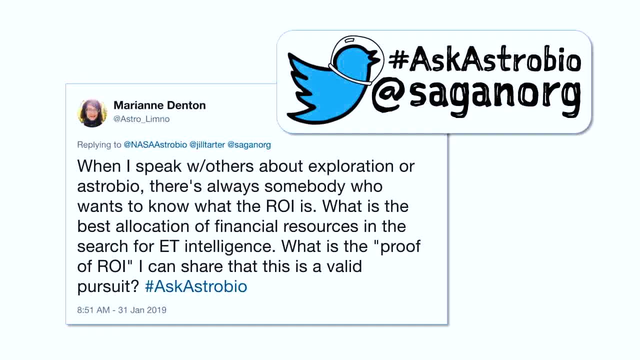 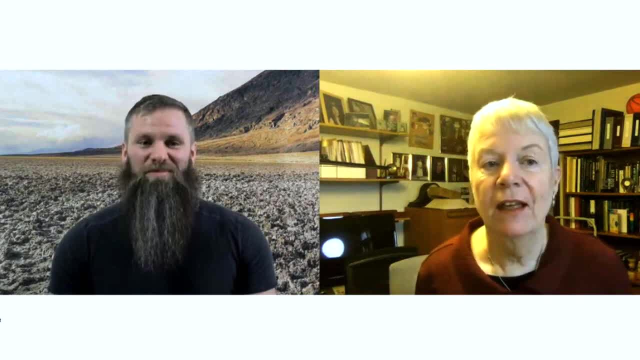 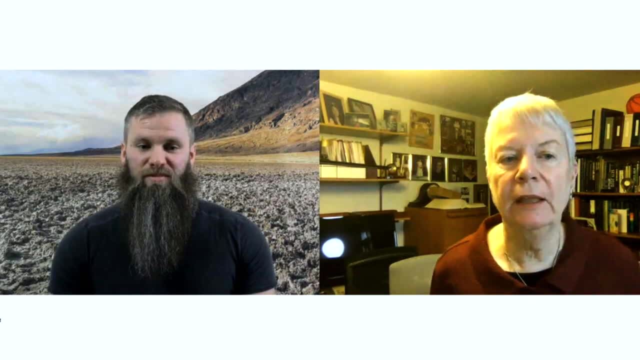 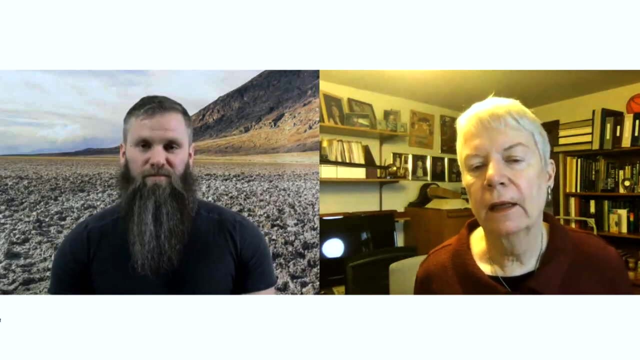 how can I best share that this is a valid pursuit, and I assume by this she means how is SETI a valid pursuit? Okay, I've got a really simple answer for her, which is that SETI may turn out to be absolutely not a good. 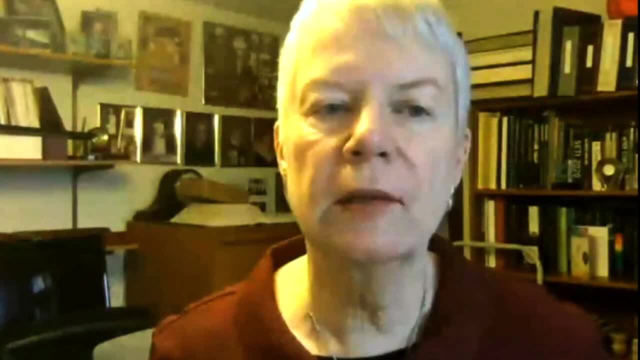 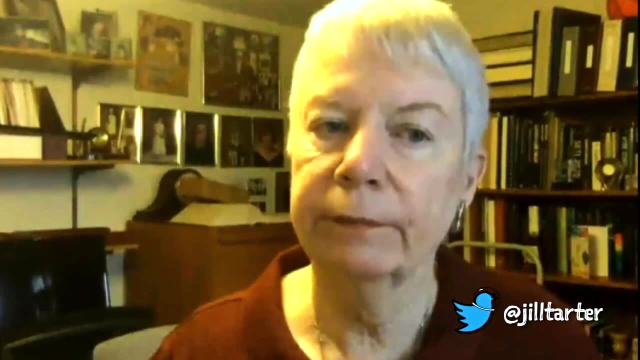 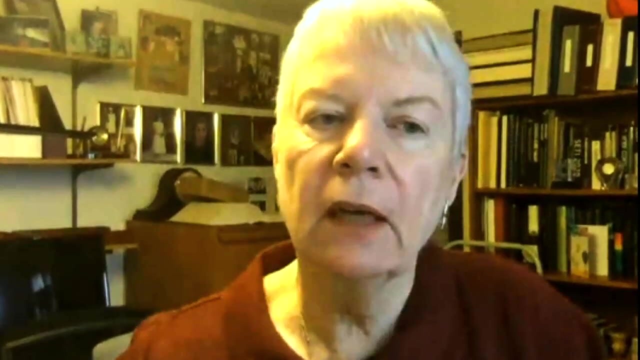 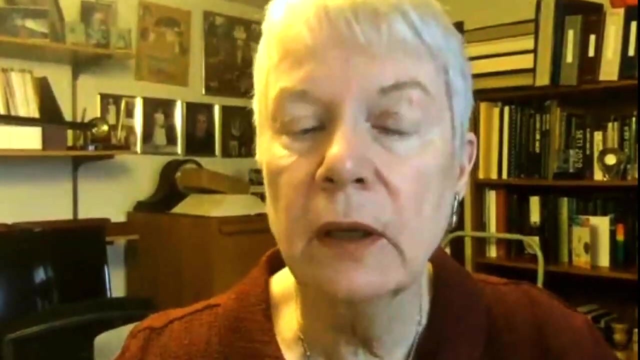 answer. It's a statistical answer, so sometimes it does not please questioners, but it's the deal. If there are any two technological civilizations that are capable of contacting one another and we succeed in that contact, it means that that other civilization has to be close by. 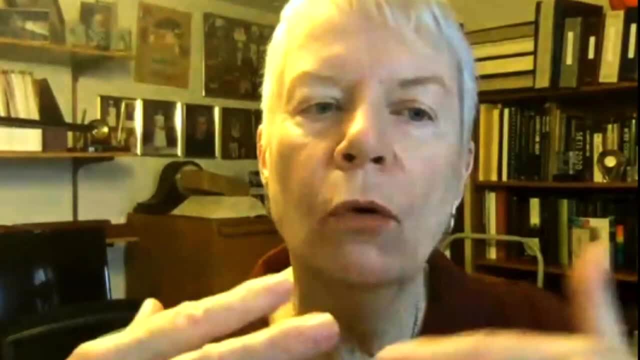 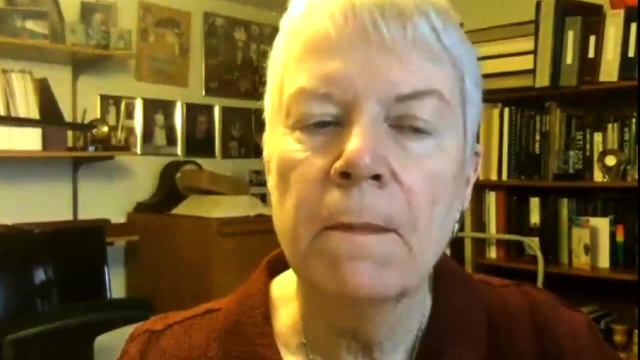 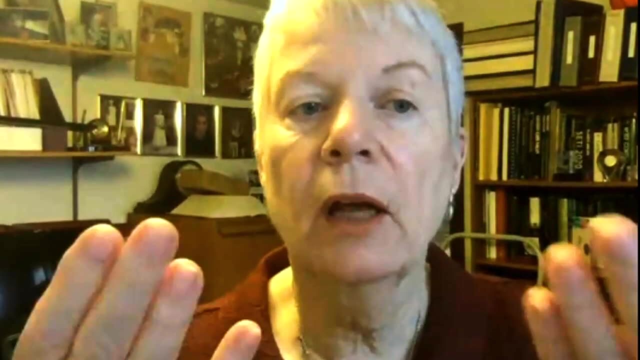 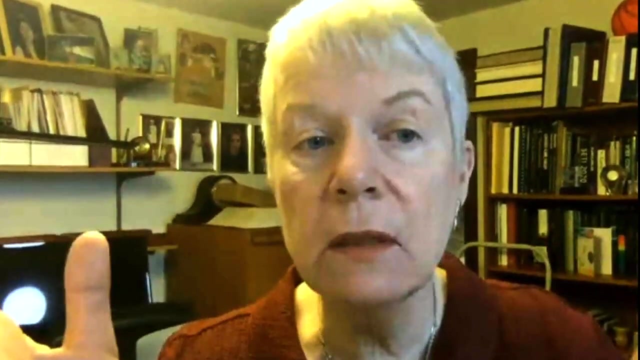 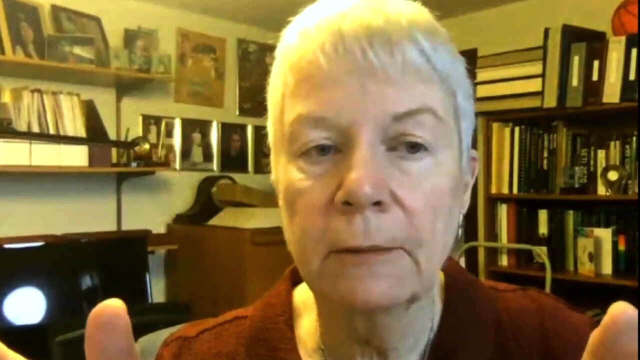 Close in time. We have to be overlapping in this 10 billion year history of our galaxy. And if technological civilizations as a rule start up, grow up, expand and either turn themselves off or do themselves, there will never be a successful contact. But turn that around. 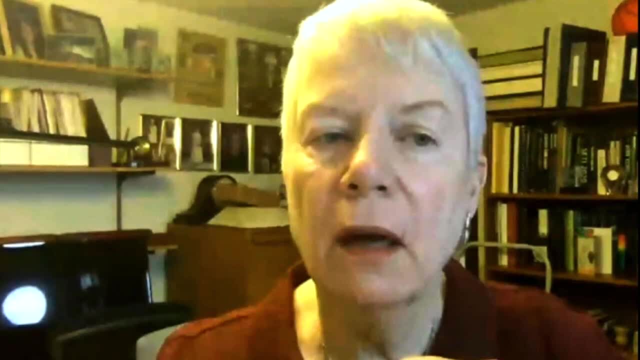 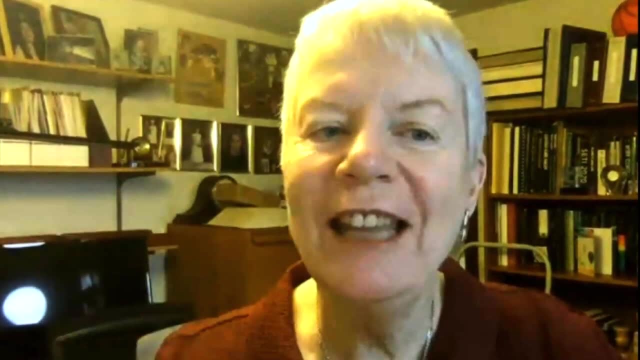 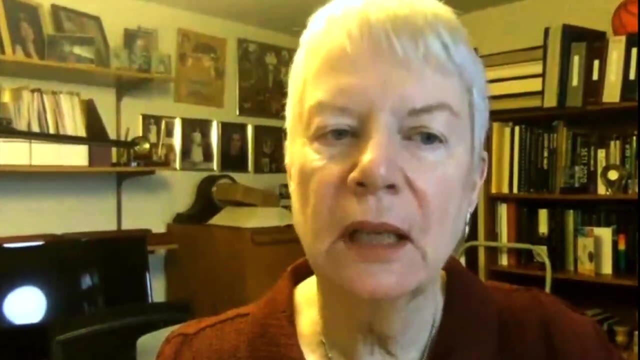 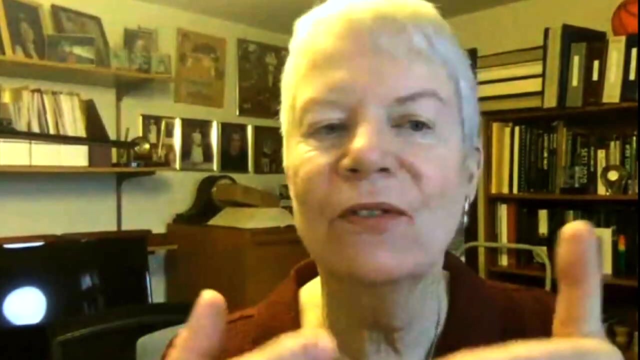 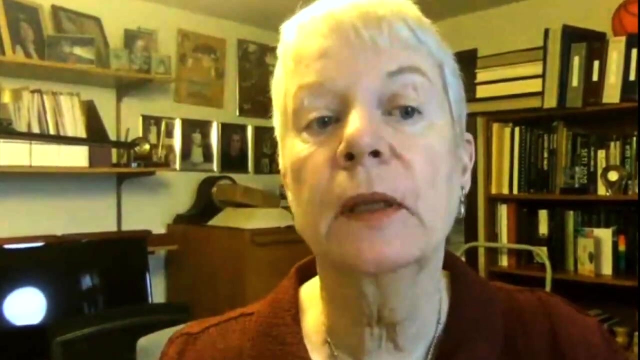 If we succeed with setting, we know that, on average, technological civilizations must be long lived. Somebody else has figured out how to do it, How to have a sustainable technological civilization in hundreds of thousands, millions of years, Something that we don't necessarily see as a. 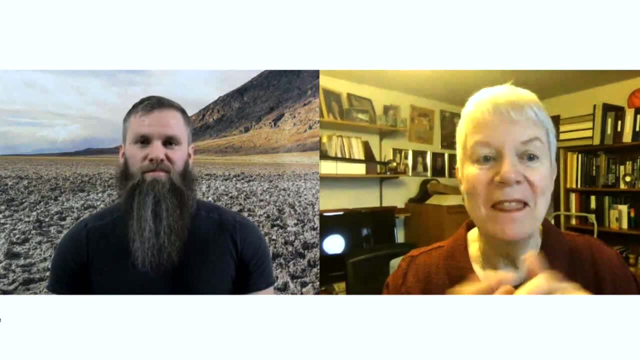 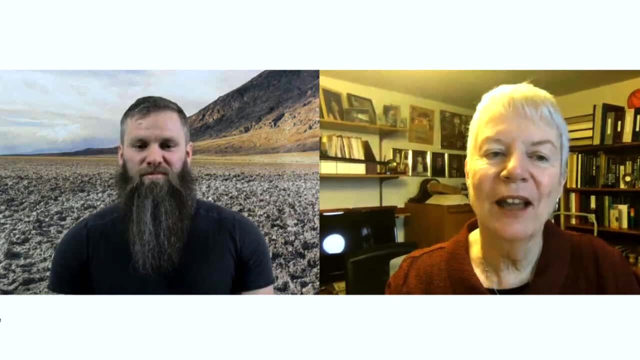 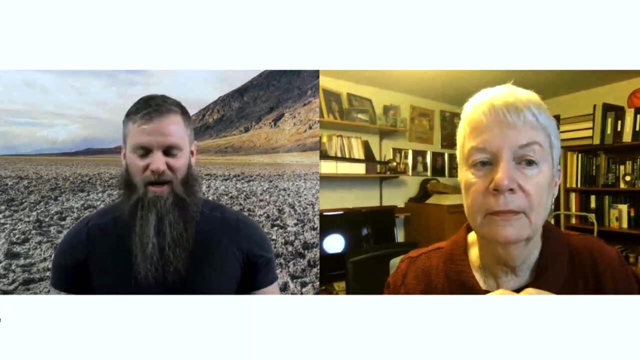 possibility for us today. We see lots of ways it could go wrong. But even a cosmic dial tone, no information, but just proof of existence that we can try and get our act together and figure out how to get there. Yeah, absolutely, And it seems. 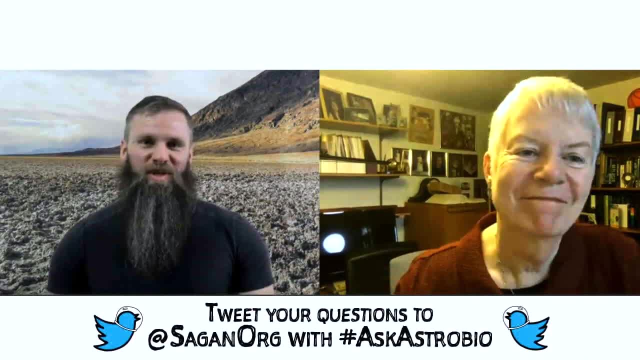 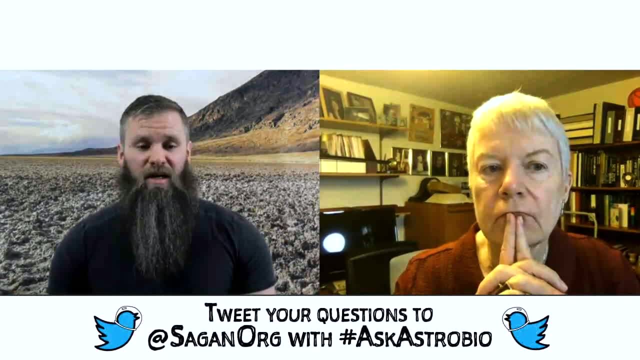 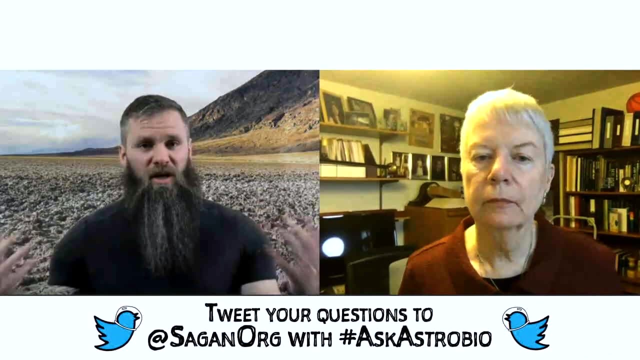 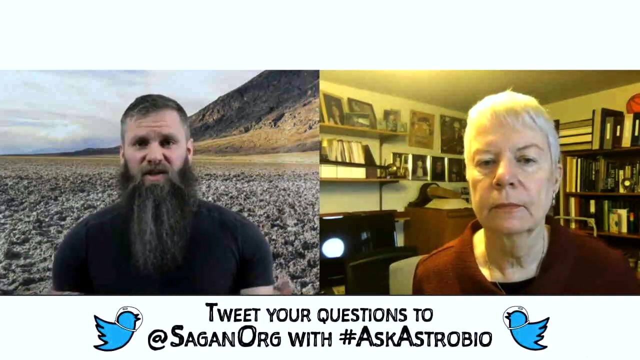 like, even though right now, I think so many of us, we tend to focus so much on the bad things sometimes going on around the world. We see war and we see the world changing. We see the world changing. We see the world changing, So we 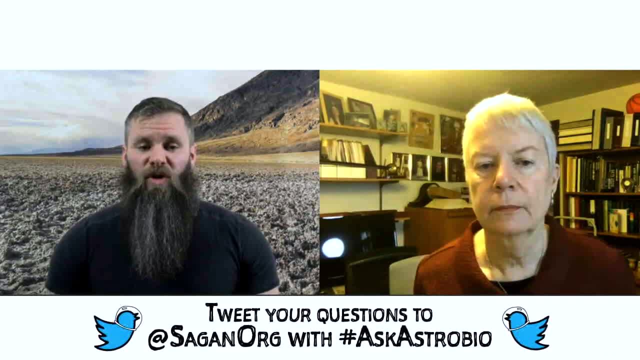 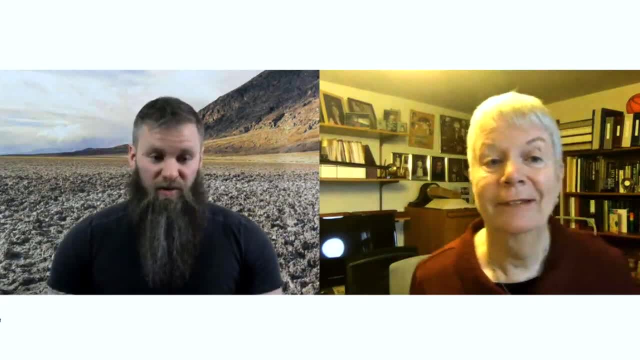 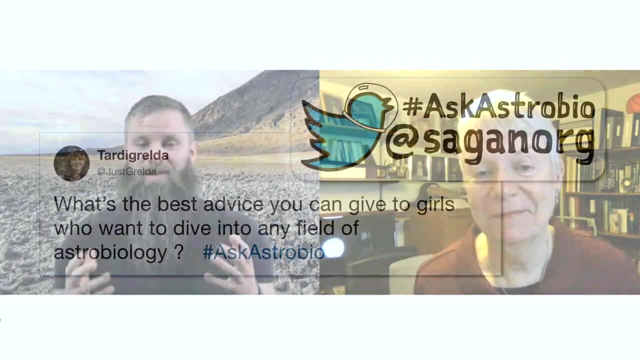 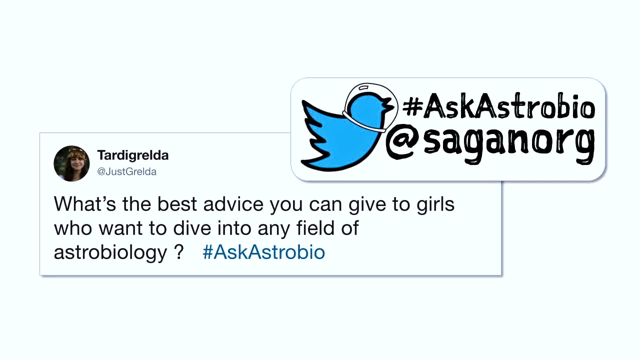 see the world changing. And we see the world changing And I think that's the most important thing that we can do, And I think that's one of the most important things that we can do to help people who want to dive into any field. 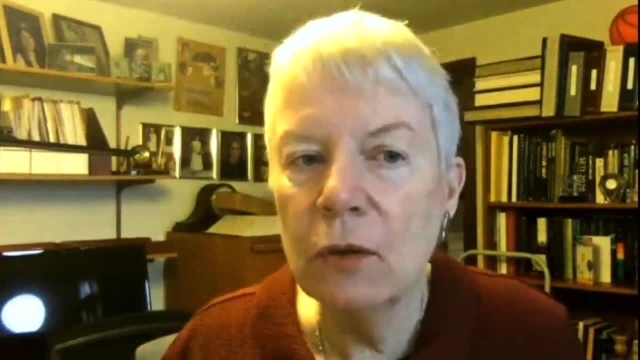 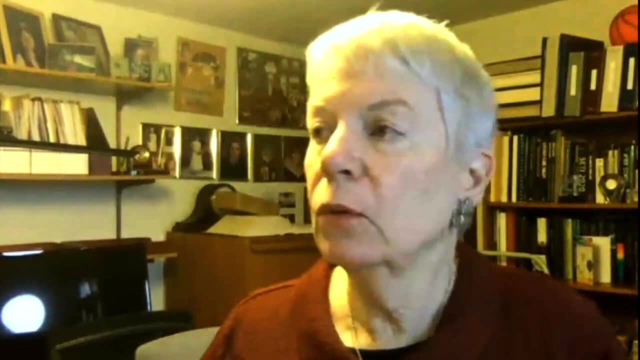 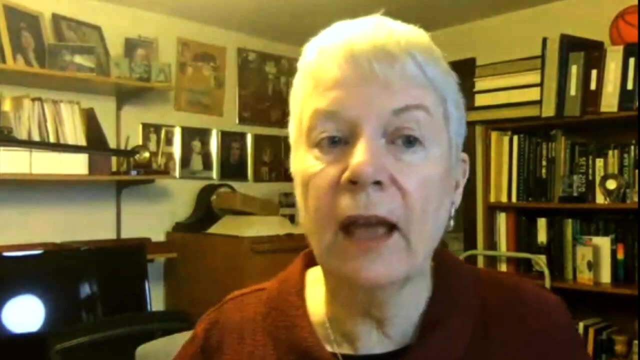 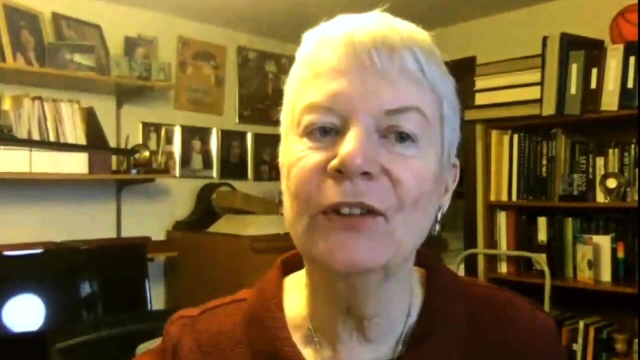 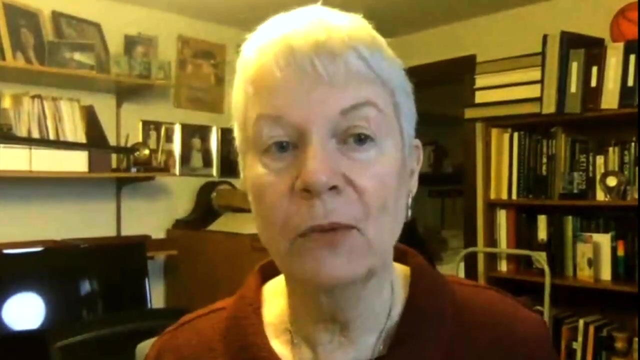 of astrobiology right now. Find out what you really love to do And then learn how to use some tools. you can essentially um drive your own boat right, so have skills. we'll travel. let's find the interesting problems, and you won't be able to solve them without me, so i want on board and you'll. 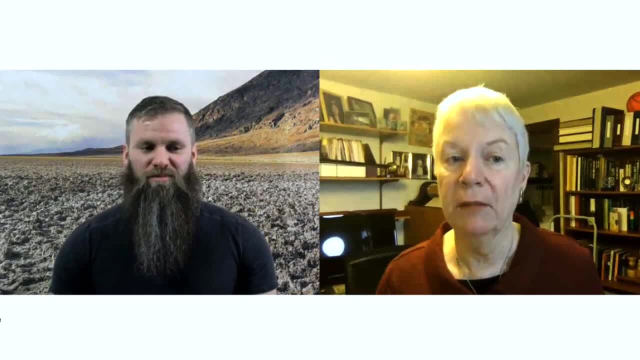 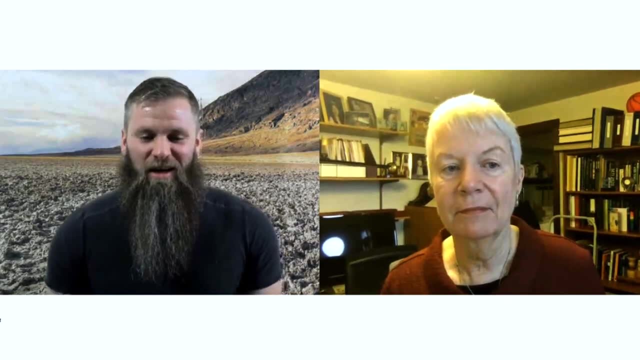 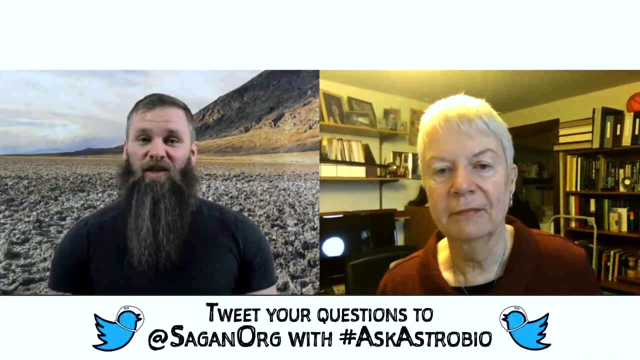 you'll turn out to be much better served by including me, absolutely, yeah, that applies to so many people who want to get involved in these things as well. um, i do remind our audience. uh, you can always tweet your question using using hashtag ask astrobio on twitter. uh, you can also ask. 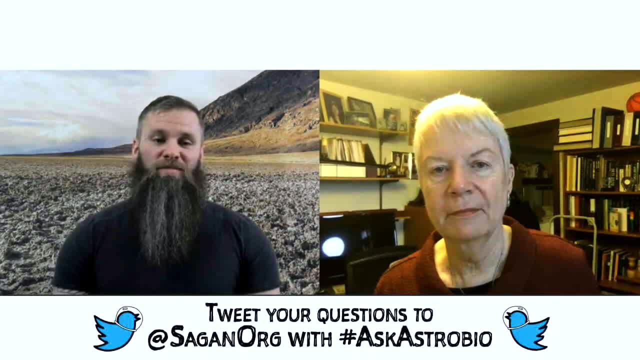 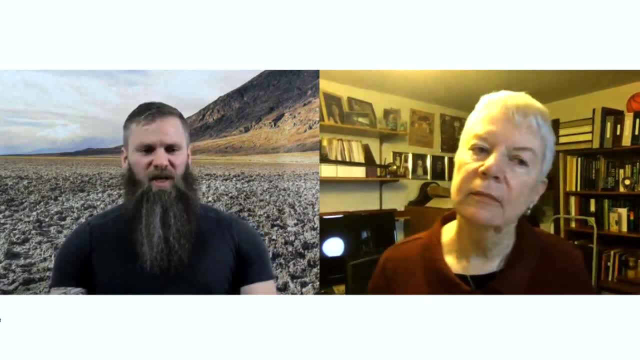 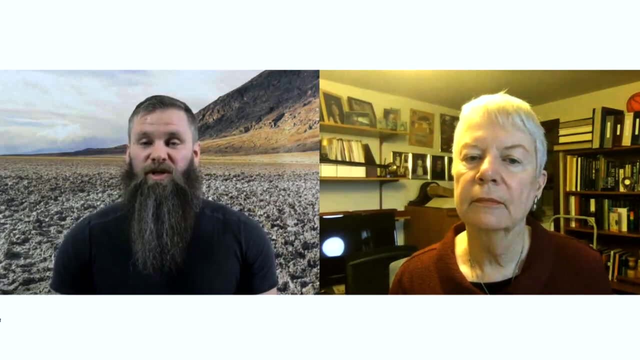 questions on facebook and on segan net. um, so our next question actually comes from facebook now, uh, from tom caruso. uh, tom wants to know. um he says: can you please tell us what you think about listening for life deep in remote ocean worlds um possibly using like seismometers and hydrophones? 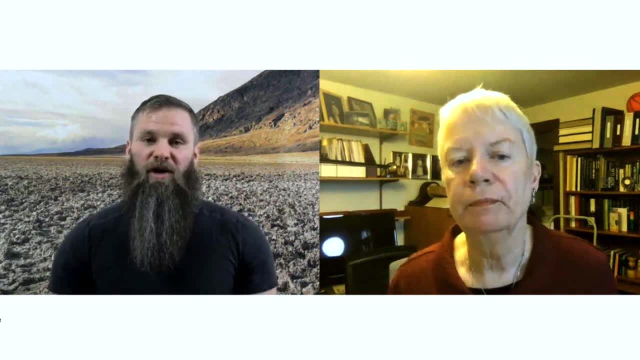 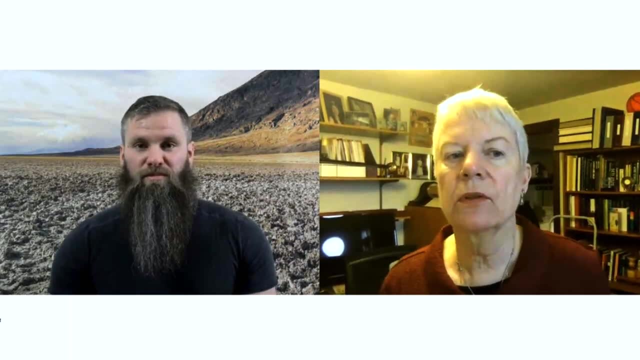 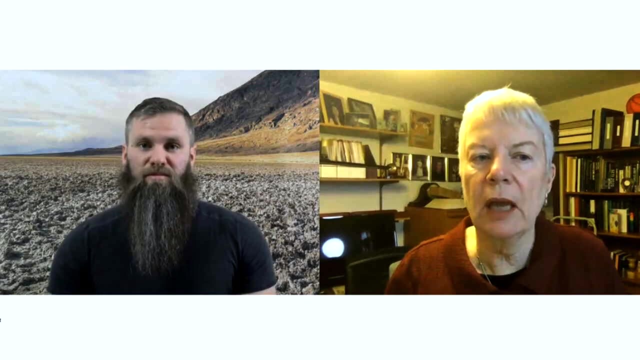 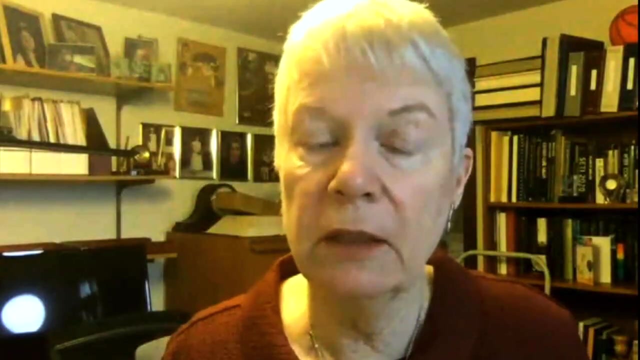 um, so kind of like doing steady but looking downwards inside of worlds. right, so we use those deep hydrophones to study humpback whales, to try and understand their social engineering as they recruit members to cooperate in bubble netting members who aren't relatives as it turns out. um, that's the technology we're beginning to. 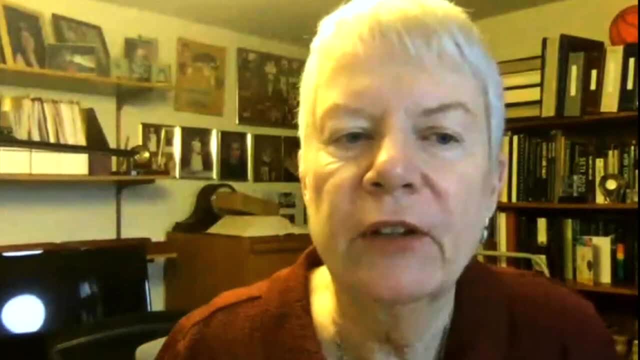 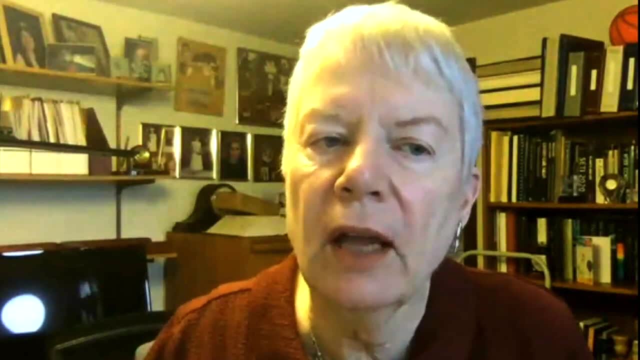 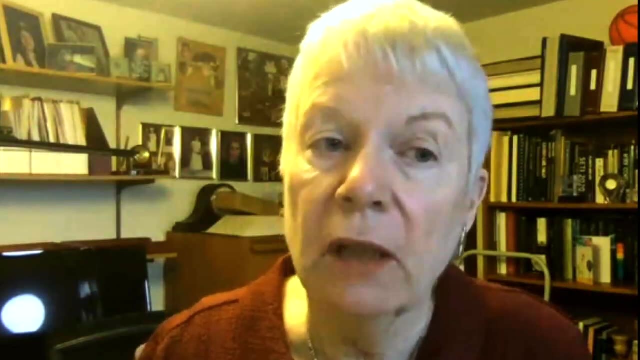 understand. we also know that when you're trying to figure this all out, it helps you to understand what's going on and it helps us if you have video as well as the audio, so that you can see their actions and tie them to the audio sounds that you're recording. that's going to be a challenge. 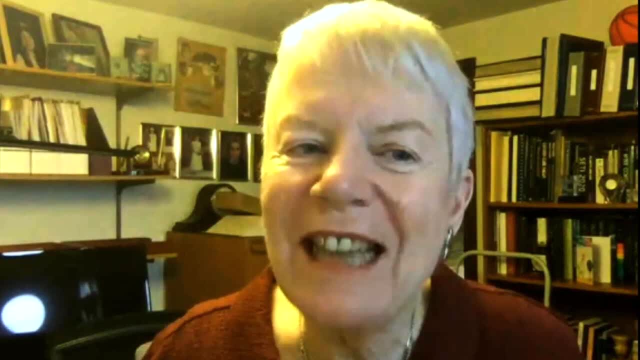 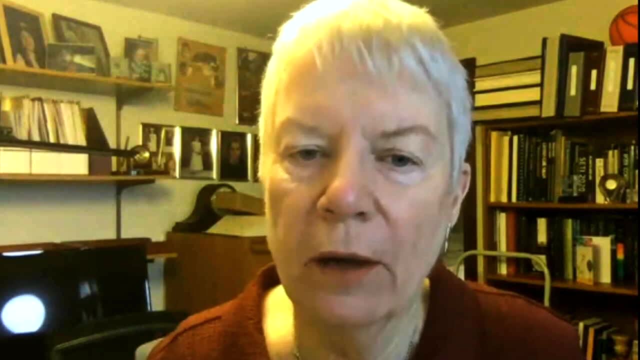 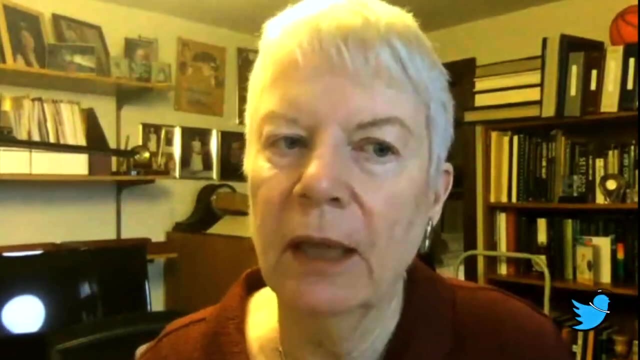 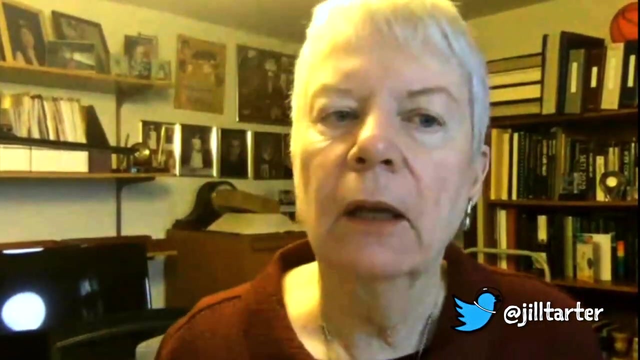 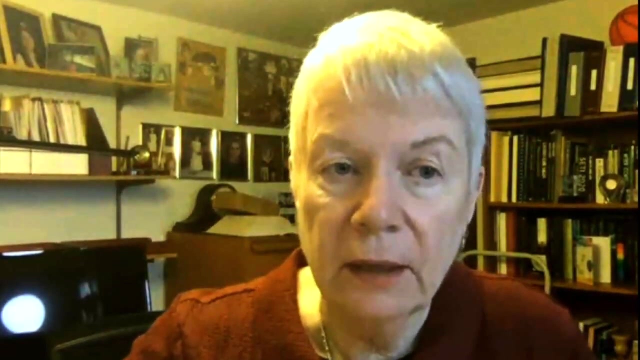 for off-world. um, what size creature uh gets to vocalize at depth in water? probably microbes aren't really very chatty, at least in terms of oral kinds of communication. large structures like the humpback who understand the structure of the ocean and can go and find the the level in the thermocline. 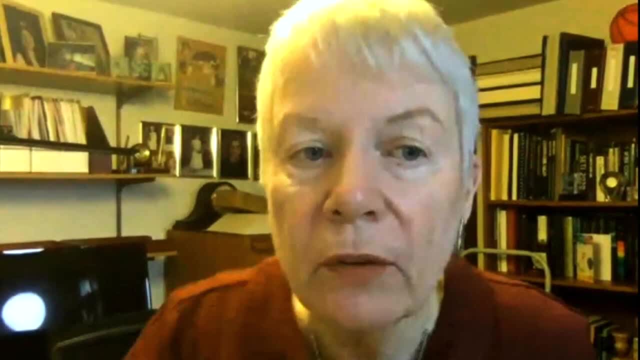 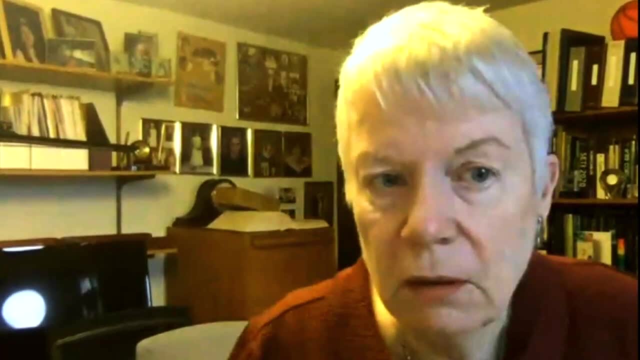 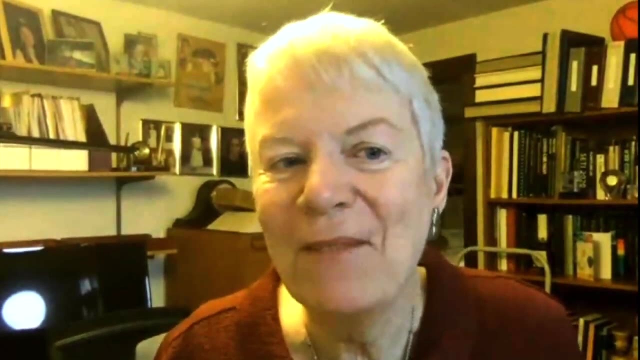 that will allow their songs and their messages to travel the longest distance. such very large creatures, um, are well suited to that kind of communication, so i think it's important to that kind of communication in a, in a liquid world, um, i don't know. i'm i'm very, very eager to see how. 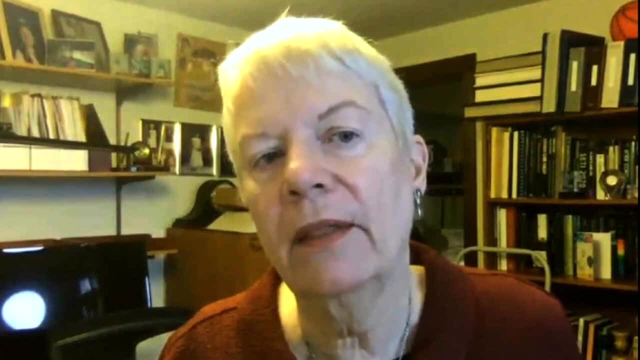 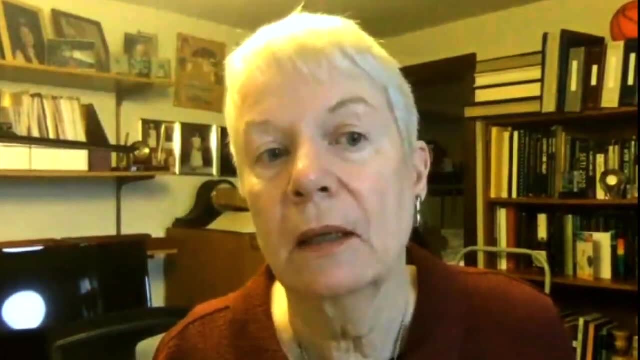 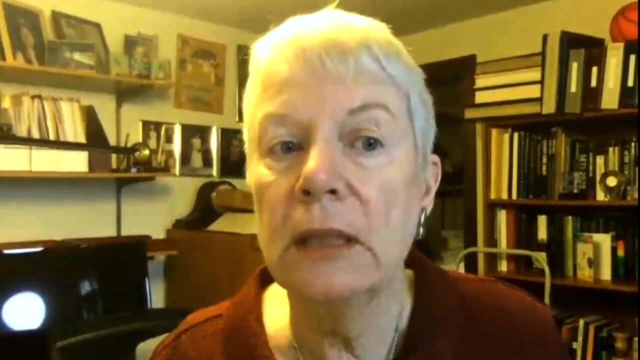 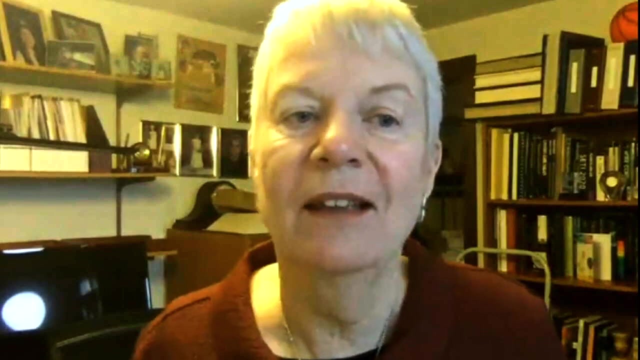 we solve the problem of sampling the ocean worlds within our own solar system, um, what can we do with plumes and how can we concentrate what it is that we collect and how can we avoid contamination the material that we are trying to collect, as we, if we have to melt through or drill through kilometers of ice to get there? 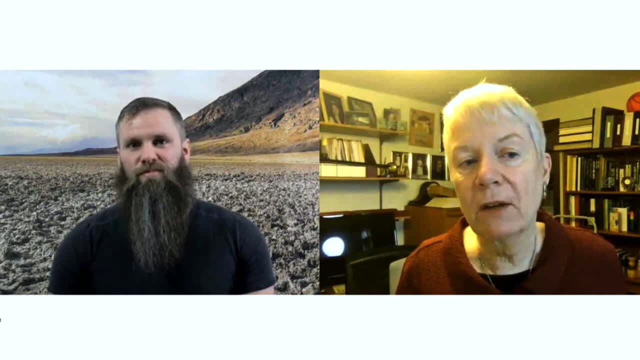 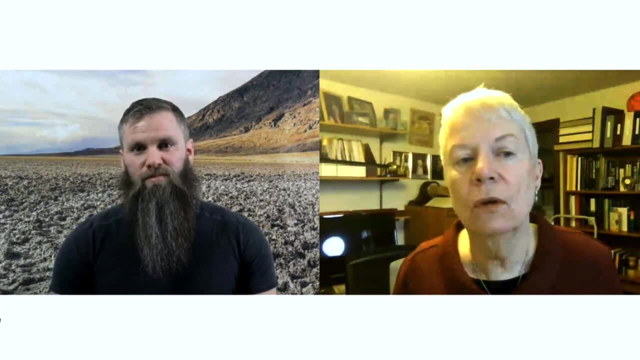 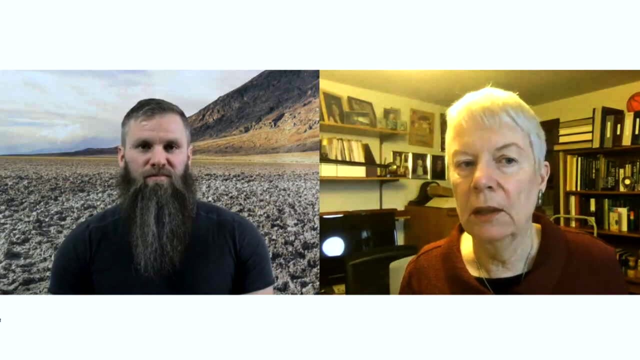 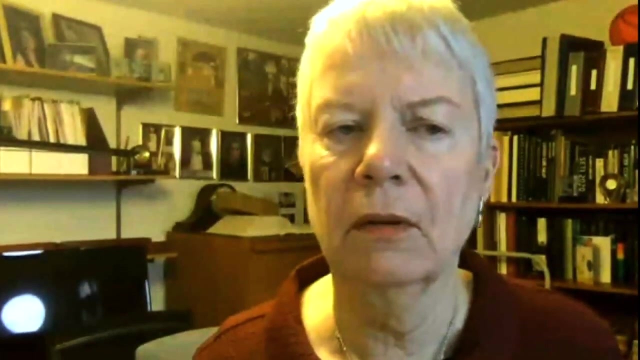 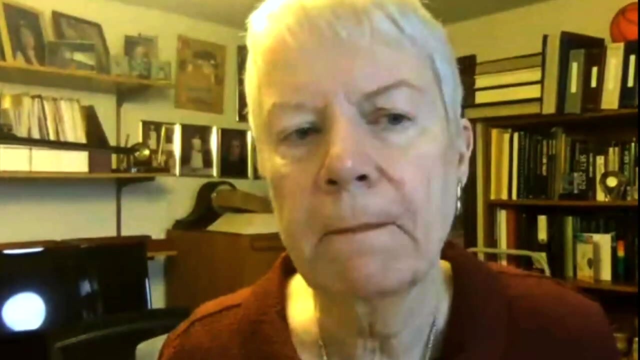 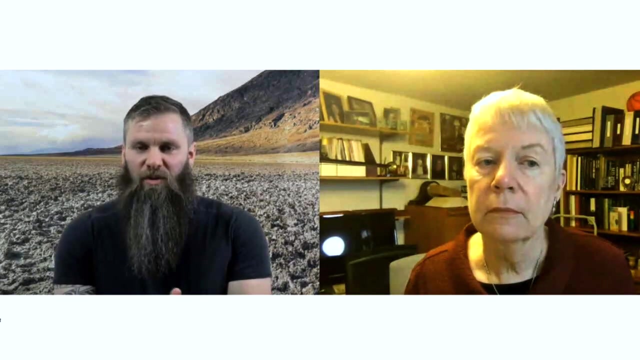 all fascinating questions, i think. thought um, if you're really going to tie it to intelligent communication, i think you're going to need some visual cues as well. well, some structure, um, um, um, um, vents, creaking and stretching and and contorting- interesting, yeah, um, since you brought up this idea of contamination, um, i do wonder what you 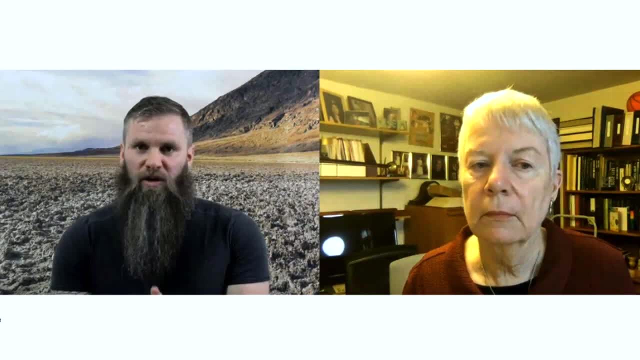 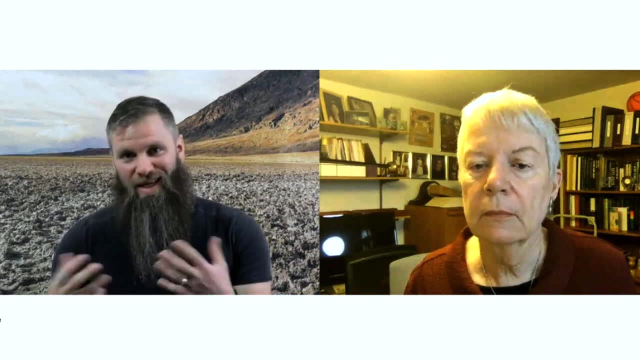 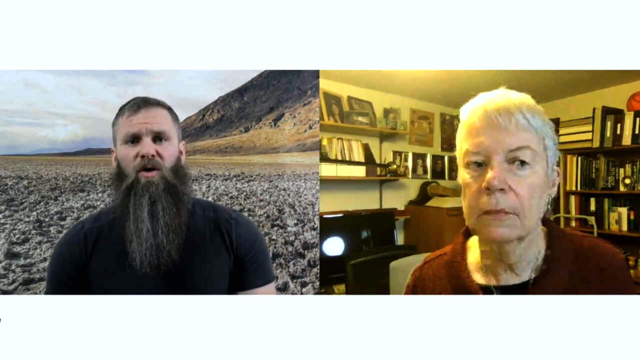 think of planetary protection? um, right now, when we launch missions through nasa? um, we have a planetary protection officer. their job is to try to make sure that we're being as clean as possible our spacecraft. we're also weary of bringing potential alien life back to earth. um what do you? 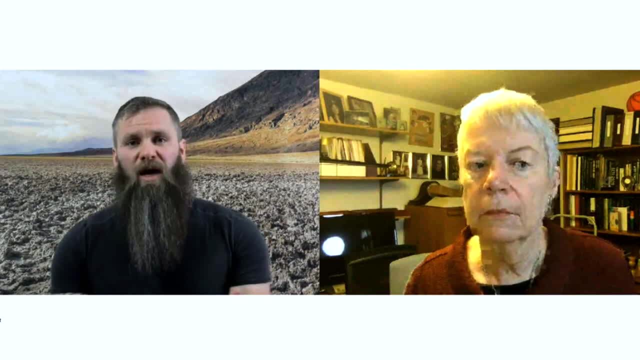 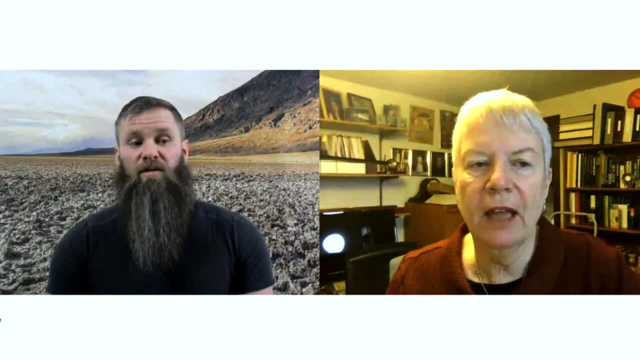 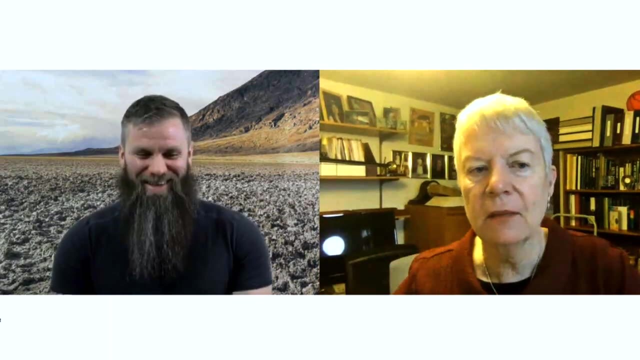 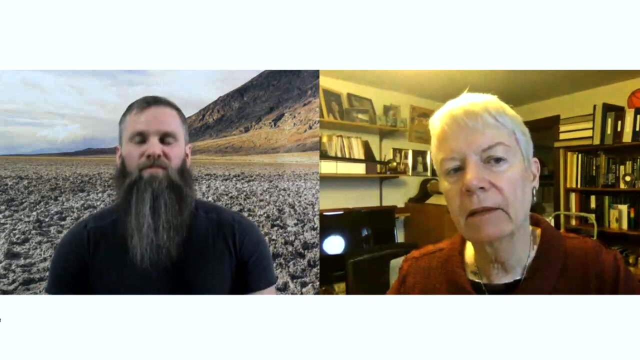 think about planetary protection, um, and then including that in our mission designs. okay, graham, i lost all of that. after what do i think about planetary protection and i vote for it. yes, okay, extremely thoughtful about how we do our research. we're only going to get, in most cases, one chance, and it would be 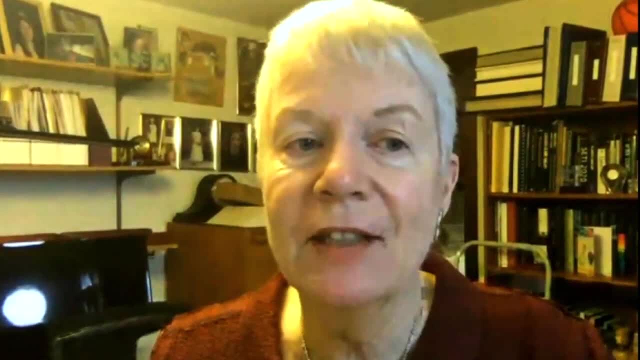 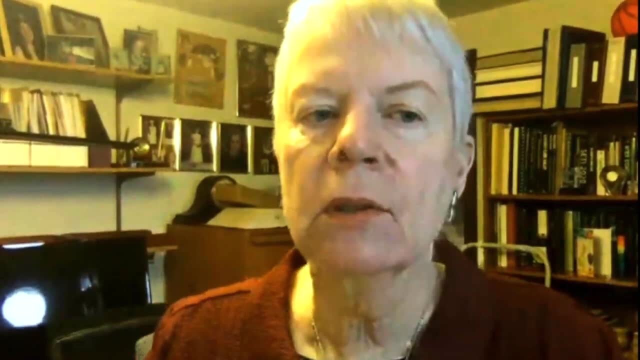 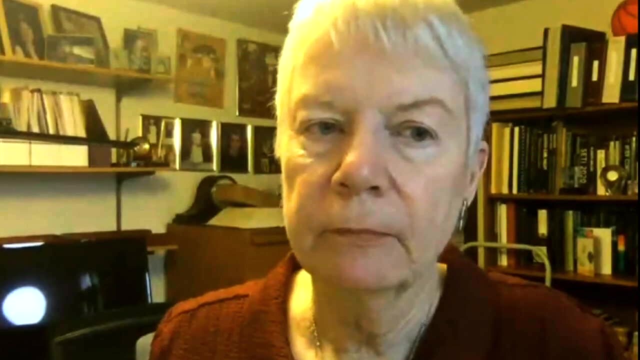 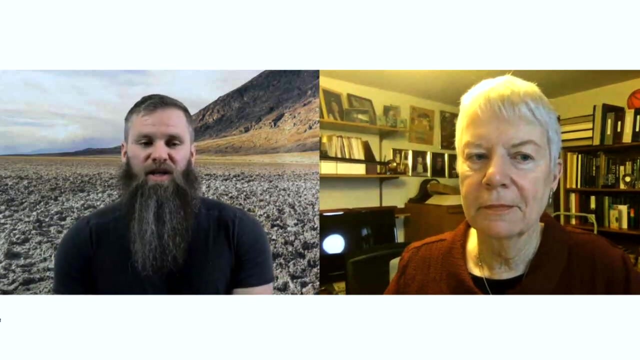 um, really disappointing if we didn't do our exploration in the most appropriate way so that we don't end up with ambiguous results. okay, awesome. um. our next question comes from the user jc on twitter. uh, jc says: is there any��? i think this is a very good question. um, i think about you know, SAMYETTE has a lot of work done here in the industry. i think about these here on the ground. a lot of work is being done here in the 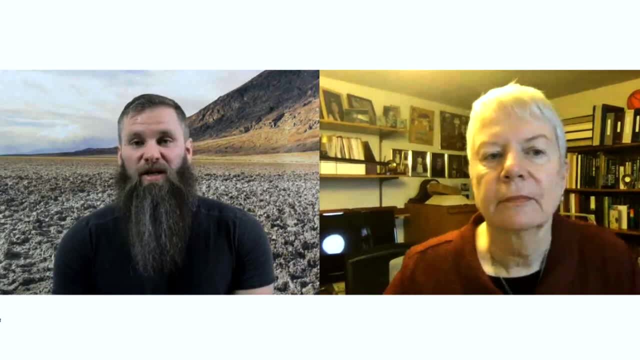 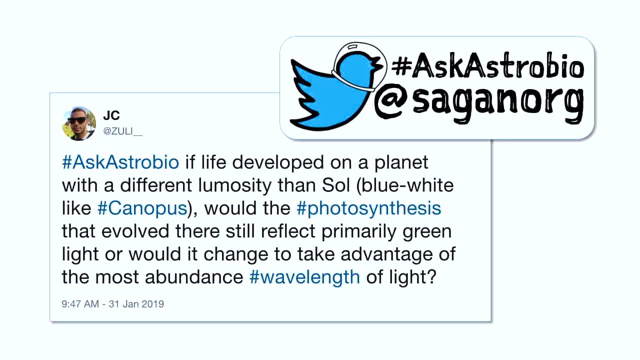 JC says, if life developed on a planet orbiting a star with a different luminosity than our sun, do you think photosynthesis that may evolve there will still reflect primarily green light, or would we see a change in what they're using, taking advantage of the most abundant wavelengths of light? 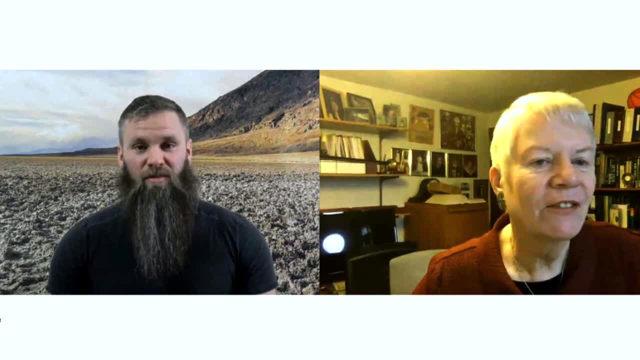 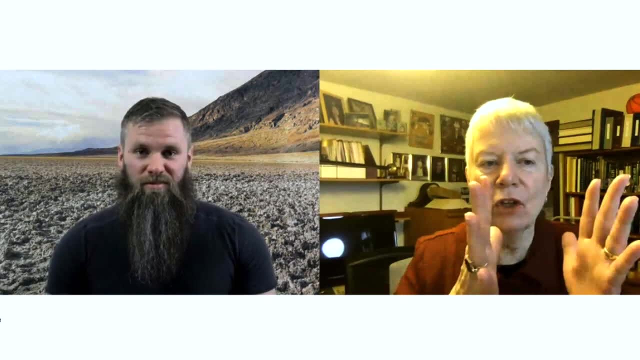 Yeah, you mentioned something earlier which leads me to believe, I think, the fact that we do this, the fact that astrobiology is a young science and wasn't a science that was all stovepiped and stumped up with, excuse me, old white males. 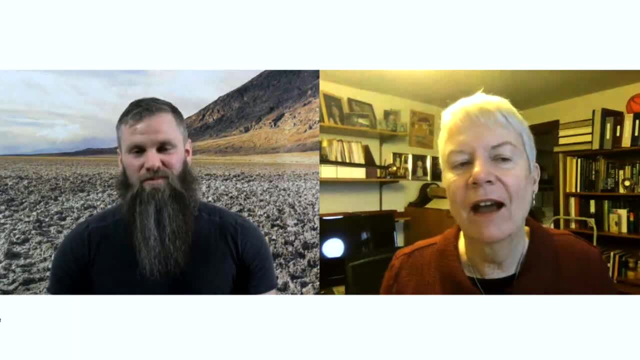 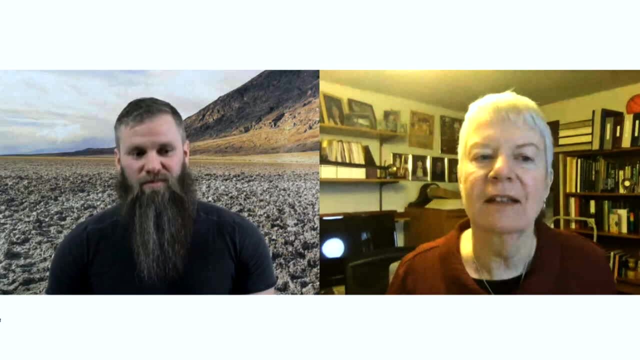 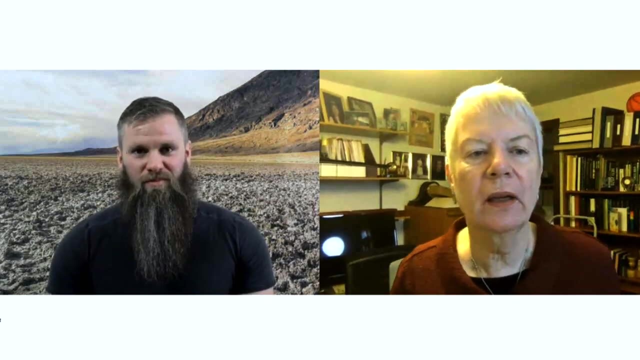 has opened up the field to young scientists of all persuasions and globally right. I think it's great. I think this is just the way we need to go. So, if you'll allow me, to give your audience a homework assignment, Oh please. 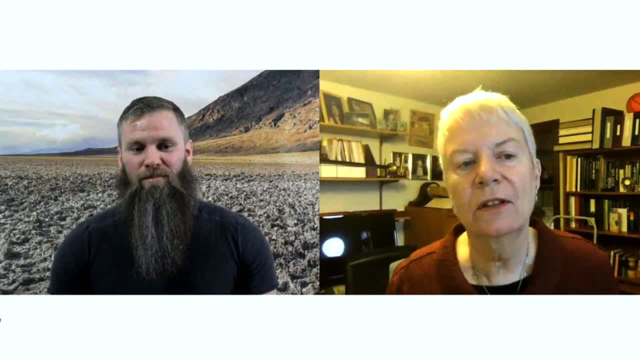 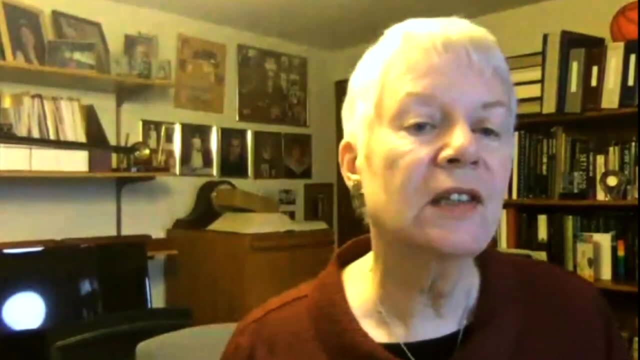 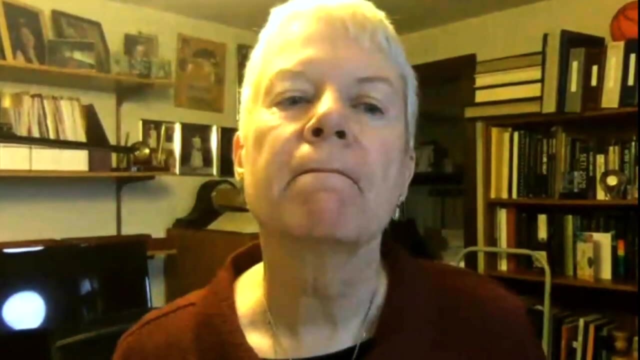 I would like to challenge them to go to all of their social media devices, each of which has a profile, and suggest to them that they might want to say in that profile. the very first thing they say about themselves is that they're an earthling. 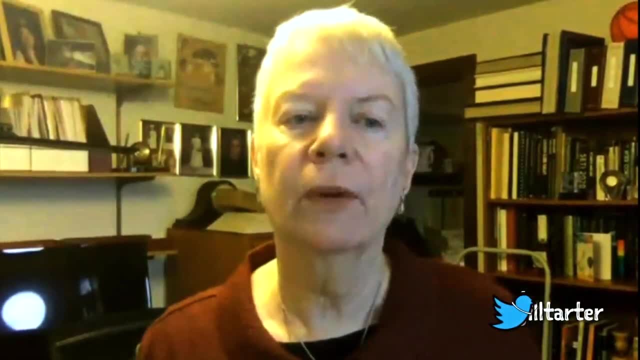 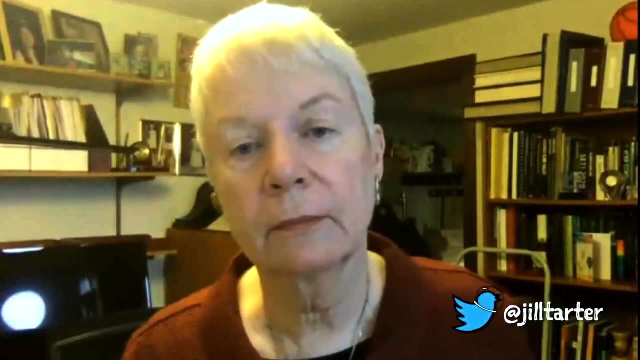 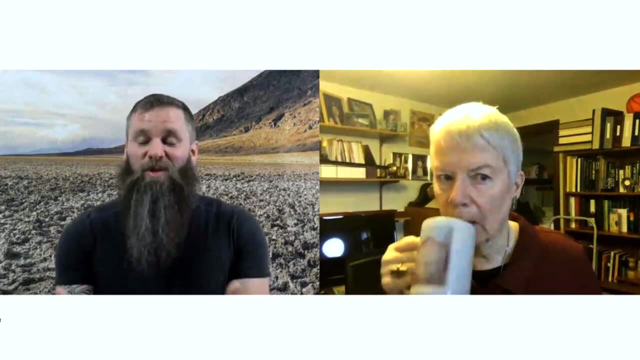 Because I think, ultimately, that's what's going to matter: We're going to find a sustainable future for ourselves and the rest of life on this planet. Yeah, absolutely. It's interesting. you mentioned how we are connecting with all these people And there are so many awesome audience members of our show from around the globe. 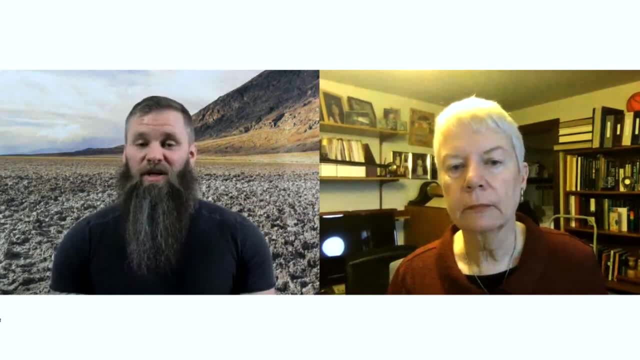 from Turkey and the UK and India and Egypt and other nations who are tuning in, because there are so many young people now across the globe who want to get involved in astrobiology. I speak with young women and young men from various countries, from various backgrounds. 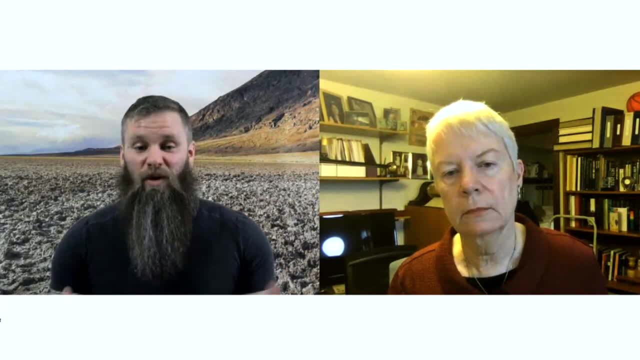 on a weekly basis these days About what they can do to get involved in astrobiology, And so I think so many of us are humbled to see how enthusiastic all these young people are, from all these different backgrounds, about these big questions of: are we alone? 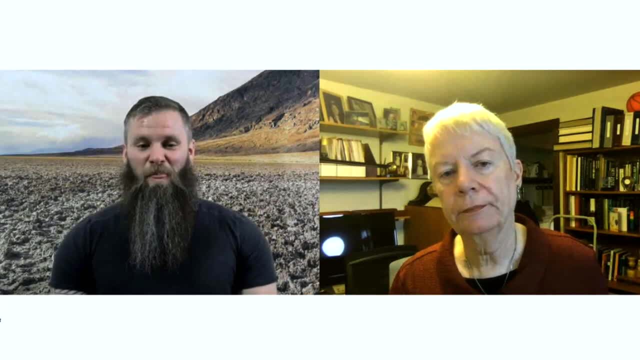 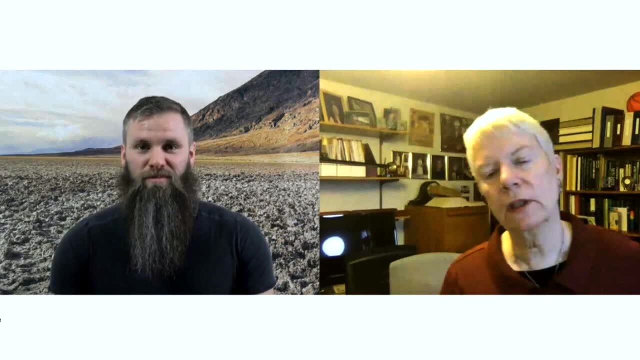 And if not, how do we find out? And I absolutely love that Right And you know, because we're now engaging globally with different cultures and different traditions as well as we're being more inclusive as far as gender Right. 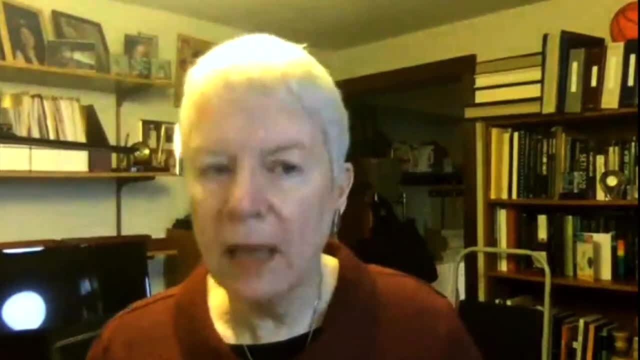 Yeah, Yeah, Yeah, Yeah. And you know, I think for me as a woman, as a person, I think that it's inevitable that we're going to stub our toes Right, That we're going to make mistakes. 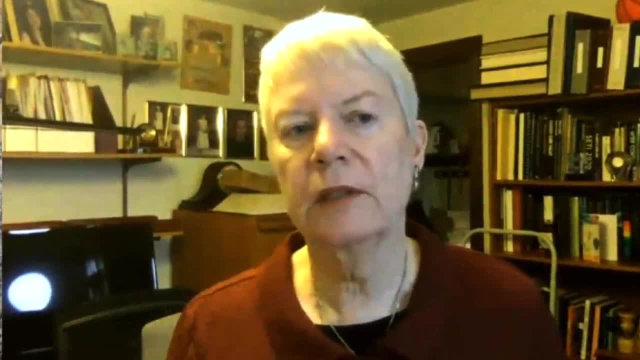 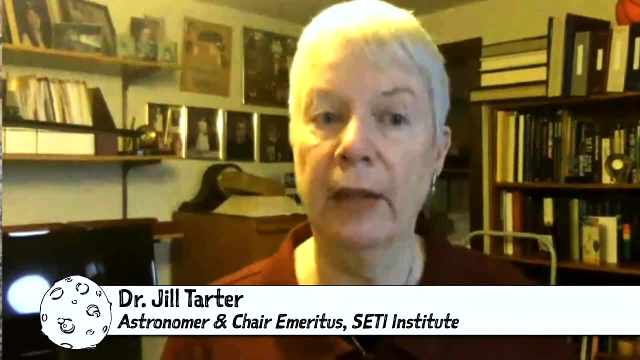 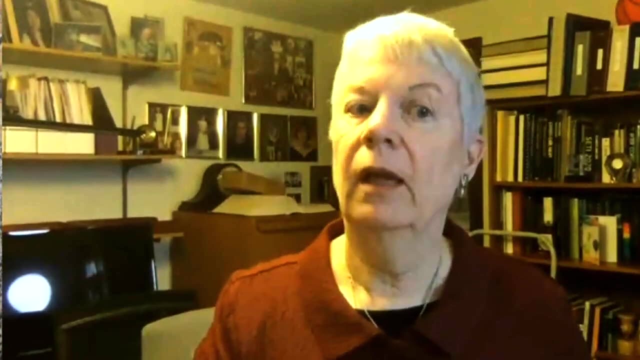 Not intentionally, not with bad will, but just out of ignorance or not understanding, And I think that we all have to be prepared for that and be willing to say, hey, whoops, that wasn't appropriate, And then we all move on and get over it. 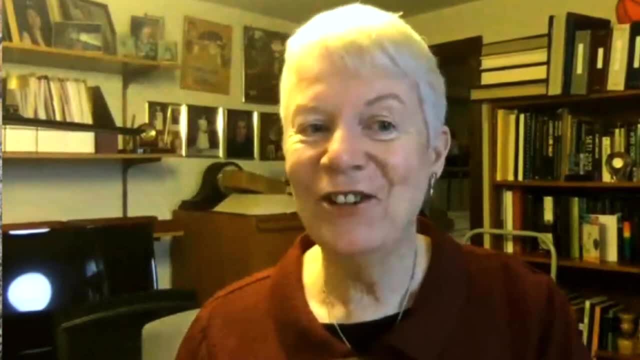 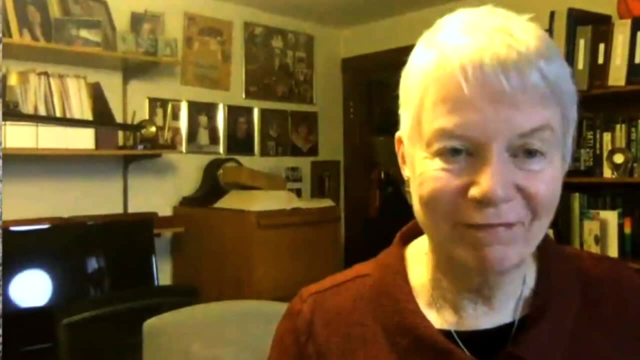 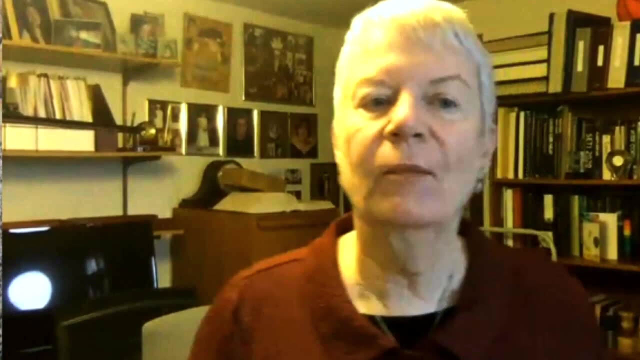 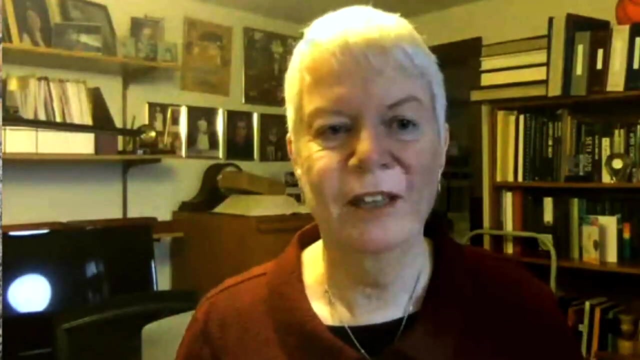 And it's only bad if you don't learn from that and repeat the action. And then we should appropriate controls or reactions. But yeah, people are going to make mistakes. be aware of it, try and move on, But if we repeat, nope. 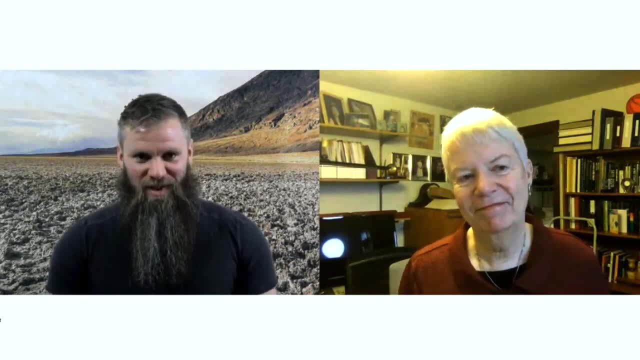 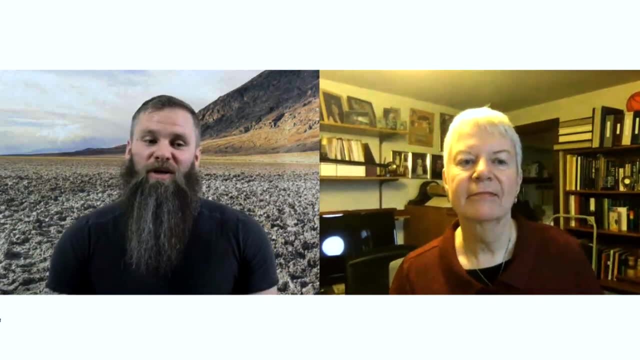 But yeah, so kind of on that idea of us making mistakes, I'm going to bring it back around to science fiction for a moment. Our user, Suraj Kumar Sahu, on SaganNet, wants to know what you think of the film Interstellar. 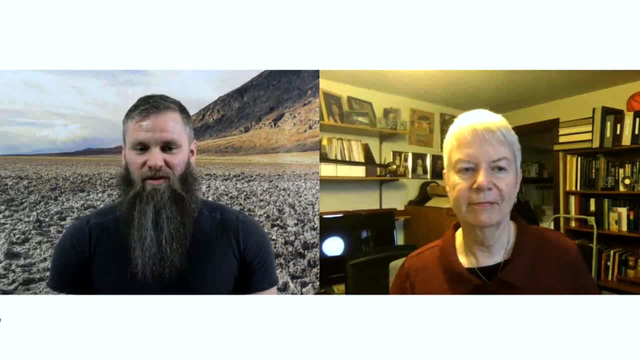 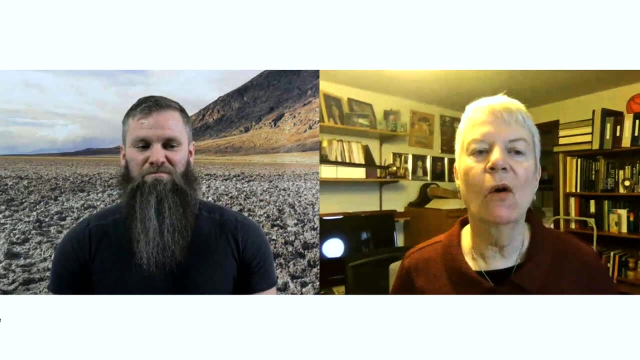 a film where it starts off with the idea that humans have made a very bad mistake, have made Earth's climate so unlivable that they want to go somewhere else to live. What do you think about the story in Interstellar Either? they didn't do their calculations correctly. 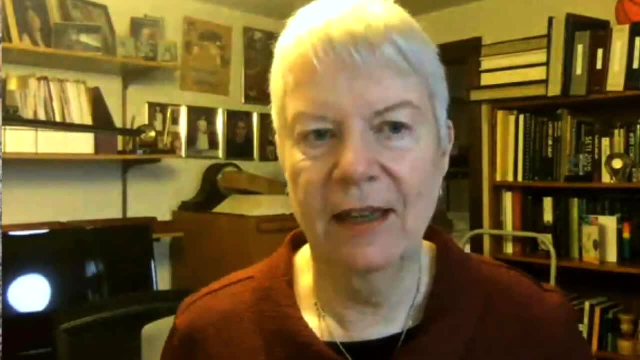 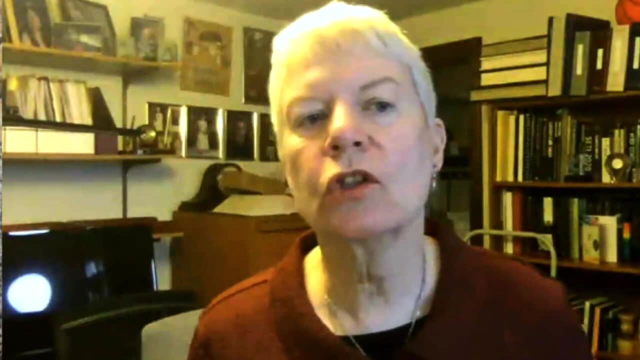 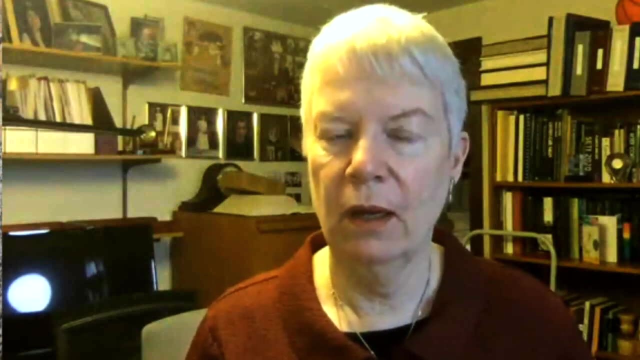 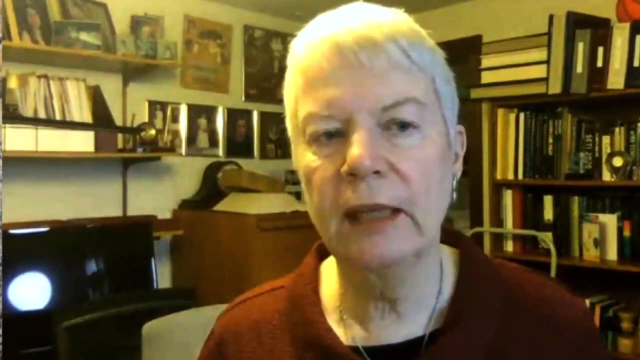 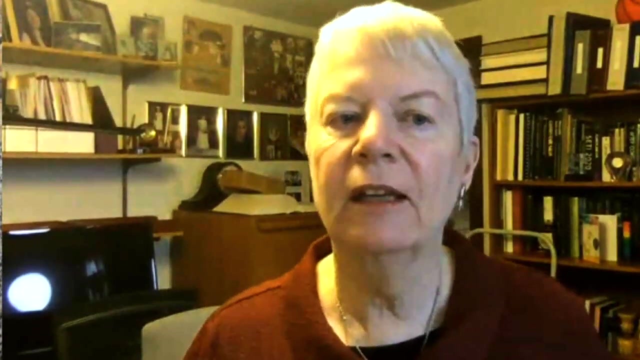 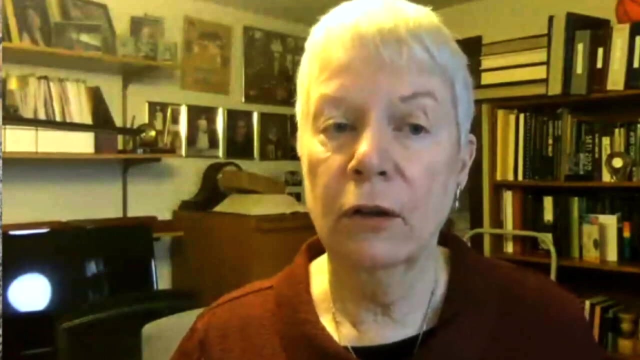 Or that framers of them did not give us enough information to make the case that it was totally unaffordable to fix things at home, Because the cost of taking a population off planet is really horrendously large And I think A lot less money would probably used wisely and in a very targeted fashion, could probably 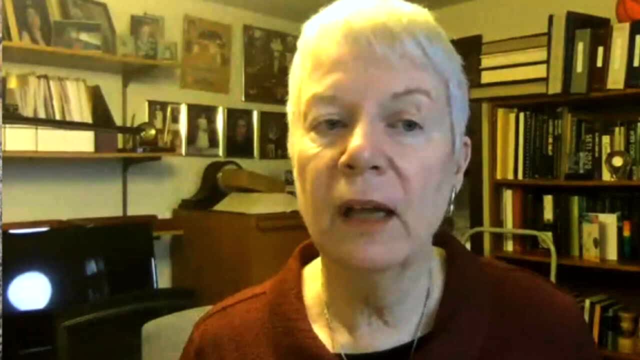 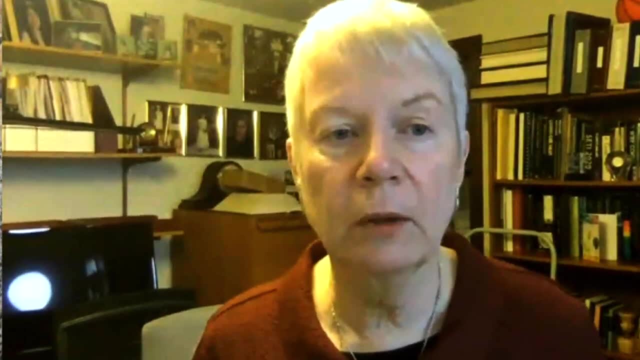 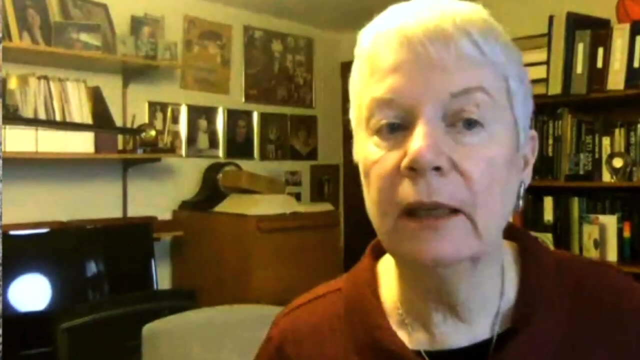 solve the problems at home And bottom line, if you don't solve them, you're just going to get them with you And you're going to be facing the same problem in the future in another location. So I think that I'm really, really excited about exploration. 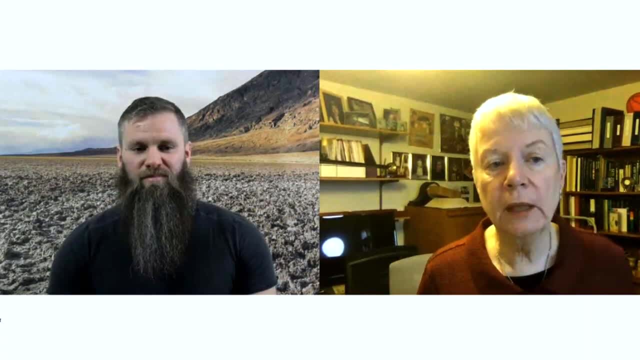 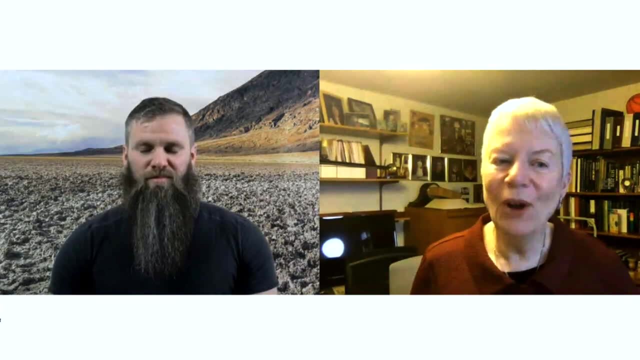 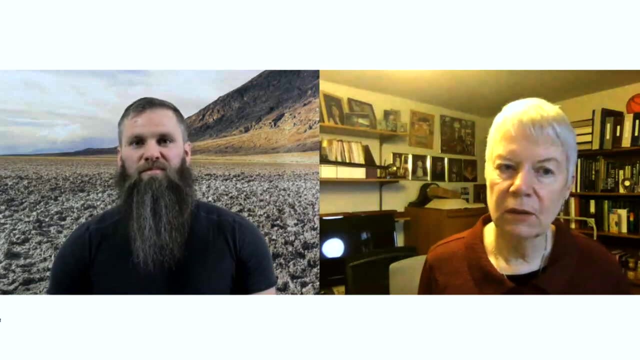 And I think humans will be occupying other bodies in the future. I think it will be all humans, I think it will be the explorers, the scientists, the engineers at the frontiers, And that's good, But hopefully they have a well-shepherded planet to come home to. 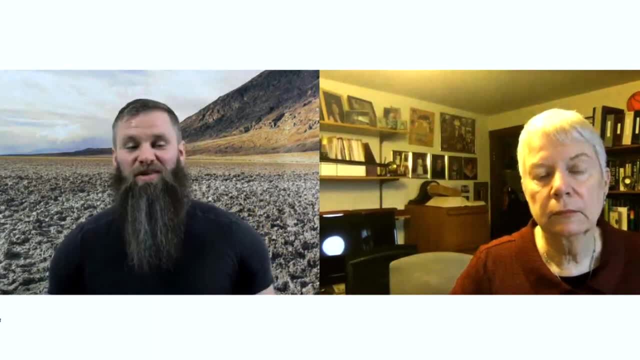 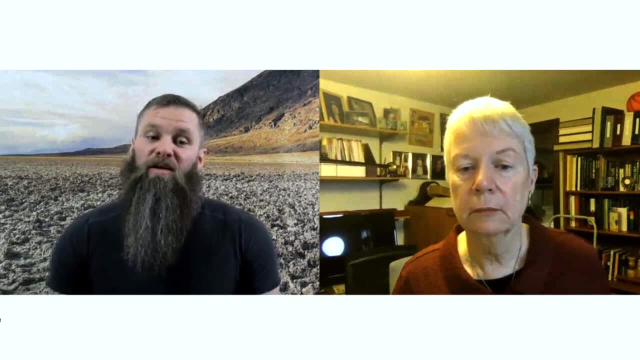 Absolutely Yeah. So the scientists, the engineers will be the next pioneers. basically, Yeah, Yeah. We have another question here from Rami El Sabah, from Seganet. Rami asks: do you think there's another form of life on another planet where the building 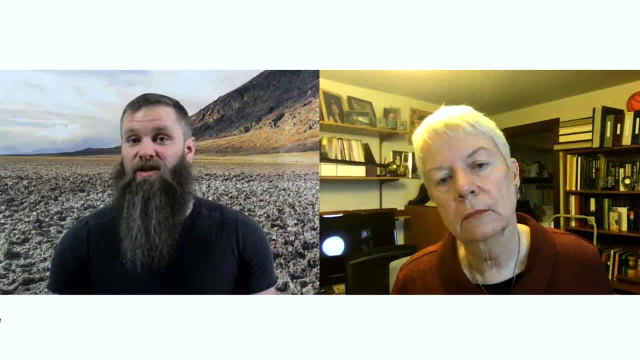 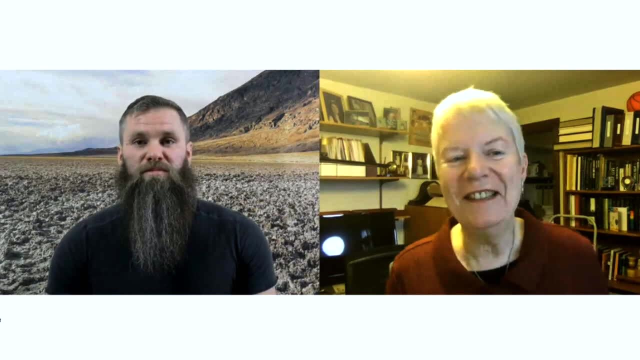 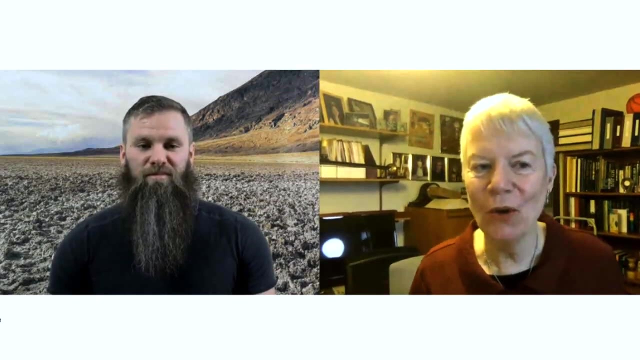 blocks are inorganic matter, So perhaps something like the silicon life that some have talked about. You know, that's really one of these things that's so hard to puzzle. Are we telling ourselves a just-so story when we make the arguments for the greater efficiency? 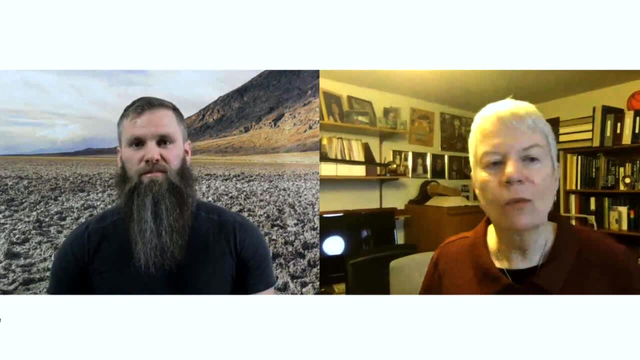 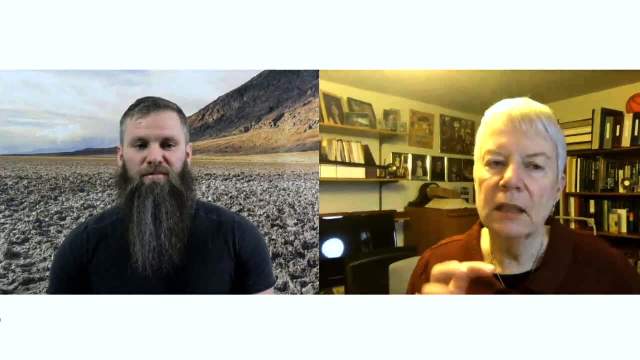 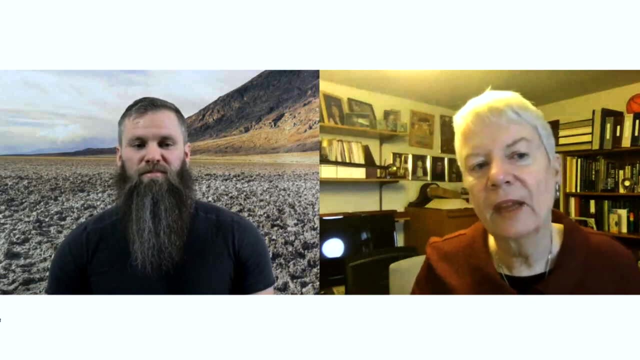 of carbon versus silicon. You know, with one example it's damn near impossible to decide what's necessary and what's contingent. I often think if I had a prehensile tail, which would be a lot of fun, I think I would. 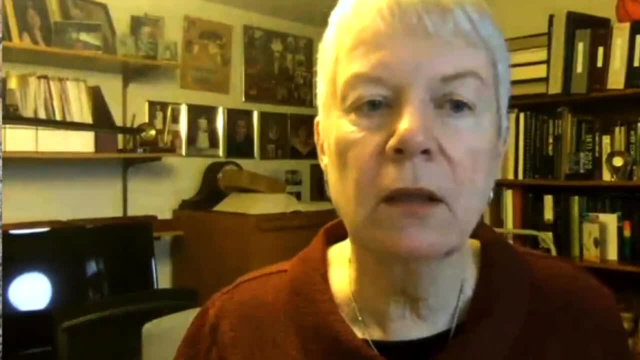 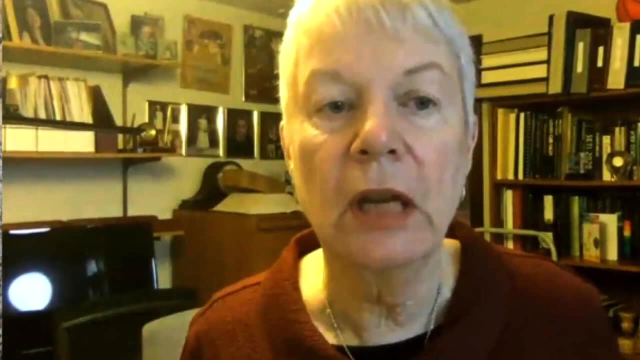 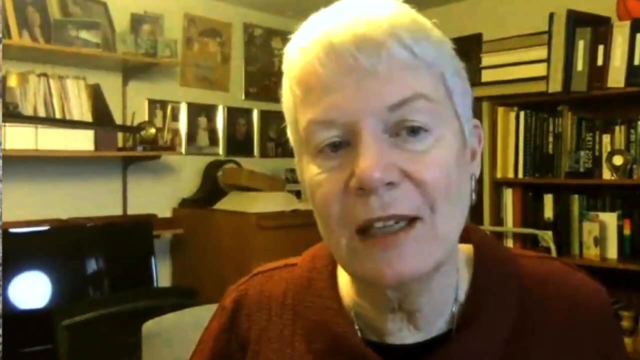 i think i would have a really good story to tell you about why i couldn't be a scientist, why i couldn't be an engineer, why i couldn't try to answer this question if i didn't have that tail. so yeah, there are lots of stories that we can tell and it's based in in the science that we 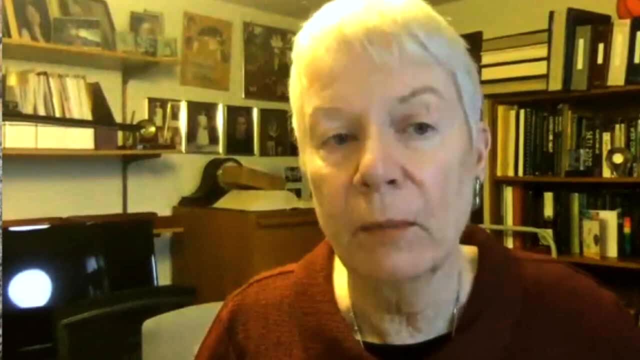 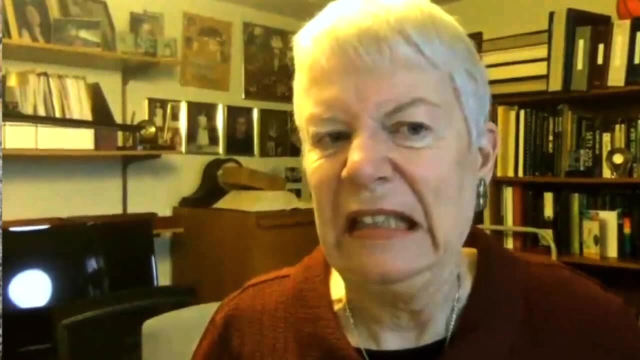 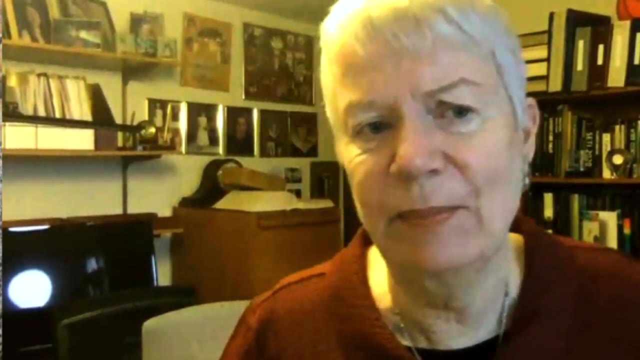 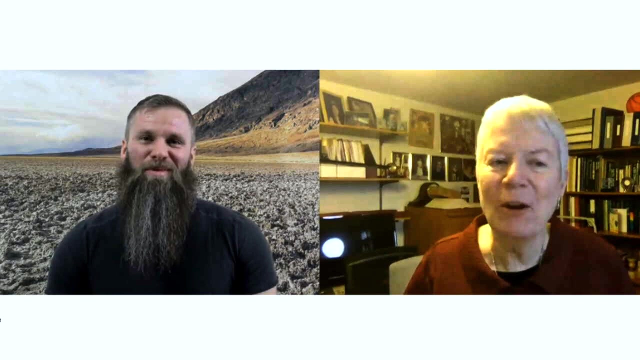 currently understand that says carbon is going to win out over silicon. i mean, if you want to get gross kind of hard to eliminate sand- i just think about the seaside and the sand inside my bathing suit, right? um? so carbon dioxide gas is is a lot easier to deal with than silicon dioxide, um. 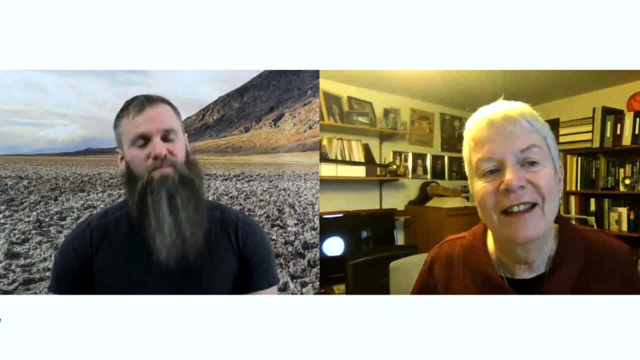 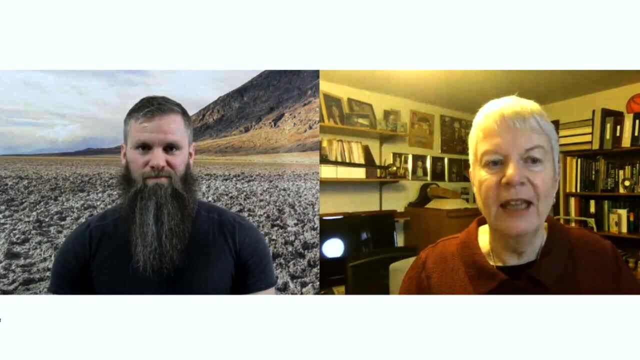 but we just. there's so much we don't know. and with all of these questions, as a physicist, do you want to tell me how to handle the data? here i'm gonna jump in here. i'm gonna do that. okay, here are all the options and let's figure out what the branching ratios are. you know how much, what percentage of? 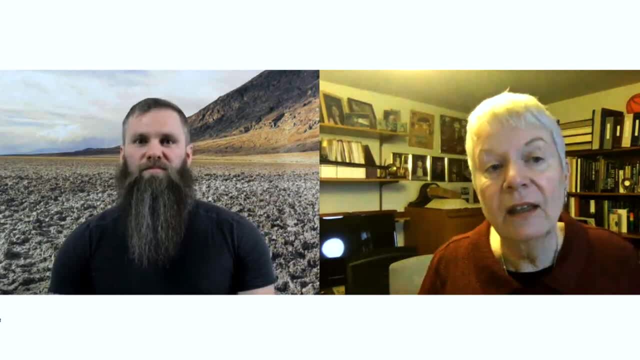 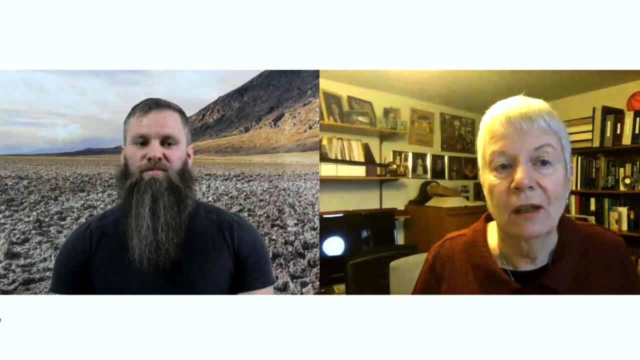 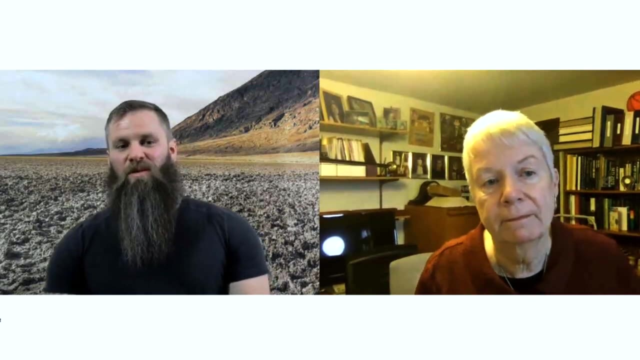 the time did things go in that direction, versus that direction, versus that direction, and then we could begin to make reasonable statements about these kinds of very good questions. at the moment, we've just got an example of one, and we have to see what we can do with that, absolutely, um. so i have one more question, then, here from our audience. 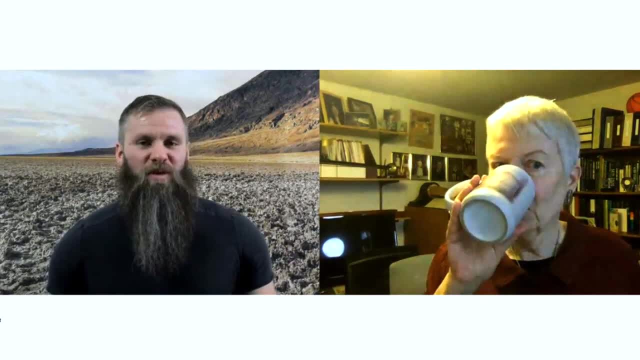 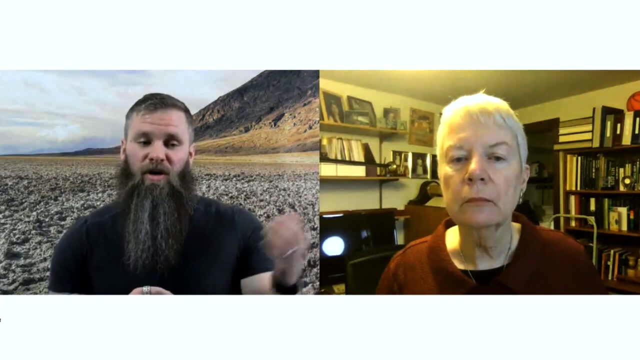 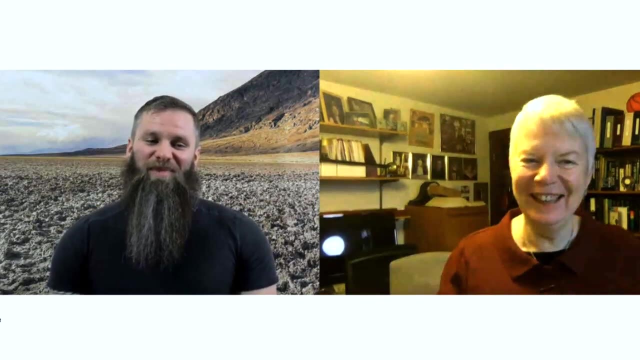 um, and it kind of follows off of that. so, rather than being based in inorganic life, whether or not biological life as we know it here on earth could evolve into a form of inorganic life. so penny boston, on live stream, has asked. she asked: what's your personal opinion as to whether 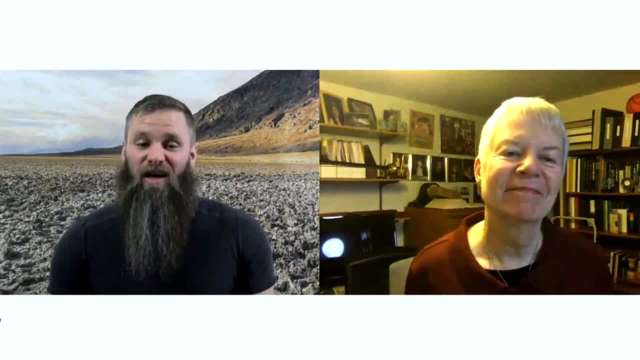 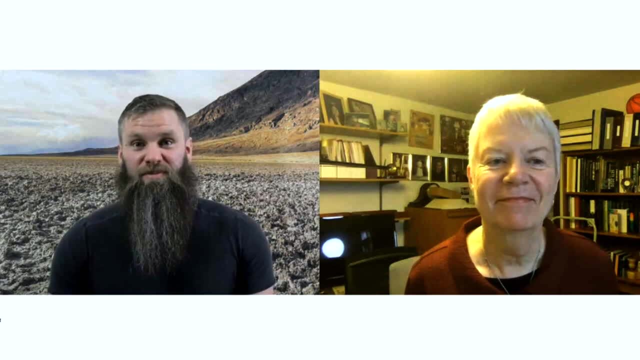 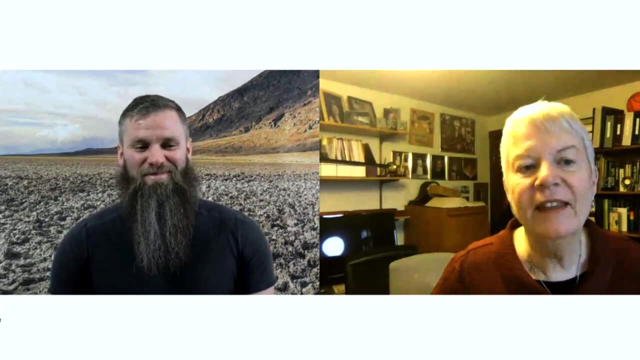 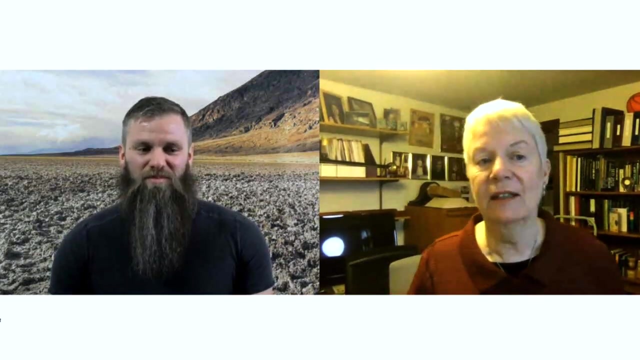 civilizations that we may discover, or that may discover us, are more likely to still be organic life, or that have transitioned to some sort of cyber race. yeah, i think that i think i've seen some of penny's cartoons and i think she's got some very interesting ideas. 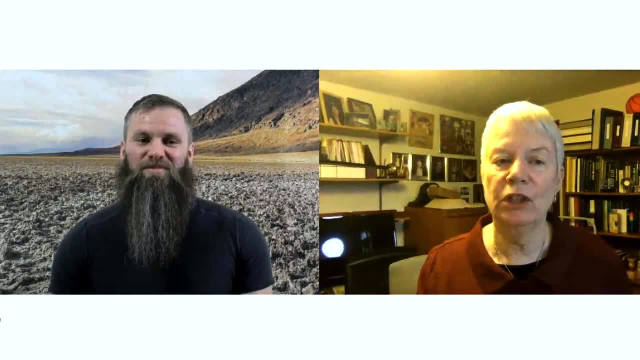 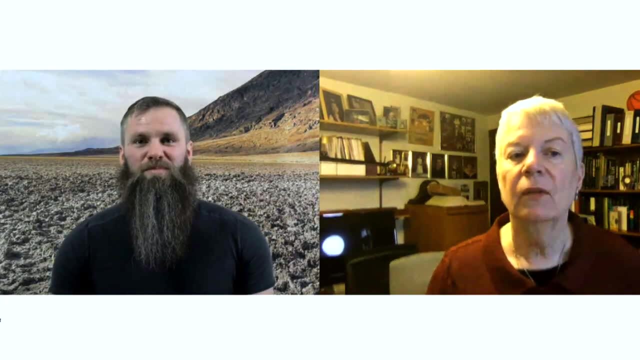 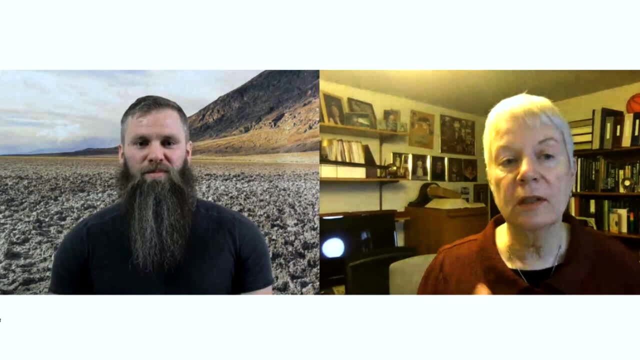 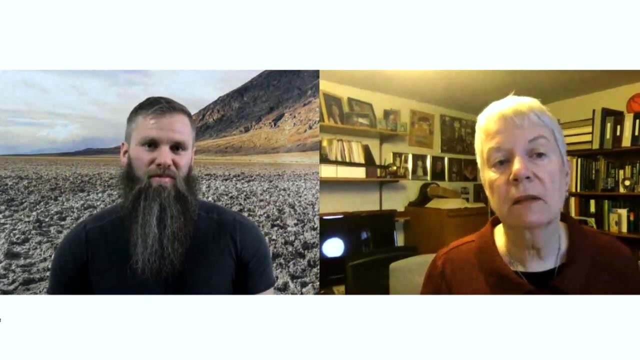 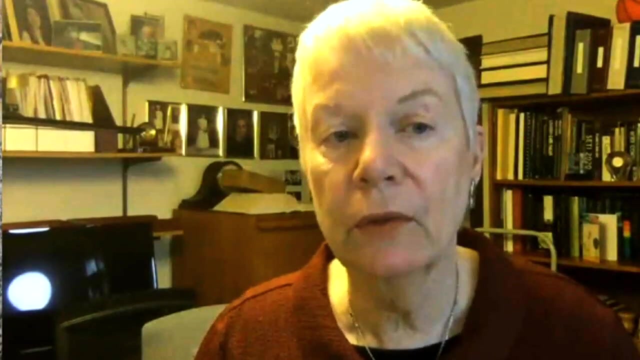 about a future evolution that takes us to be more a cooperative partnership with, um, silicon-based intelligence. i mean some people go the other way and say, once the silicon-based intelligence shows up, we don't really need the biologicals anymore, maybe we'll make good pets. um i i actually think it's going to be a cooperative co-evolution such as we've had. 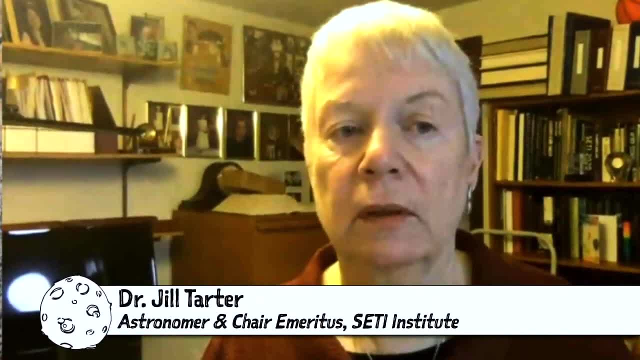 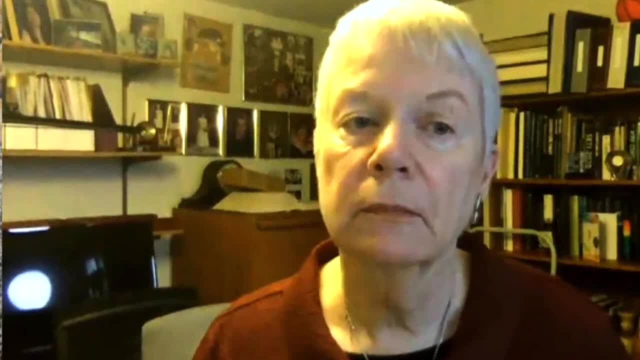 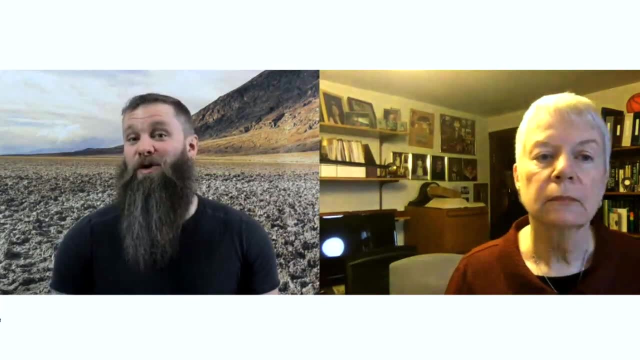 on this planet for billions of years and we, ultimately, we probably will not be the smartest kid on the board. interesting, so the future might not just be just us, but us sharing our world and our future with with another thing. i like that. well, that's all the time that we had. 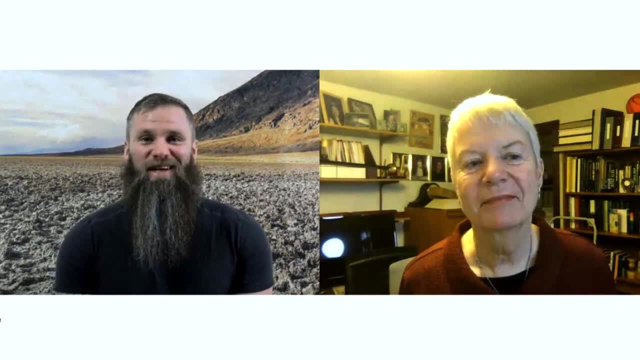 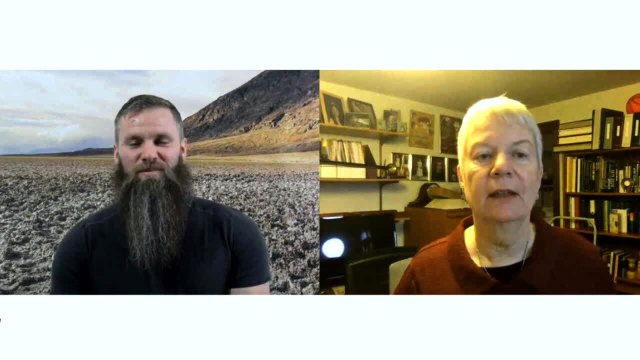 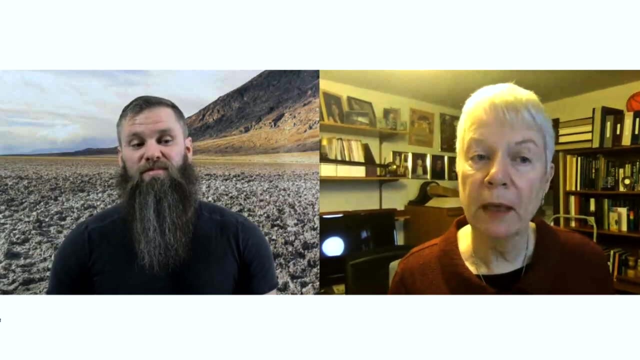 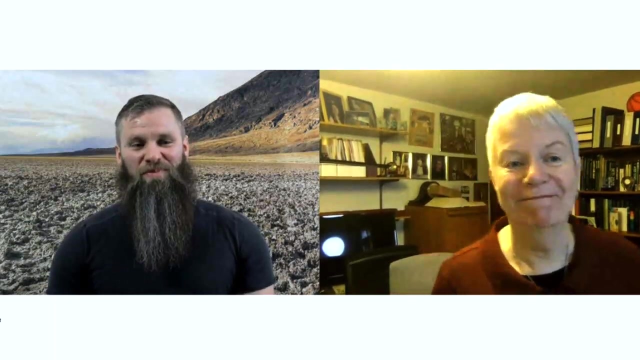 for today's episode. uh, jill, thank you so much for joining us for ask an astrobiologist. oh, it's been my pleasure and i'm sorry. we've had these hiccups and technological freezes, and caleb reminds us that on a finite world, a cosmic perspective is a necessity and not a luxury. so it's beautiful, caleb. i think we'll leave.